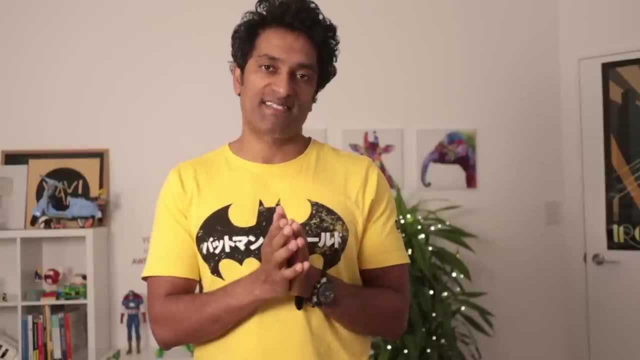 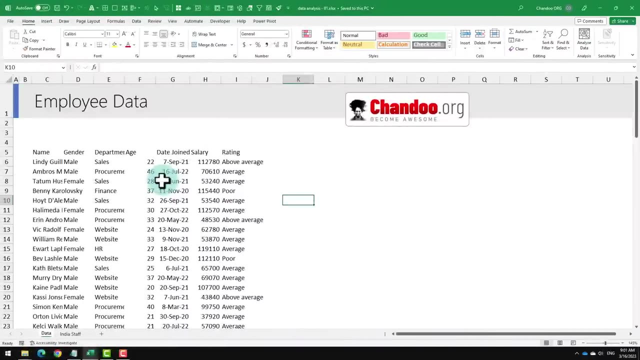 so that you understand and implement them for your success. Let's go. How to use Excel to solve problems in Excel. This is the sample data file that we will be using in this video. Here, as you can see, we have two kinds of data. One is the data and another is India staff. 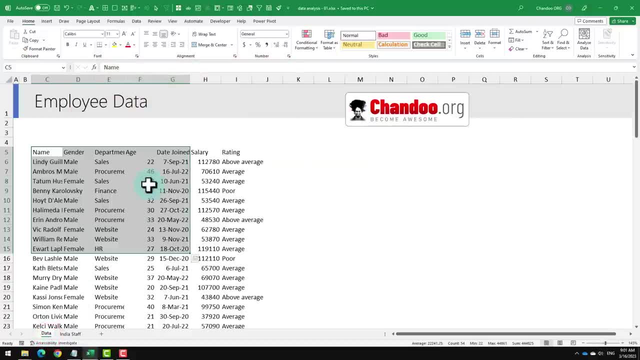 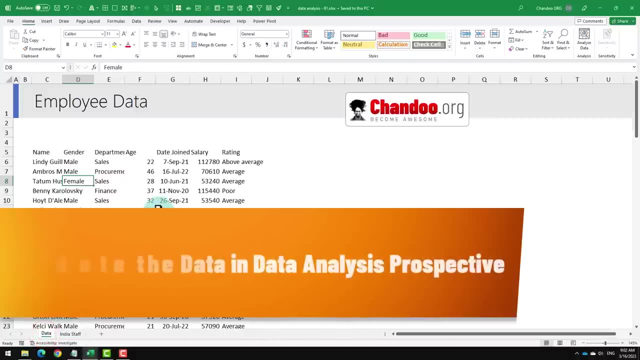 Awesome Chocolates primarily operates out of Wellington, New Zealand, But we also have a branch in India and the data is split into two tabs: one for our Wellington staff and this is our India staff data. So our first task is to take all of this data, consolidate it, clean it and make sure that it is 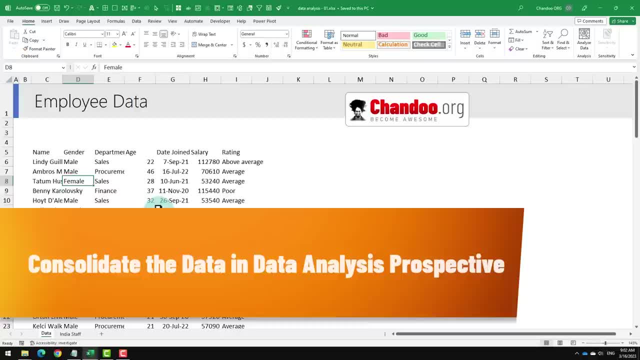 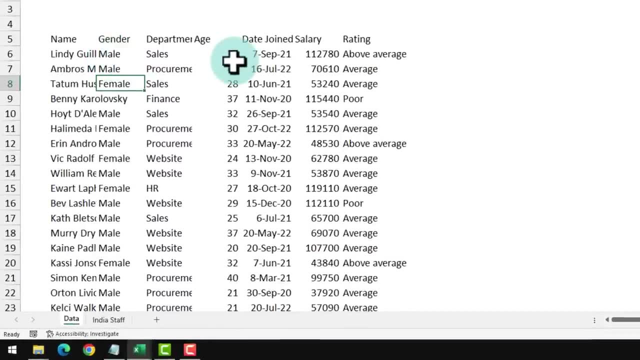 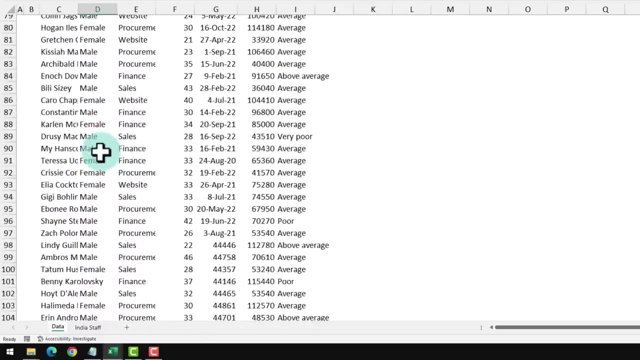 in the ready to use form from a data analysis perspective. Whenever you have data like this, it is a big challenge to understand and use the data if the data is not properly maintained Here, as you can see, there is a lot of information. 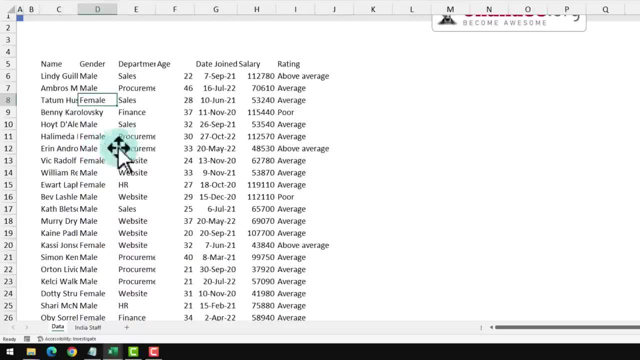 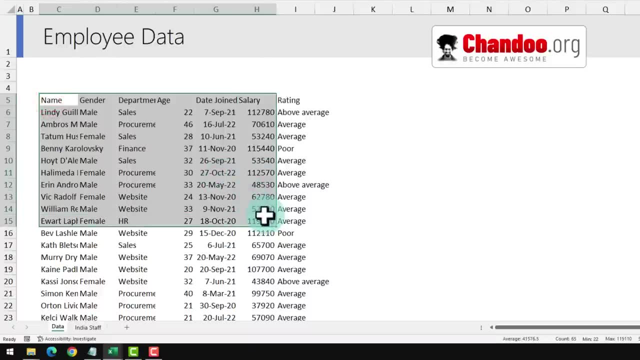 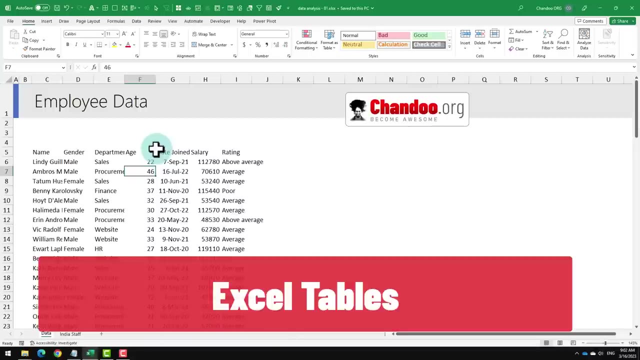 and we are not even sure if there are any duplicates, missing elements or anything else in the data. so what we will do is first take each of these data sets and then turn it into a usable format. this is where excel tables come into picture, usually anytime you are analyzing business data. 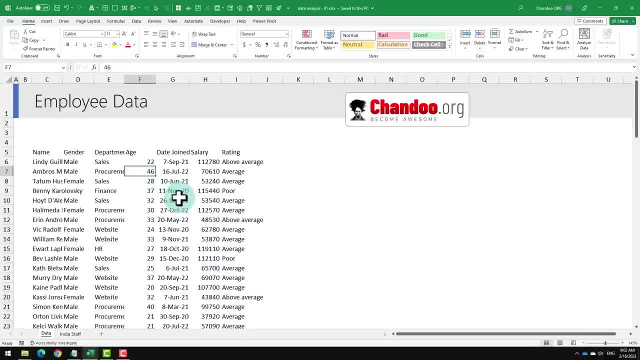 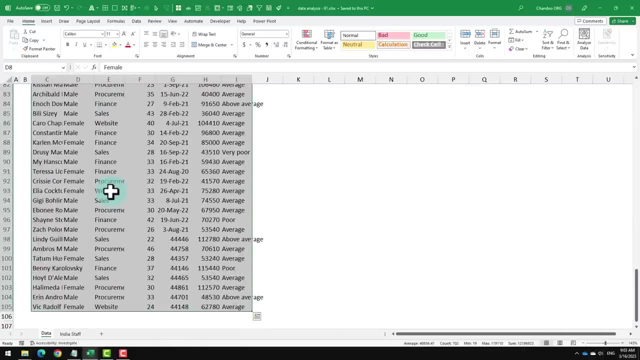 the data always tends to be in a tabular format, so all you have to do is either select your entire data, and this is where you can use the shortcut ctrl a, you must select one of the cells in the data and press ctrl a, and excel will select the entire range where your data sits together. 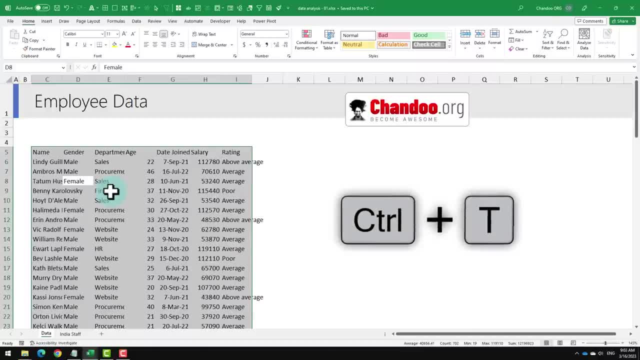 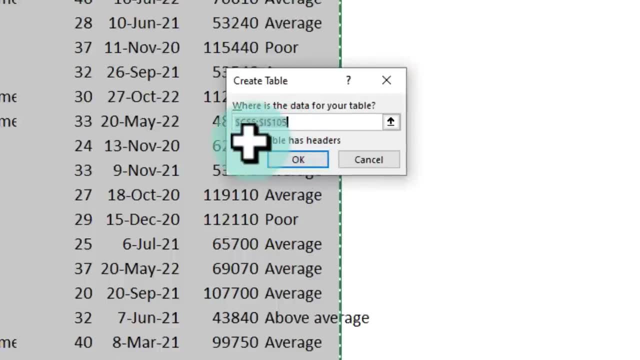 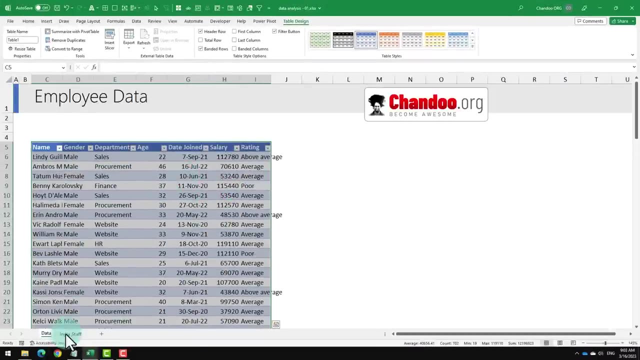 and then press ctrl t- t for table. this will prompt you- how do you want your table and whether you have a header row. in our case, we do have a header row, so i'm going to check that and click ok, and now we have a table here. let's do the same for india staff. ctrl a, ctrl t. 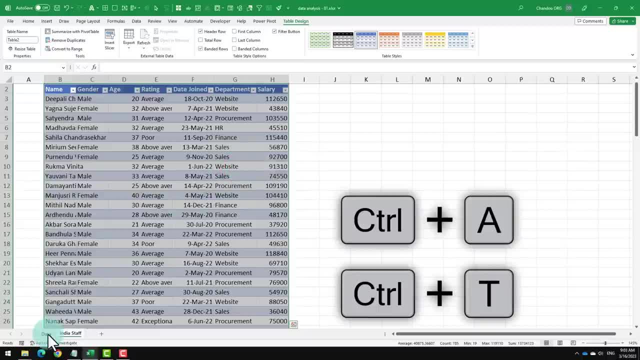 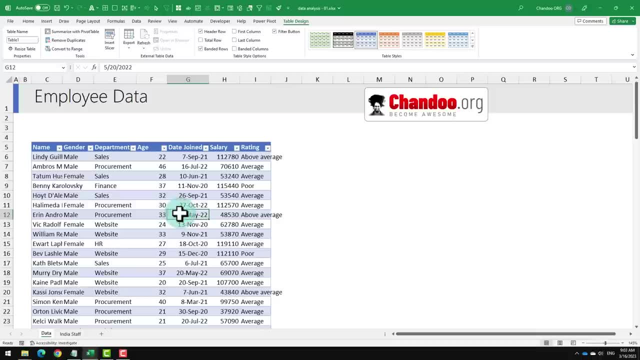 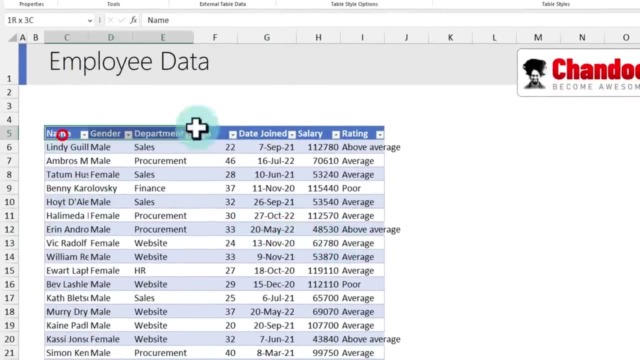 so now we do have both data sets formatted in the tabular format. what tables make is they quickly apply some simple formatting on your data, give some borders and highlights and everything. they also add this header row in a different color and set up filters for you so you can quickly eyeball. 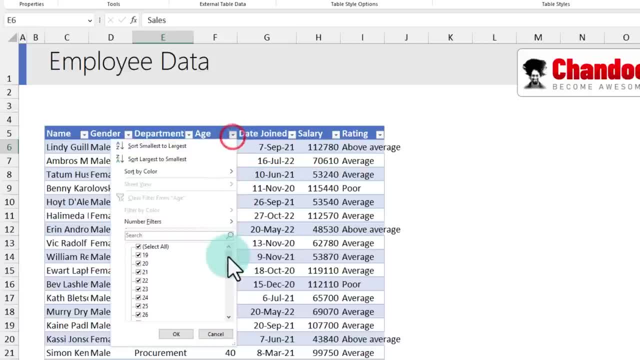 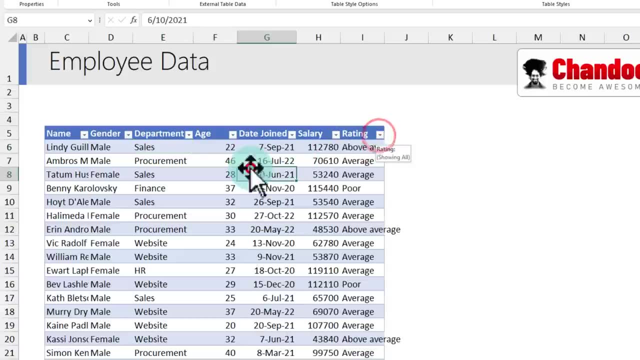 and see what departments we have, what is the age range of our employees, from 19 all the way up to 46, or what sort of rating are there? let's see this entire data in one view. clearly you can see that, for example, the name column doesn't show the full name. likewise, the rating kind of spills outside. one quick trick. 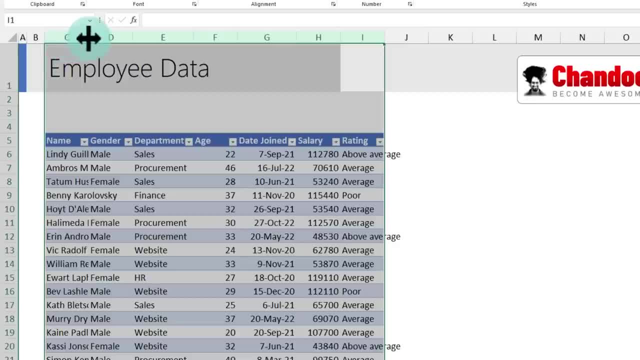 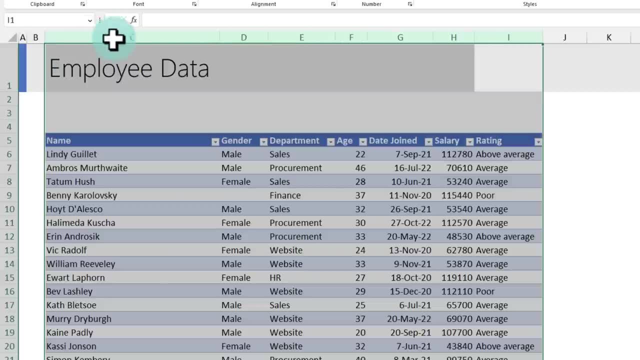 that you can apply here is: you can select all of these columns, place your mouse pointer somewhere in the middle of the columns and double click, and that will resize all the columns. now, what happened in the case of c is because my header here is quite long, this column c also became 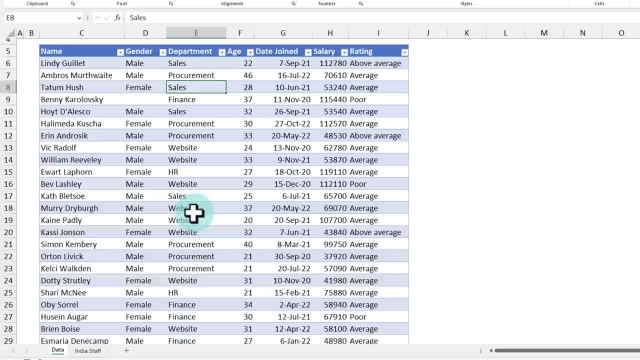 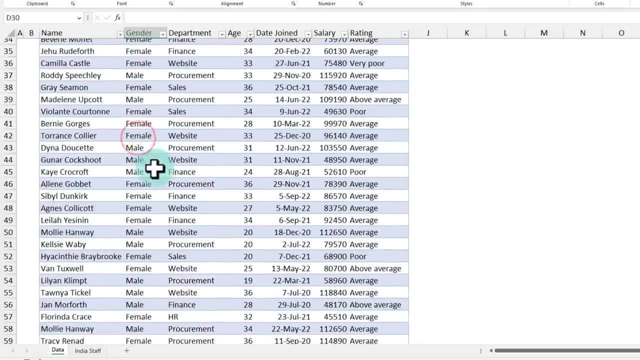 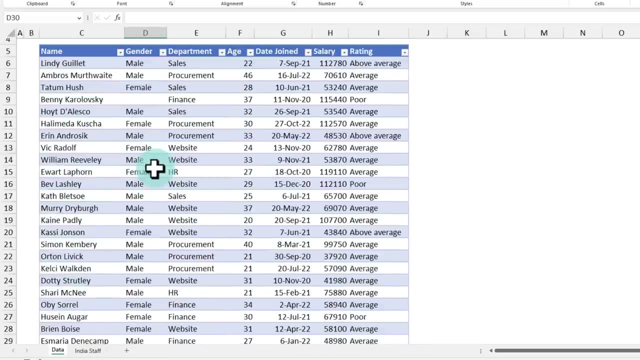 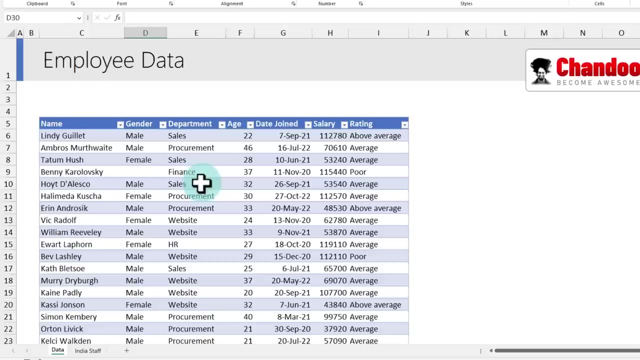 too big. as i adjust this, i can quickly see some problems with our data. for example, some employees do not have any gender information. likewise, there might be other issues that are harder to spot, but they are still there. let's do the same for our india staff, and now we do have two parts of the puzzle. our new zealand data is here in the data table. this will be. 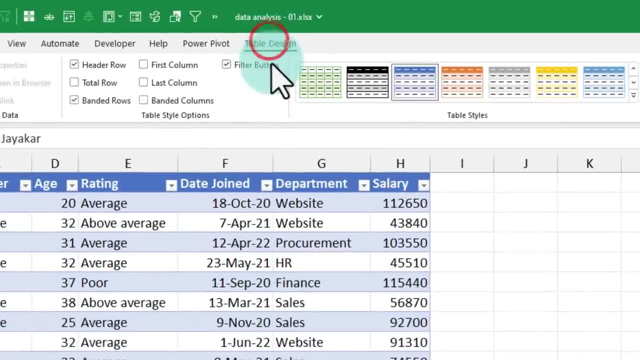 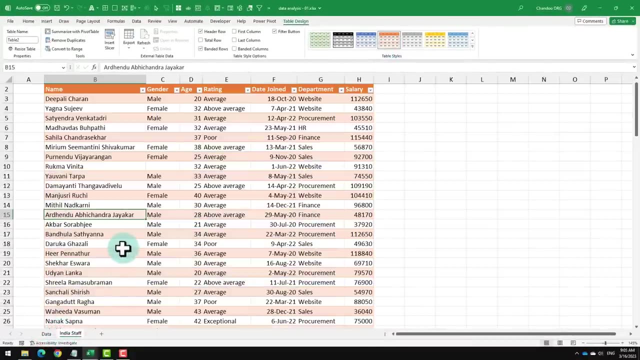 in the blue color our india data. i'm going to change the color of this. for this you can go to the table design ribbon and let's just go with the this orange color for india data so it's easy for us to tell them a part: blue is new zealand, orange is india, but this kind. 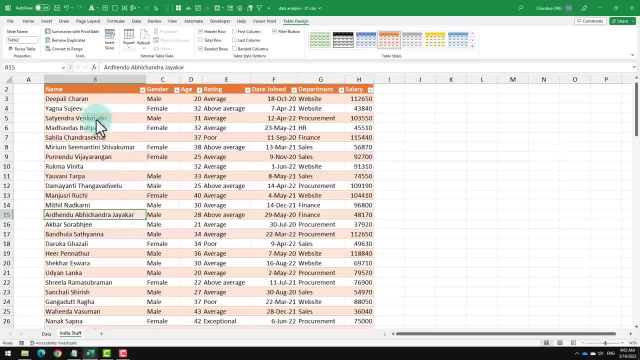 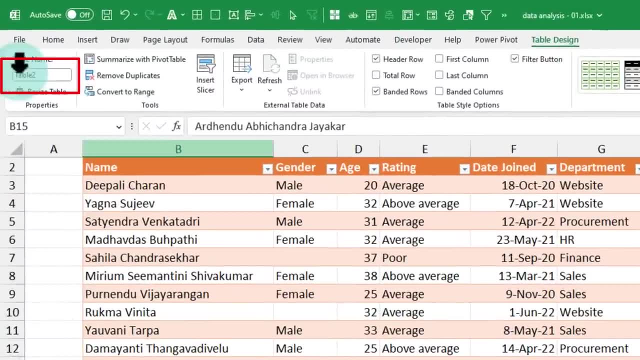 of telling apart is too tricky. so this is where a table name comes into picture. if you go to the table design ribbon, you'll see that the tables have a name option. right now, the india table is table two. i'm gonna call this as india underscore staff. 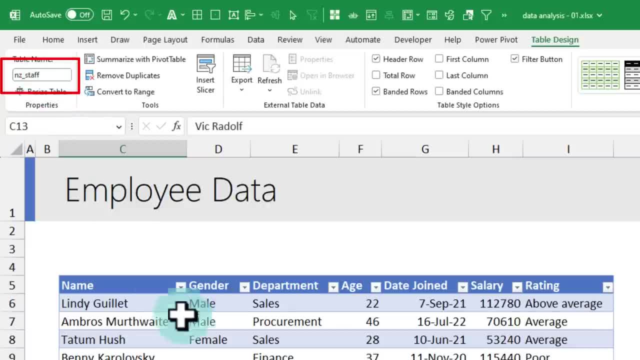 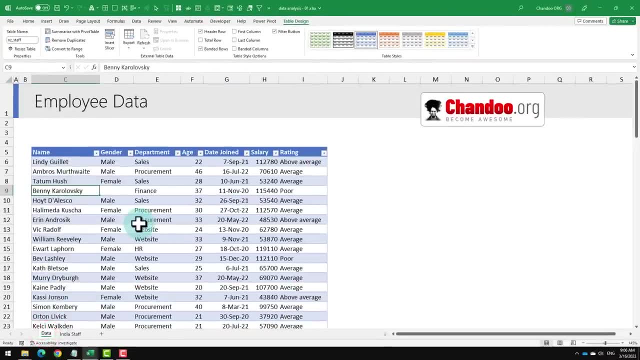 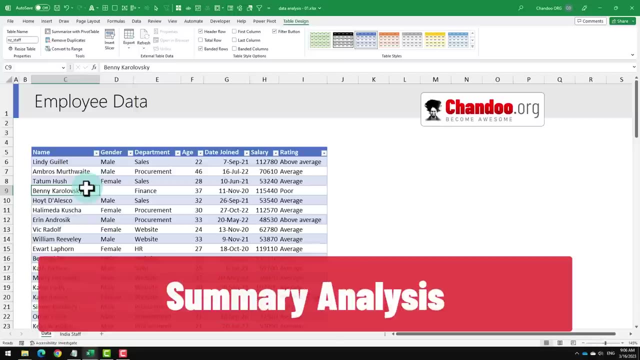 and then this one would be nz underscore staff. so now i have two tables- new zealand staff and india staff- neatly arranged. let's just say you don't want to combine the data. you just want to keep the data as it is in separate tables. but you would like to do some quick summary analysis of the data. 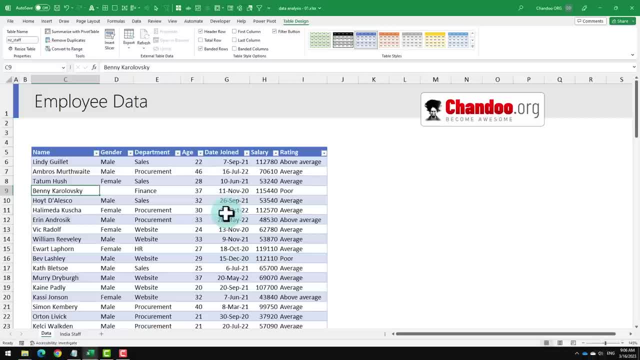 like, for example, you want to know how many employees are there or what is the average salary, etc. what you could do with tables is, when you have a table, you can select any cell in the table, go to the table design ribbon and, from here, enable the total row option. 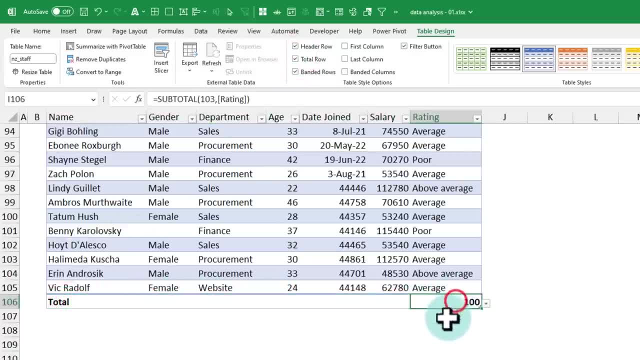 this will add a total row at the very bottom and here it tells me we have 100 people in the new zealand data. this in itself looks suspicious to me because i don't think we have that many people in New Zealand, but we will investigate that a little later. Let's say I 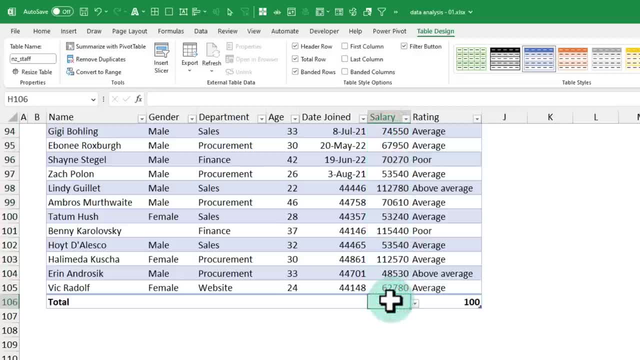 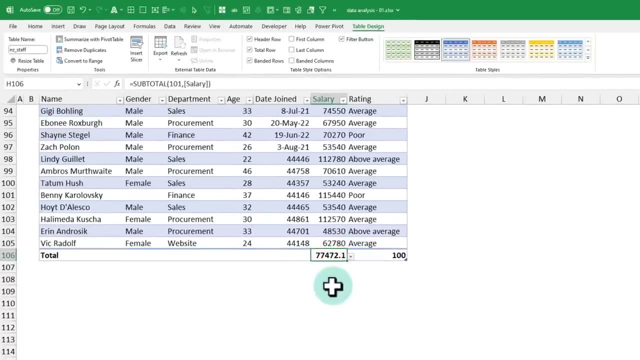 want to see what the average salary is, so I can go to here. it will show me a little bit of drop down next to it and I can pick the average option from there. so the average salary in New Zealand is $77472.. Now it would be good if this is formatted in dollars, so I'm gonna select this entire column. 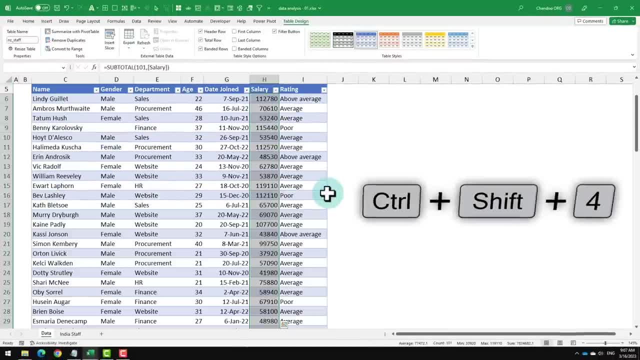 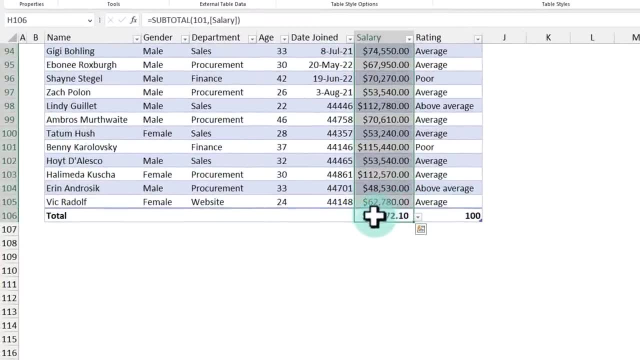 and then press the shortcut ctrl shift 4 or ctrl- dollar symbol. this is gonna apply dollar formatting with two decimal places so that it's easy to read. and then for age again I can do an average. New Zealand average age is 30.52 for date. joint kind of things you don't want to do- averages. 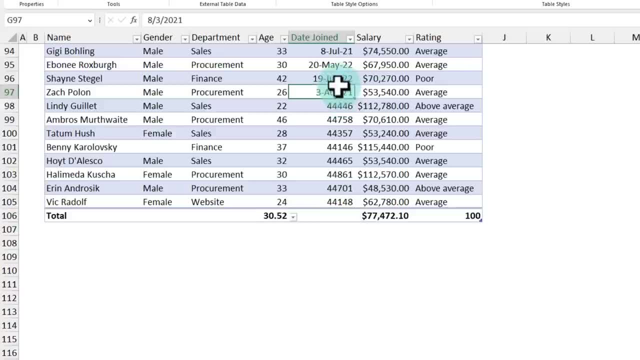 or anything, because it doesn't make any sense. some of these dates look all right. the other dates are looking in number four. This is because, by default, excel stores data for dates in the number format. so if you don't apply date formatting, it defaults to this kind of four, four, four, four six. 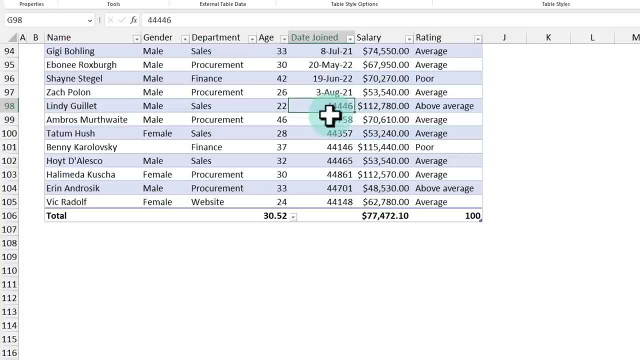 what it means is: this date is actually forty four thousand four hundred and forty six days since the start of excel calendar. excel calendar begins on first of january 1900, so every day is one number, and this is the number of the day how many days that date is. we don't really care for this kind of a thing, so I'm going to select. 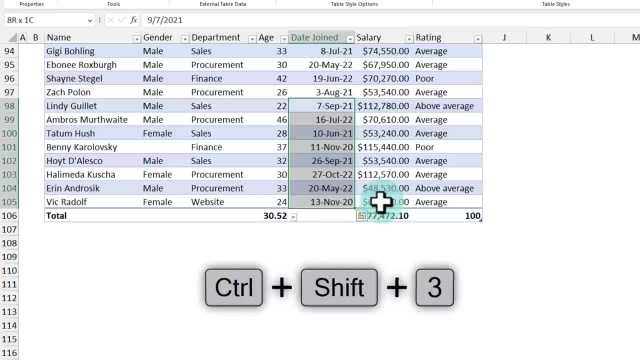 all of these again and then press ctrl shift 3 to turn the date formatting correctly. so these two shortcuts- ctrl shift 4 for currency, ctrl shift 3 for dates- are really simple to remember and very handy to press and they quickly change the formatting for you. 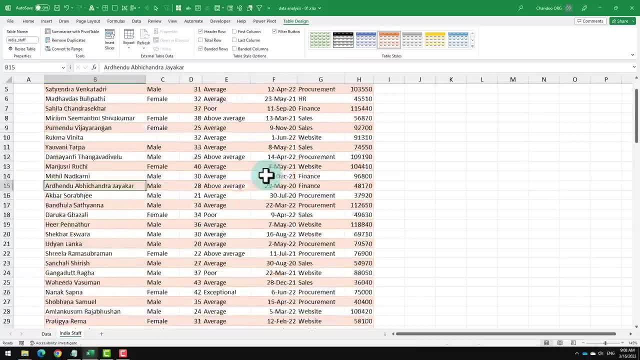 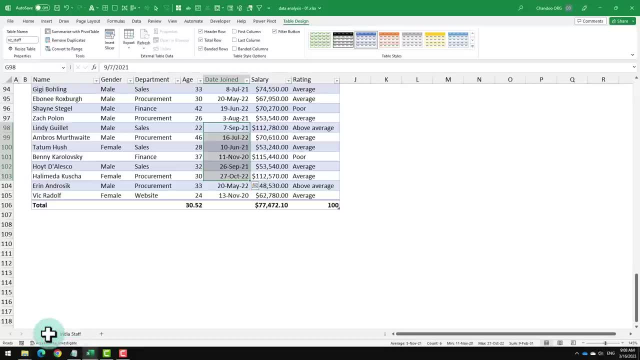 Using that total row we can add quick analysis of our information to the tables, but that sort of a thing is quite useless and also if the data itself is not clean, then these numbers will be wrong. so let's do some quick checks here. I want to see if there is any duplications of the names. if I use the filter here, I will not. 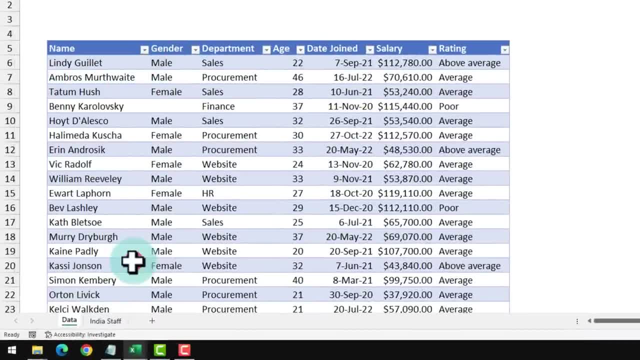 be able to tell apart if a name has repeated or not. so this is where we can select an entire column. to select an entire column in the table, you can place your cursor on the header and when it turns into that black color down arrow symbol, click and it will pick the 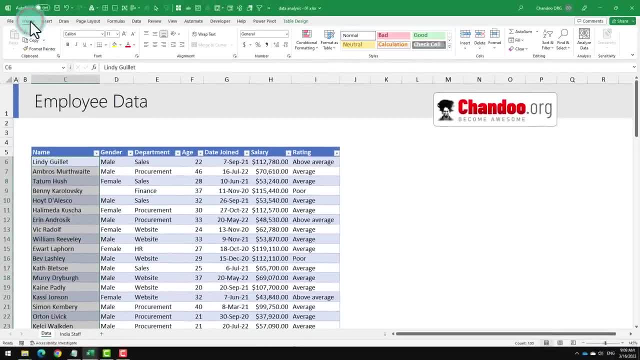 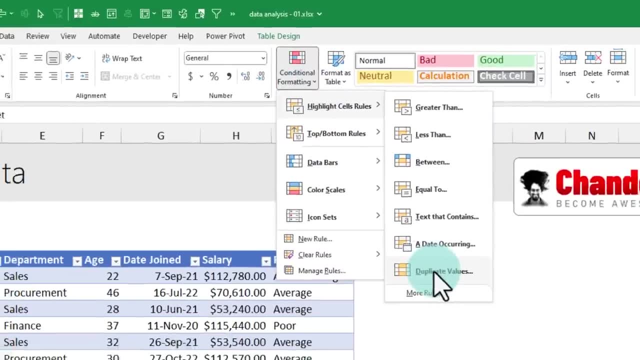 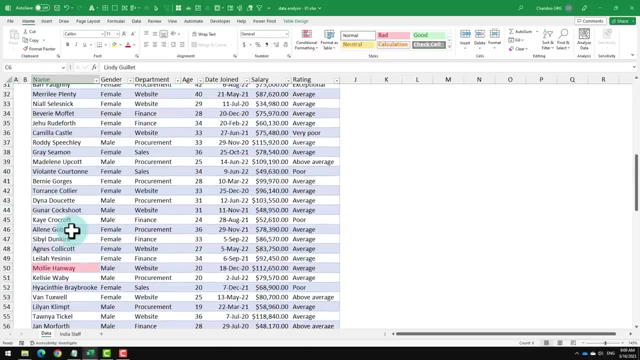 entire column. now you can go to home. ribbon click on conditional formatting. highlight duplicate values. this is a great way to check if there are any duplicates and when you click ok you can see that all of these guys have actually appeared many times in the data, like molly hanway. 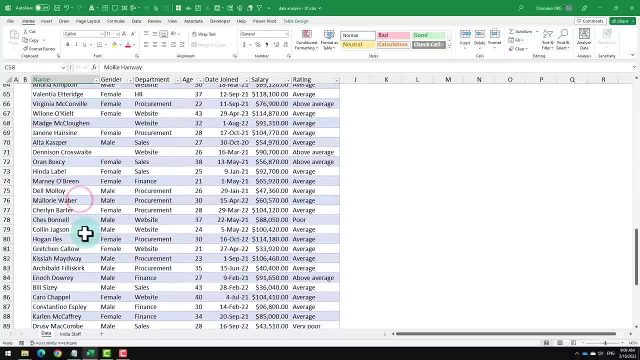 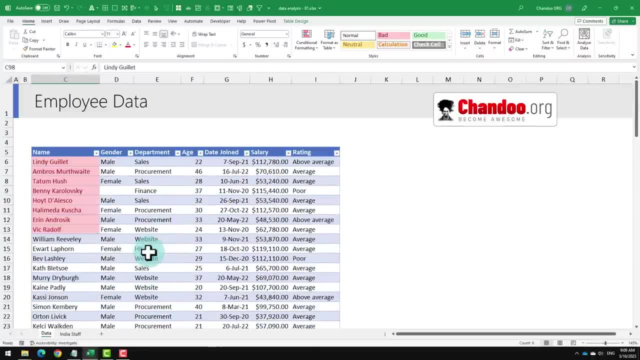 probably appeared somewhere else further down. Yeah, here, and then all of these as well, so looks like someone, when they are preparing this data copy, pasted the information and that created a problem. one way to fix this problem is you can highlight one set of the duplicates, so we do still want to keep one of these rows. 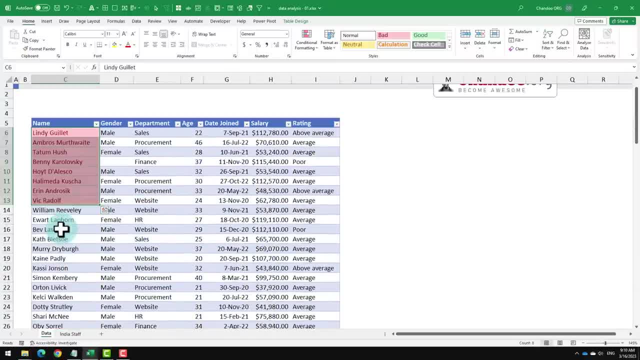 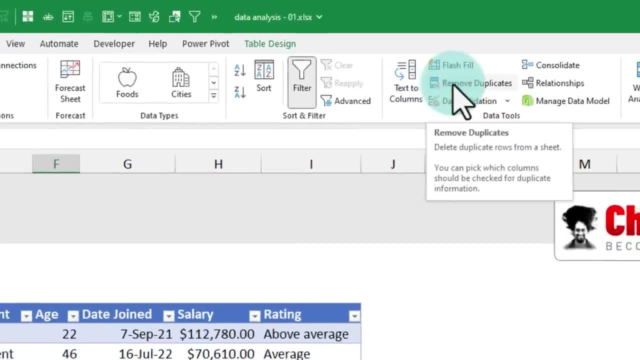 but the second occurrence we can delete it. this kind of a thing can be done manually using the data ribbon remove duplicates button. I'm not going to use this because we need to solve this problem not only for the new zealand data, but also for the india data. 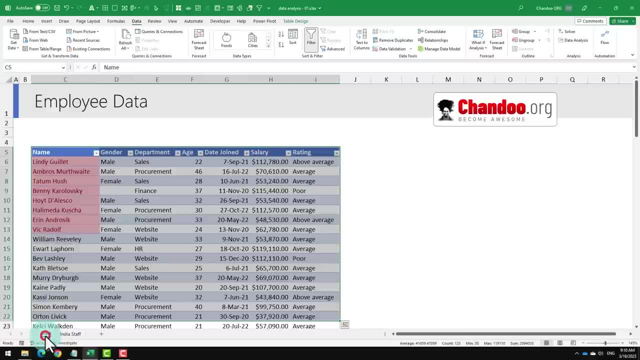 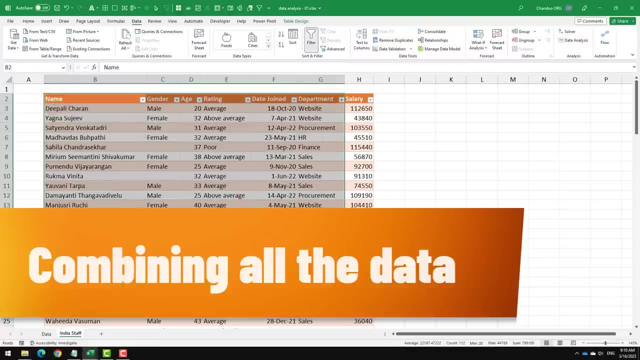 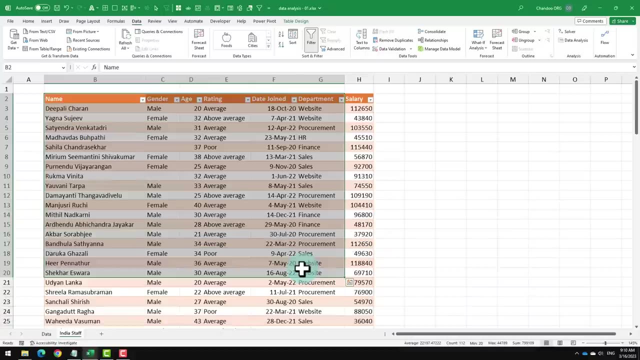 plus, there are other problems that we would like to fix as well. for our next step, we are going to take the new zealand data and india data and then combine everything into one consolidated table, and then that is the table that we will use to do all our data analysis. 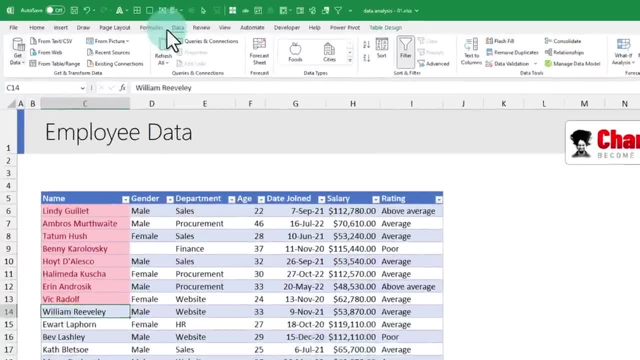 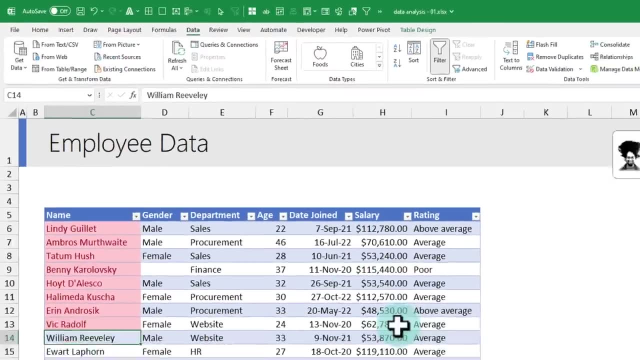 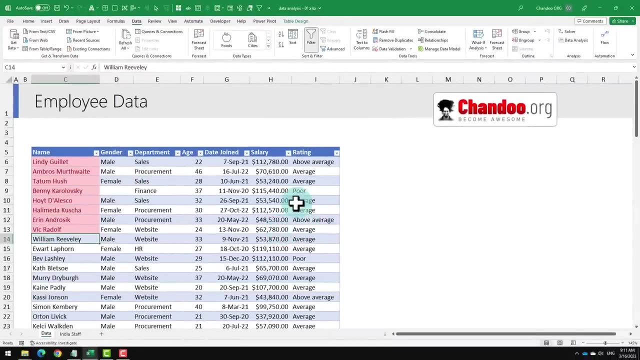 to do this kind of a thing, we are going to use the data ribbon get and transform data area. this is what normally we refer to as power query. a quick note here I'm using excel 365 for this particular video. if you are using an older version of excel, you can still use tables, power query and many of the other. 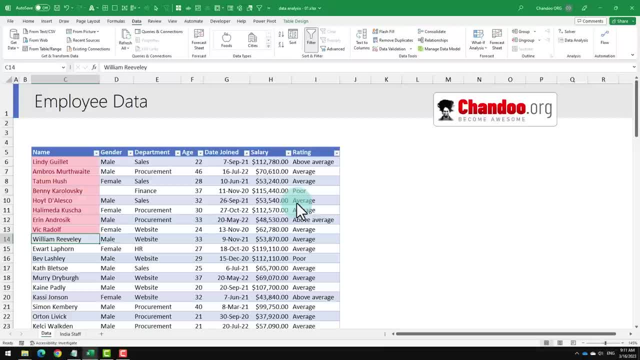 things that I will be showing, but they might be called different or they might appear on different parts of the screen. so refer to the help on the web or somewhere if you get stuck, or post a comment so that I can help you out where to find these things. so, now that we have data, 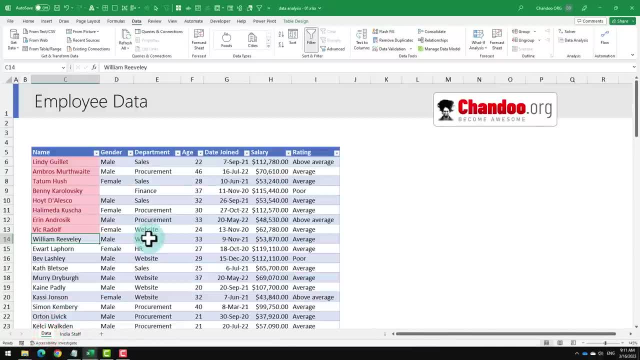 and india data in separate tabs. let's go ahead and combine these two into one giant table and then do the analysis. first up, let's take this data and load it into power query. to do this we can just select any cell here and then from the data ribbon click on from table. 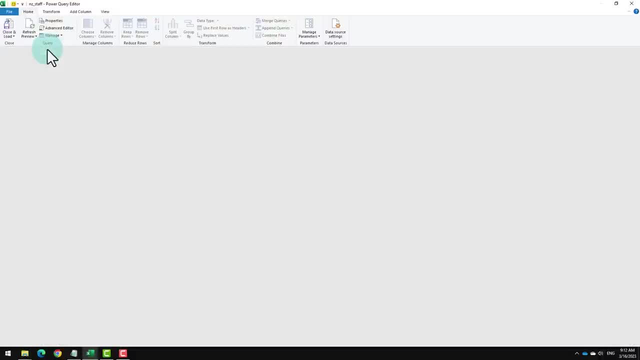 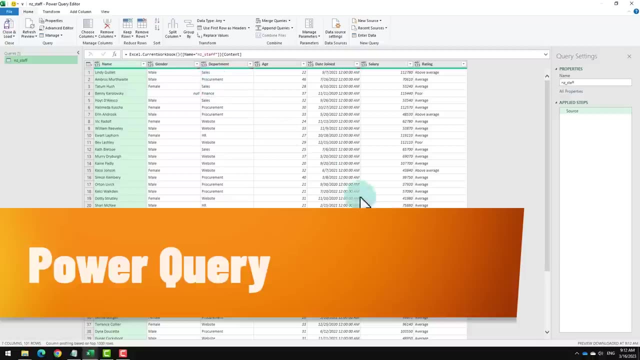 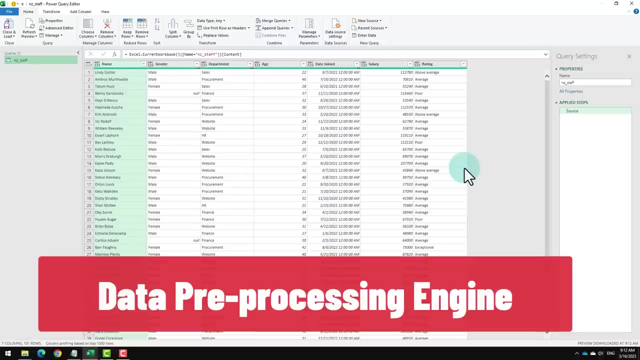 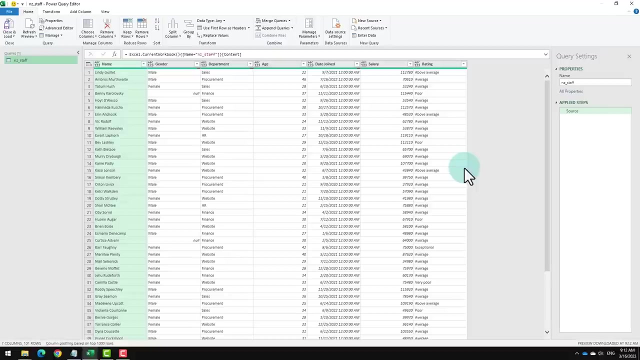 range option. this will load my nz staff into the power query as a table. if you have never used power query before, power query is a data pre-processing engine that we can use to kind of tell excel how we would like our data to be cleaned, what additional steps we want to do on our data and all of that. 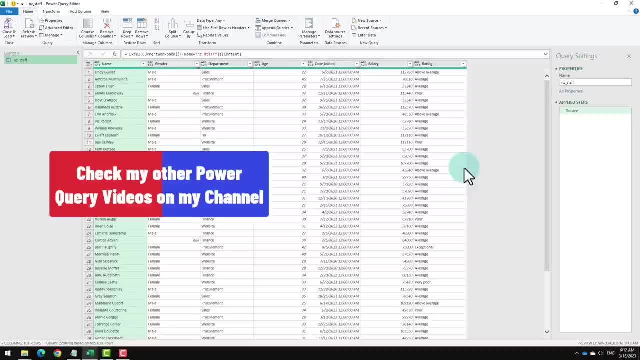 I do have many other detailed videos on power query on my channel, so I will not do a introduction to power query here, but feel free to watch some of the other power query videos that appear as a card up on the top here or in the video description to learn more about power query. 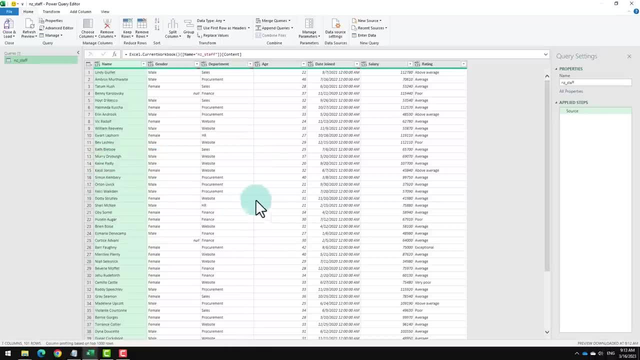 so now that our nz staff data is here, we would like to bring the india staff data also into the power query so that we can then combine both of them. as we are already here, if I try to go back, I can't minimize, nor I can go back to my data, because it won't let me do that while I am. 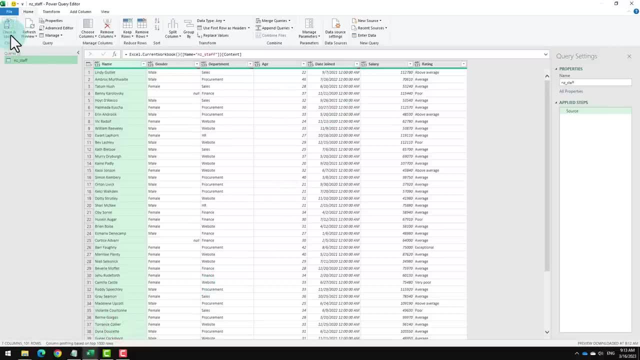 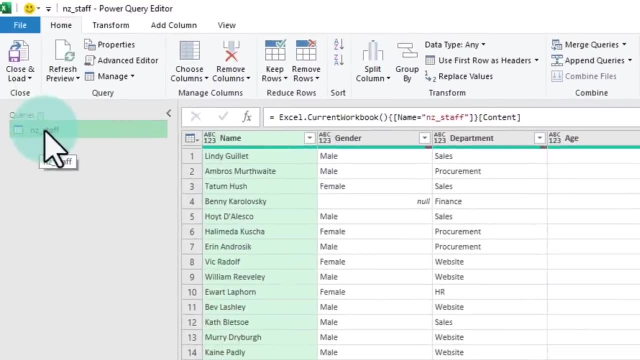 in power query. the only way is to close and load, but that will create additional headaches for us. so, instead of that, what I'm going to do is- because we already have nz- I'm just going to make a copy of this, right click on it and then use the duplicate button to create a duplicate of this. 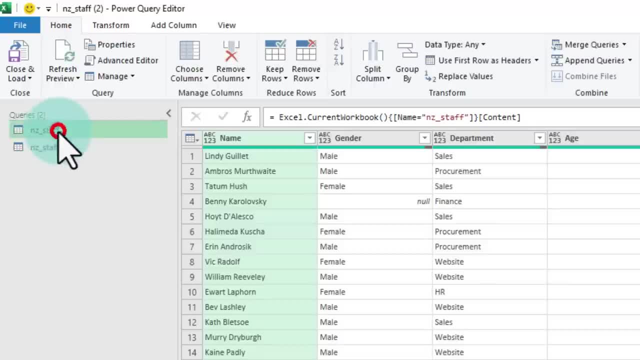 so it kind of copy pastes. so we now have two answers staffs, same data, really. in the second one i am going to look at the formula bar. if you do not have the formula bar here, you can go to the view ribbon and check the formula bar option so that the formula bar appears. 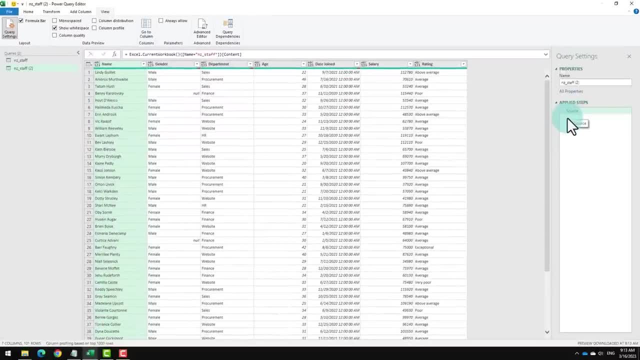 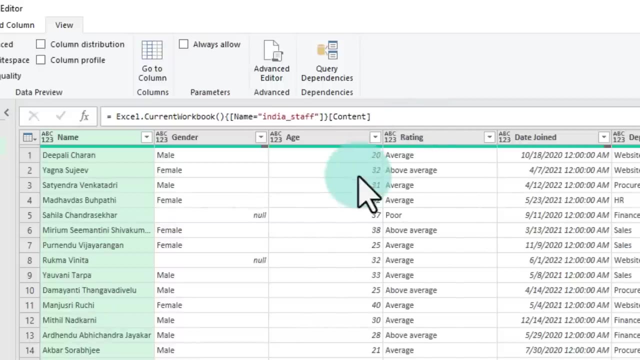 and then from here, make sure that you are selecting the source step. on the second duplicated one and where it says nz underscore staff. i'm going to change this to india underscore staff and when you hit enter it's gonna load up india data here. so now we have. 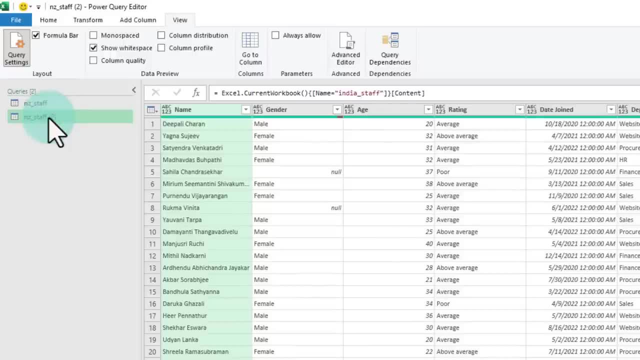 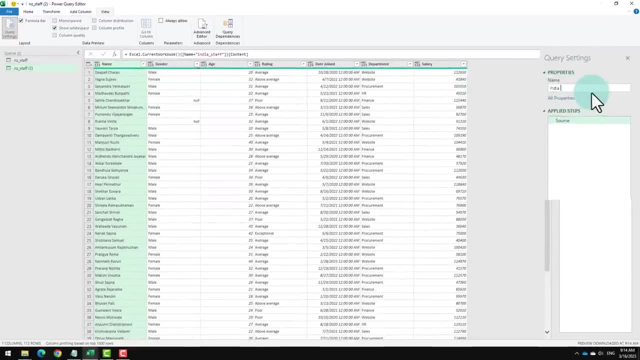 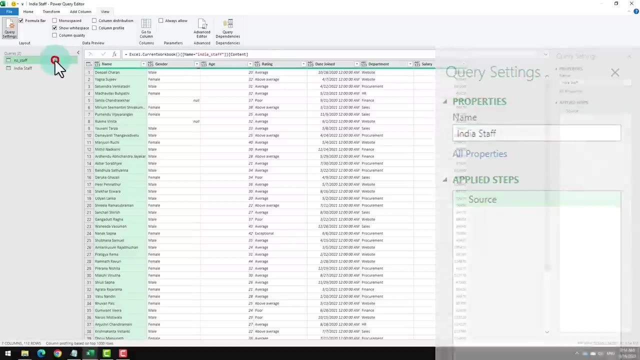 two tables. the first one is called nz staff. the second one is also called nz staff 2, but it shows the india data. let's rename this as india staff and both data sets are here. before we combine this, let's go to the new zealand staff and add. 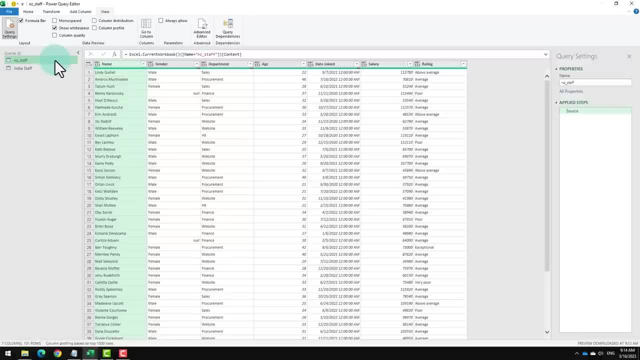 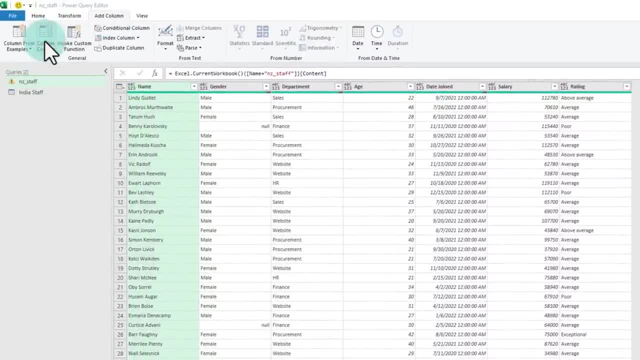 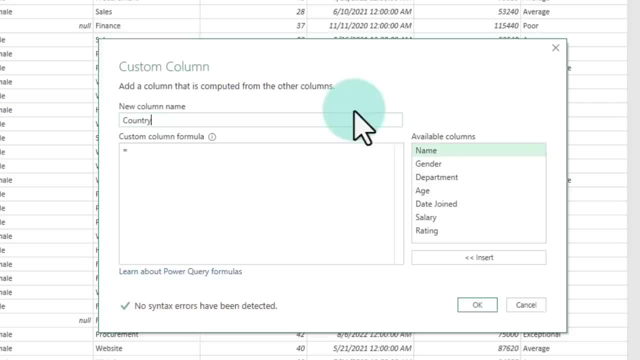 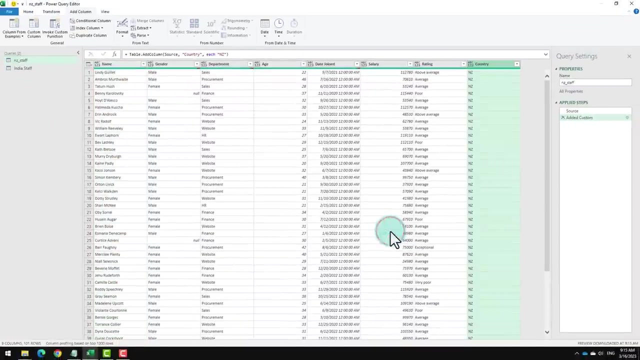 and then say custom column. that column just has to say New Zealand for everybody. so we will name this column as country and here the formula will be just double quotes nz. so it will just put the text value of nz all the way through. this is an easy way for us to identify that this data is. 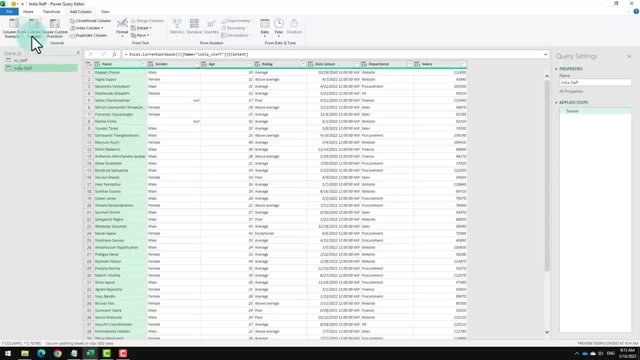 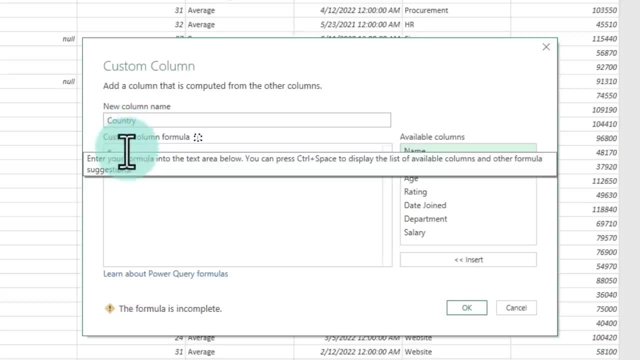 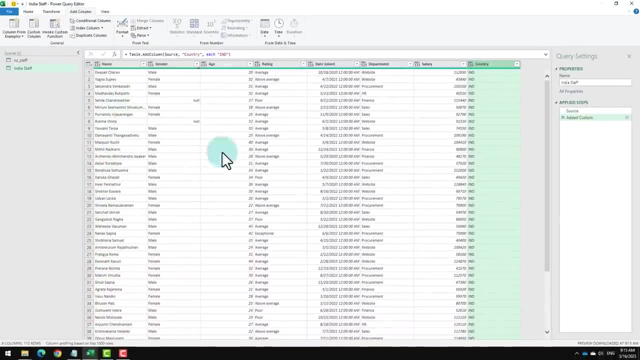 actually New Zealand data. let's go to the India and then do the same. make sure you name the columns exactly same, so country. and so the second table would have India as the country. first table has New Zealand as the country. a quick note here: when you are observing New Zealand data, 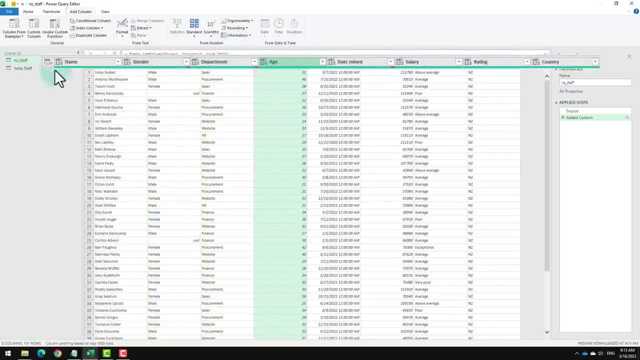 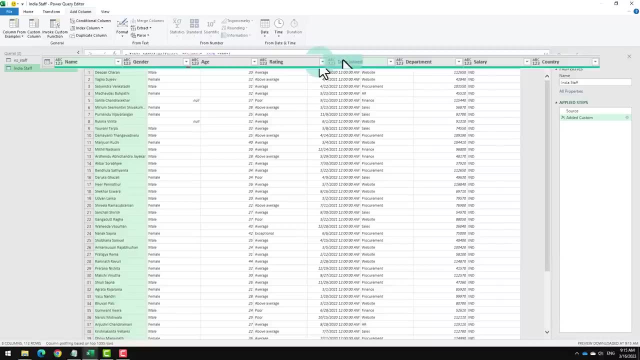 has a name gender department age, in that order, whereas India staff has name gender age rating. so department is somewhere here in the middle. the columns are jumbled, but the names of the columns are exactly same, so this is a important thing to keep in mind when you are consolidating. 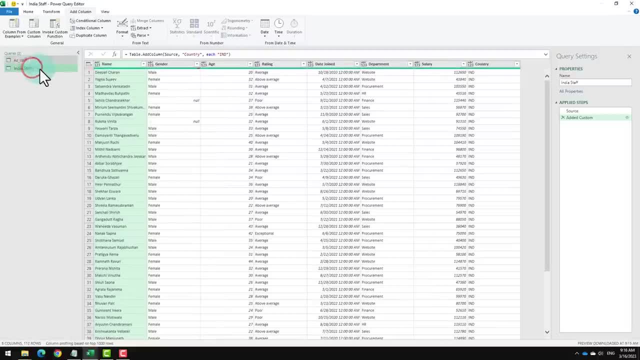 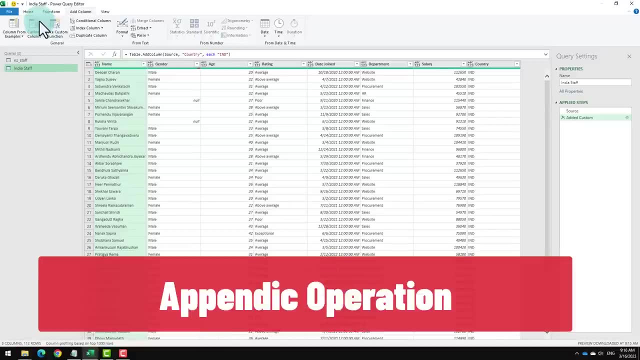 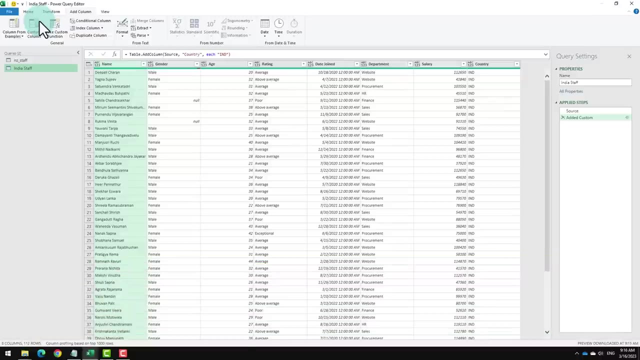 the data. now I do have two tables, but I don't want two tables. I want everything to be combined into one single table. so this kind of an operation is called appending, where you take two data sets that have similar column structure and then append them, stitch them together one underneath another. so go to home ribbon and use append queries button. 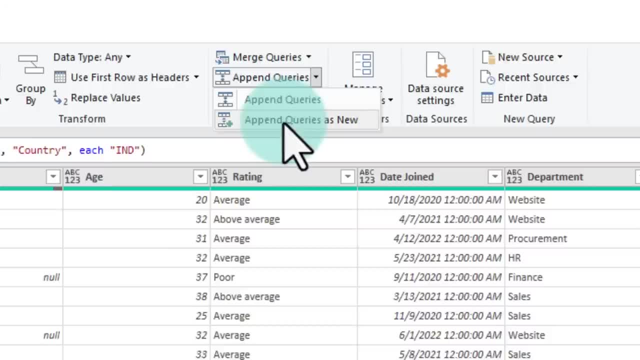 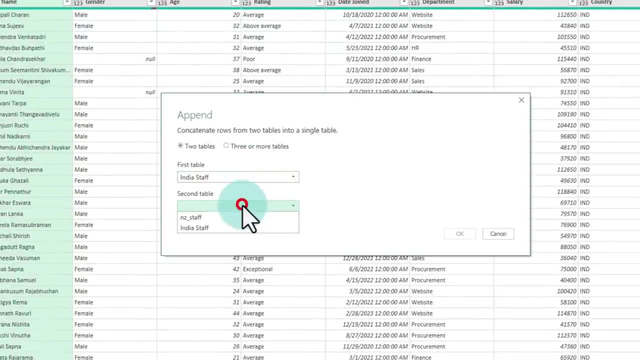 click on that under link here and then say: append queries as new. this will create a new query that combines both my India staff and nz staff. so just pick the tables that you want and it will. when you say okay, it's going to add a new query. and then it will create a new query that combines both my India staff and nz staff. so just pick the tables that you want and it will. when you say okay, it's going to. 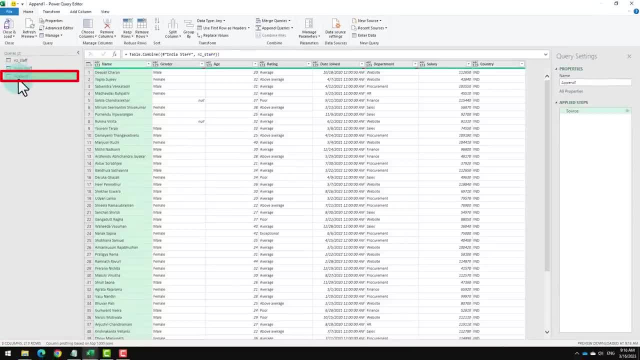 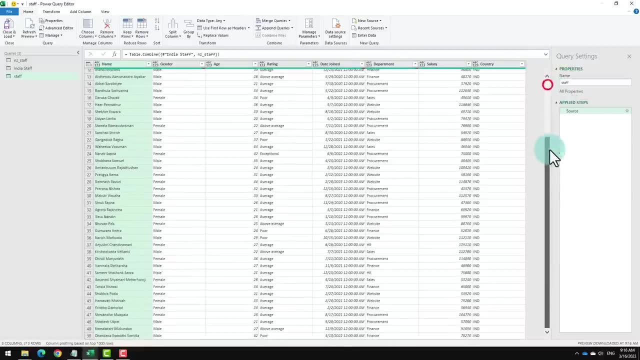 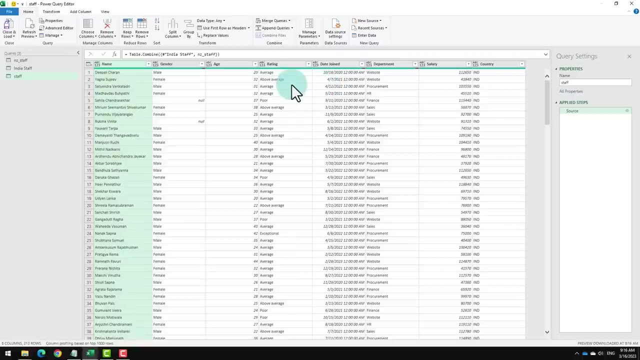 combine everything into a new query. it will be called append one and we can then just call this table as staff. this is all our staff. it has all our India and New Zealand people, everybody one underneath another. at this point, let's do a quick cleaning of the data. the first cleanup activity: 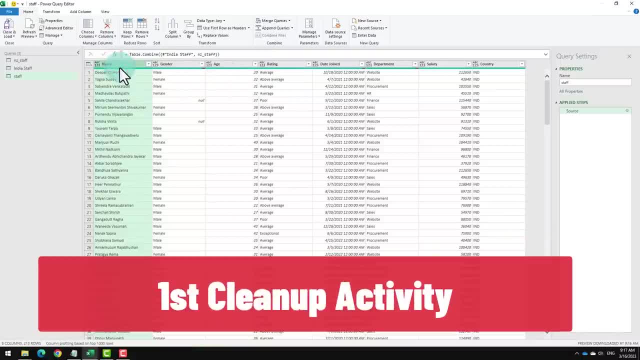 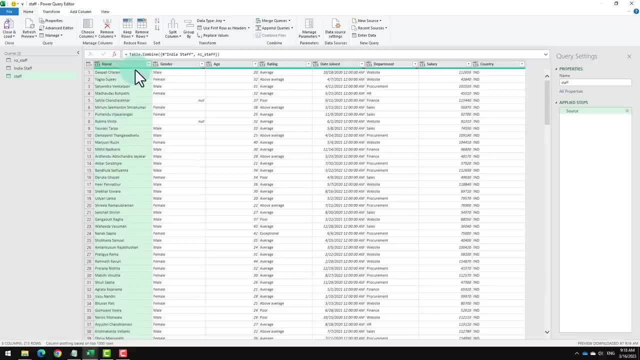 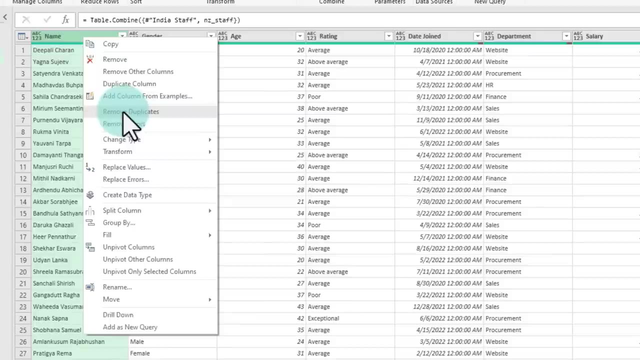 that I would like to do is check the name column and if there is any duplicate values, take out. we'll just select this column, right click and then say remove duplicates. what power query will do at this point is it will keep the first occurrence of the name and then subsequent. 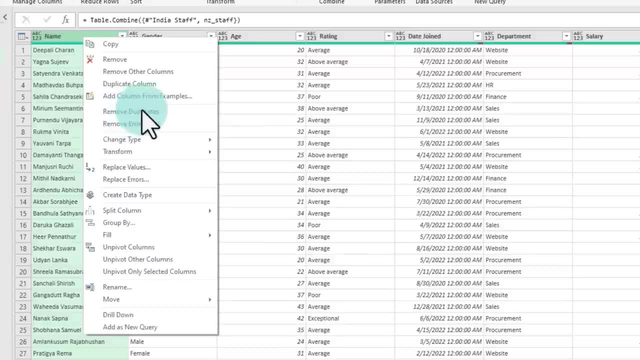 occurrences of the same name will be deleted. this sort of a thing could be a little dangerous to do if you have a large set of data and same name could potentially appear multiple times. for example, if you take a very large company, there might be five people who are called bar phony. 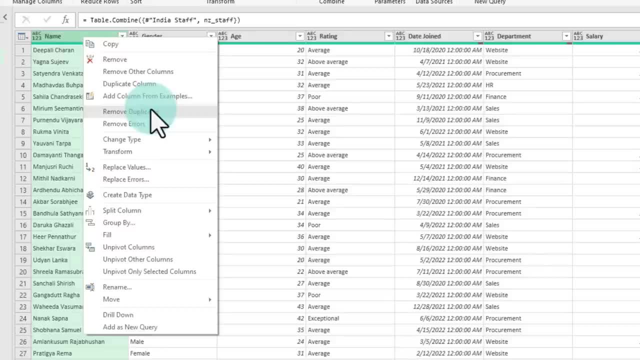 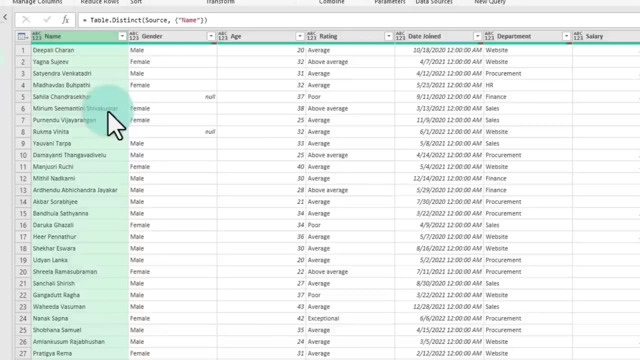 in awesome chocolates we only have one such person. so if you do have such a duplication possible, then you want to pick a column like employee id or some other number that is distinct and use that to remove duplicates. so let's do the remove duplicates on this and it will remove some duplicate values from the consolidated data. 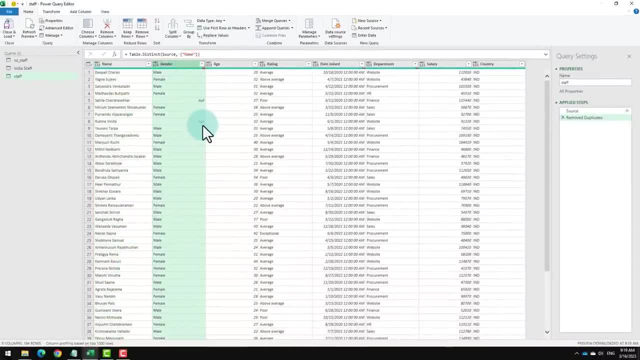 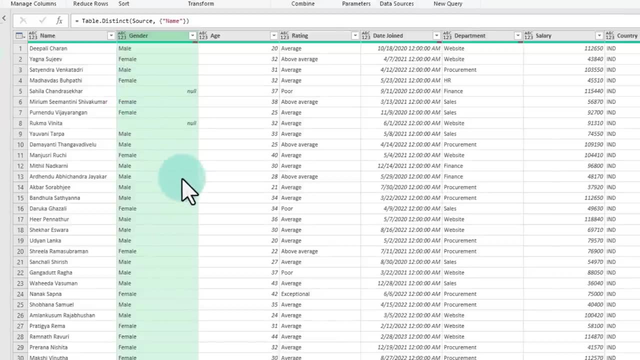 next up, let's deal with the problem of gender values missing. anytime a gender value is not present, what we really want to do is code them as other gender. so to do this we can use a replacement type of a step within power query. so select the gender. 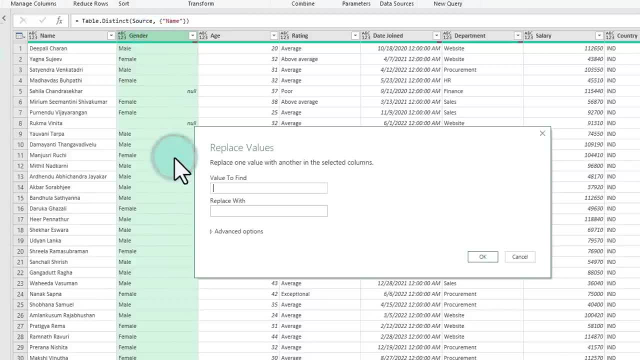 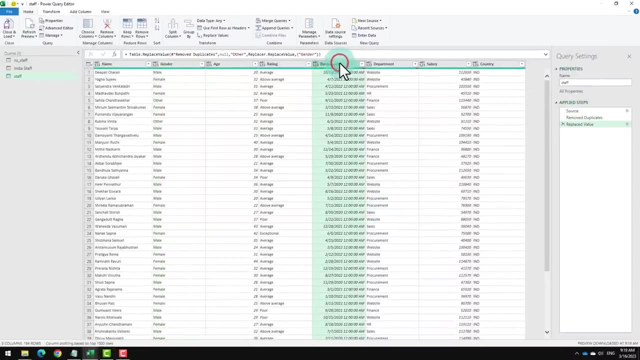 column, right click and then say replace values. the missing genders are called null here, so we can say value to find would be null in small letters and then replace with other. next up I'm going to look at the date joined column. here the green bar tells me that potentially there is a blank. 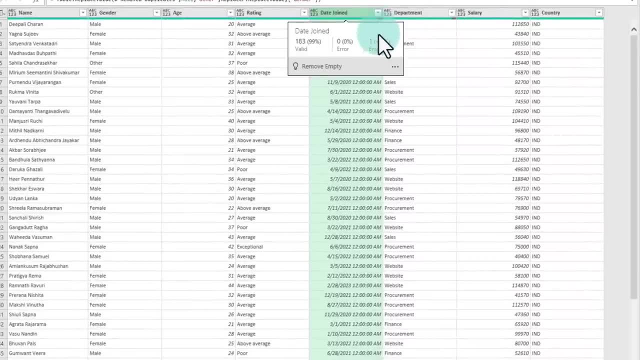 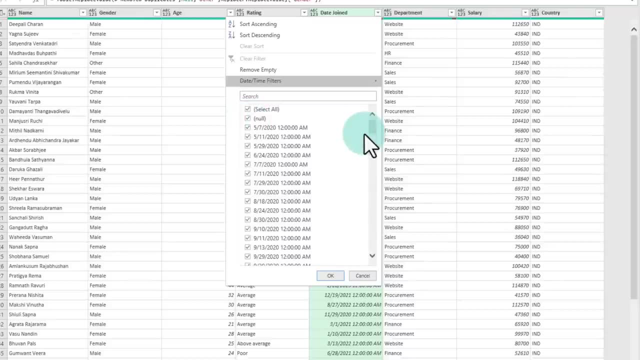 value because it is. it doesn't go all the way to the end. there is one empty value. I'm just going to see what's happening. there is somebody without a date join. I guess this is probably incorrect data, again from a data analysis perspective, if an employee doesn't have a date joined. 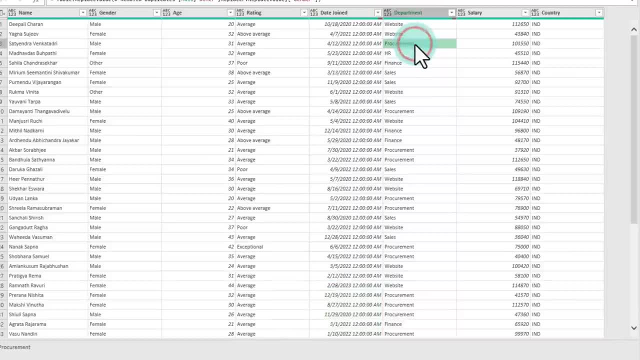 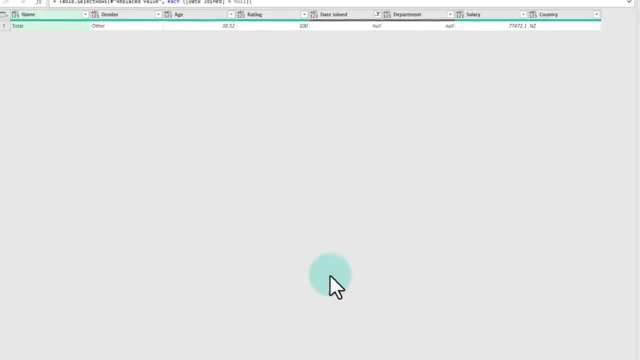 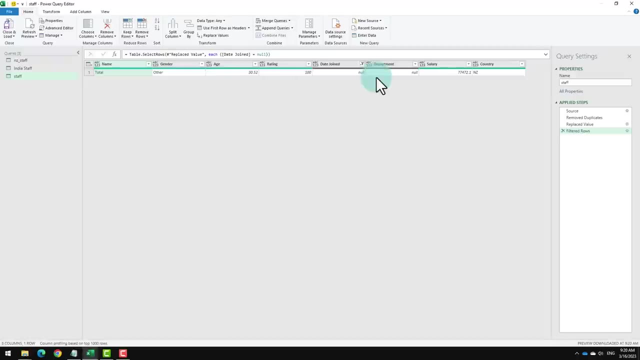 they shouldn't even be in our data. so it could be that that is the grand total row. I'm just gonna delete that. yes, see, this was the total row that we added in our pre-analysis work. that we did so because that total row is there. it kind of appears as the data. this is not actual data, so 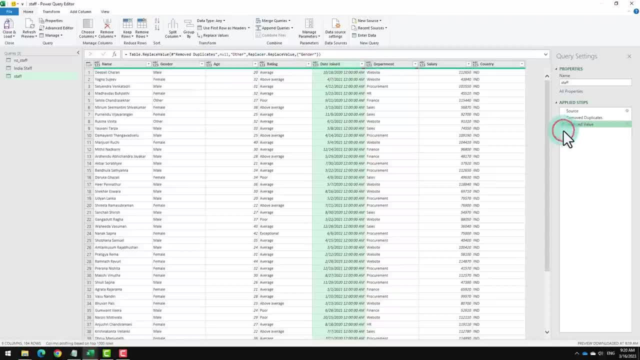 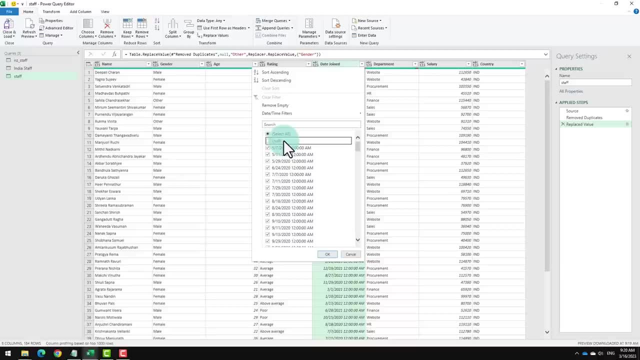 what we can do is I'm going to undo that step by deleting that and then uncheck the null value. so anybody that have null date joined, that means they don't have a date of join. it would be either a total row or in current data, so we can just delete that. 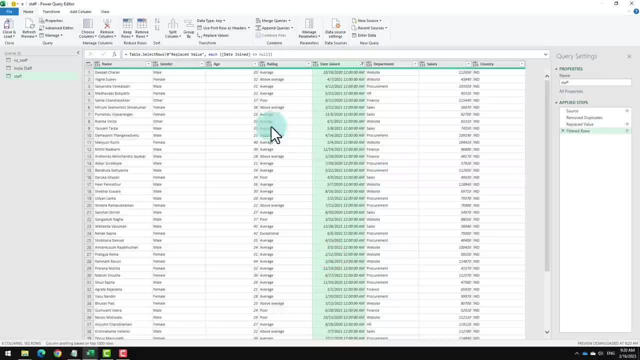 as well, and that all looks good. so we have got name, gender, age, rating, date, joined department, salary and country. so this is the final data. this is the data that we can now take and use to do our data analysis work. so at this point, what we want is we can go to the home ribbon. 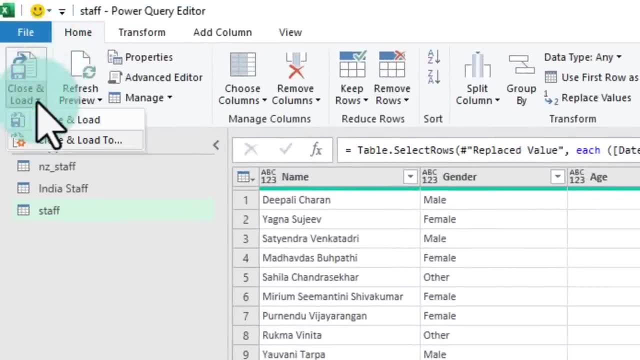 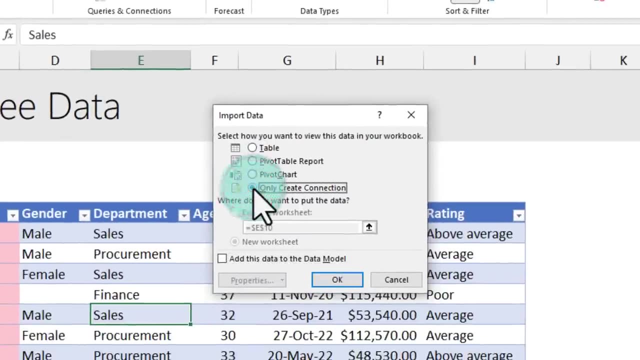 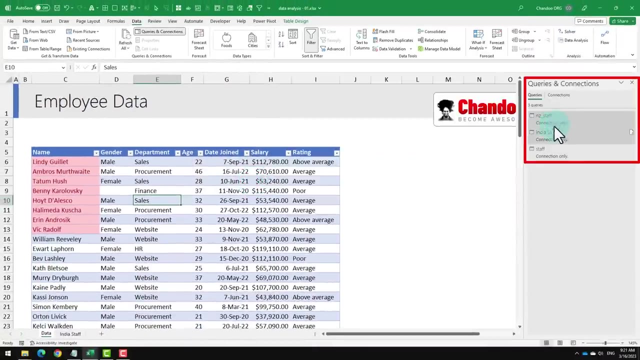 click on the little arrow next to close and load and use the third option, close and load 2, and then for now I'm just going to say just make a connection, don't load anything, and click OK. so this will load all the three queries that we built: nzstaff, India staff and final staff as 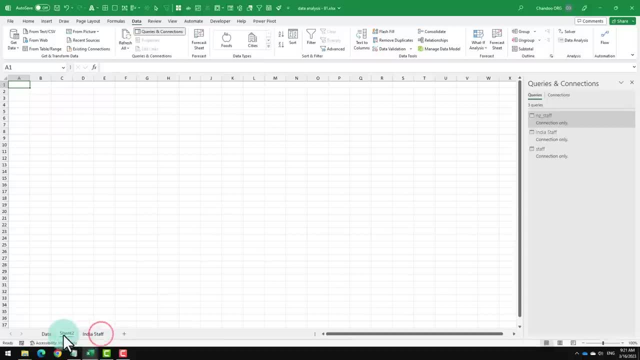 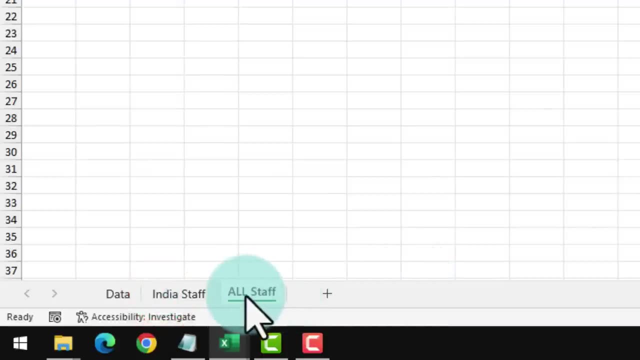 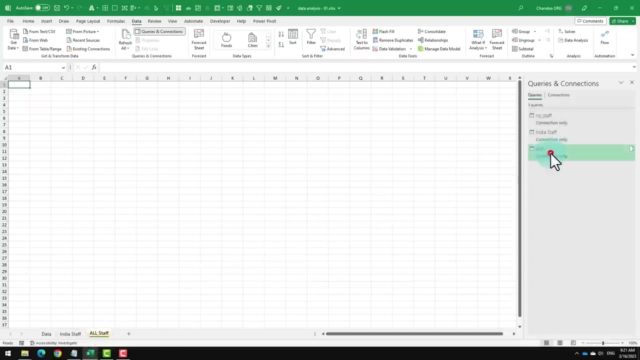 connections. now let's add a new tab and this tab we will call this as all staff and this is our master data. so I'm going to right click here, tab color and then make the color yellow so we can quickly spot it when you have multiple spreadsheets. so in this all staff page I want to load my all the staff. so 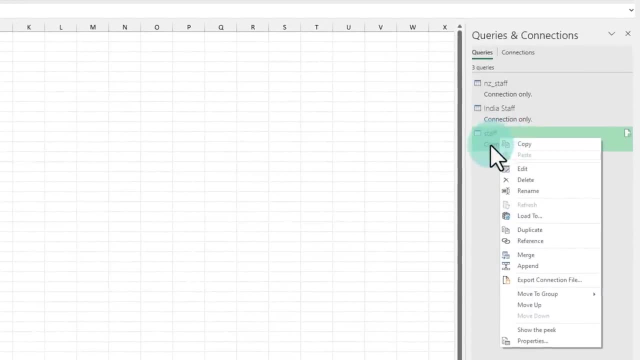 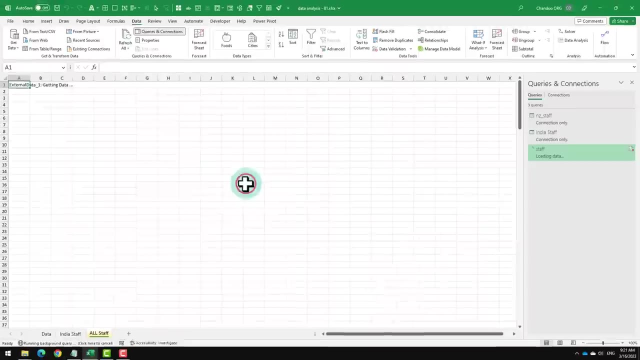 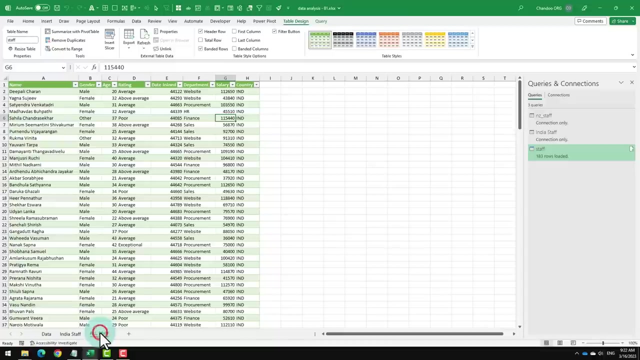 right click this one and then right click on the staff and then say load to and load it as a table in the existing worksheet here so that it will load the all staff data here. so we started with the blue table, orange table, combined and cleaned everything to end up with this data set that has all our employees. you. 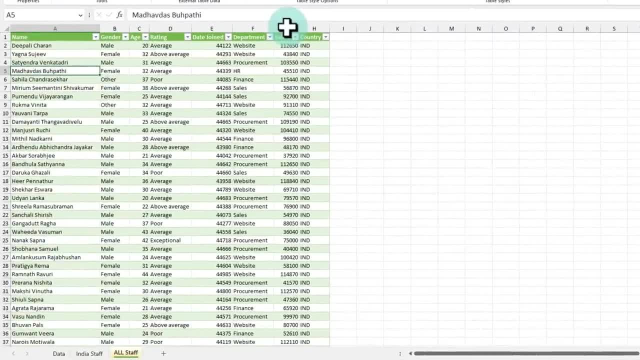 might think, what is this? all staff data? and that's not the case. you can see that. think: oh, does the staff have same kind of salary in India and New Zealand? yes, awesome chocolates. even though it has a branch in India, the salaries are still paid in dollars. so we can combine. 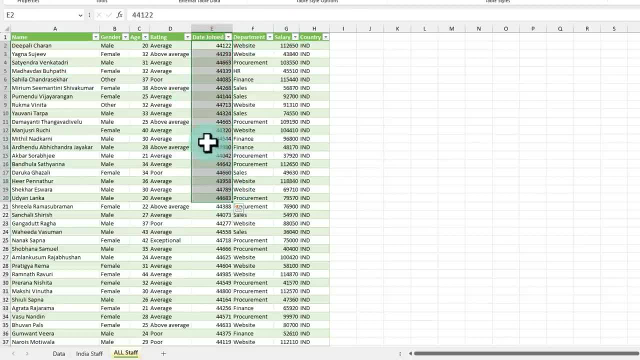 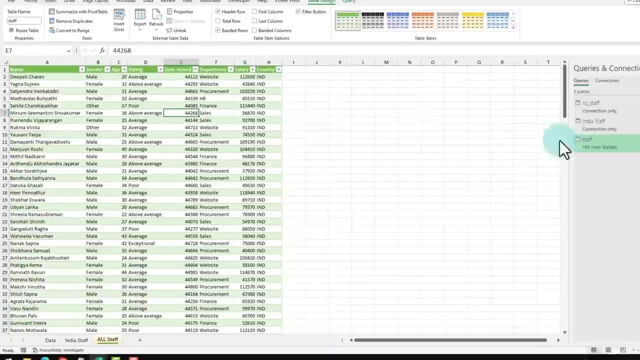 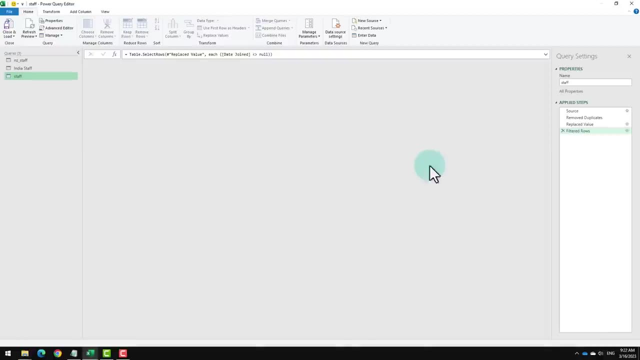 everything here. what about the date? the dates look like numbers again. we can apply date formatting again on this column, but let's just do that in power query. so I'm gonna right click on my staff data and edit the query quickly, jump back to power query and select the date joined, right click. 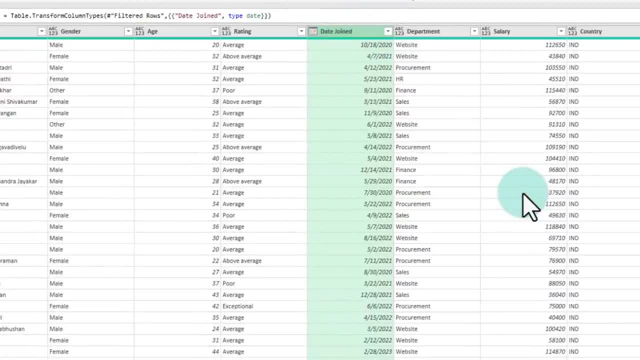 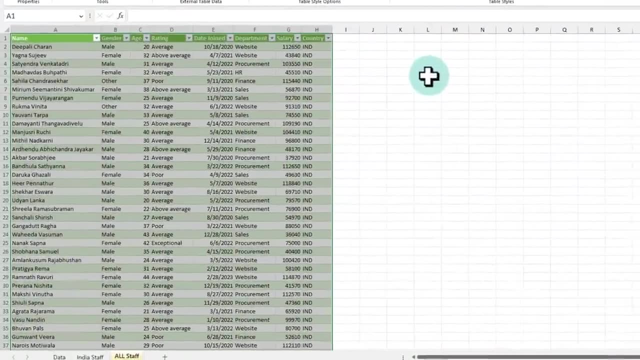 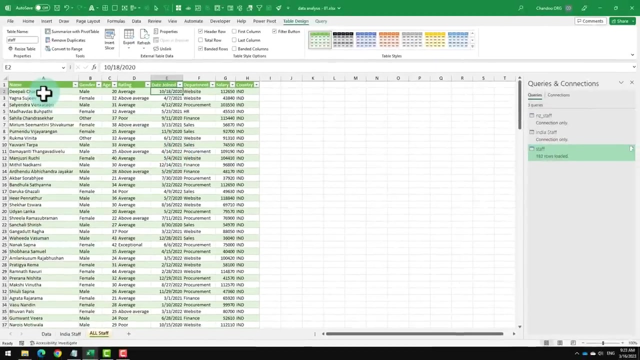 change type to date, so that we tell power query that this is actually a date column, and click on close and load, so that when, when the data is loaded into excel, it will appear as a date value. perfect. so now that we have cleaned our data, let's go ahead and answer some business questions. 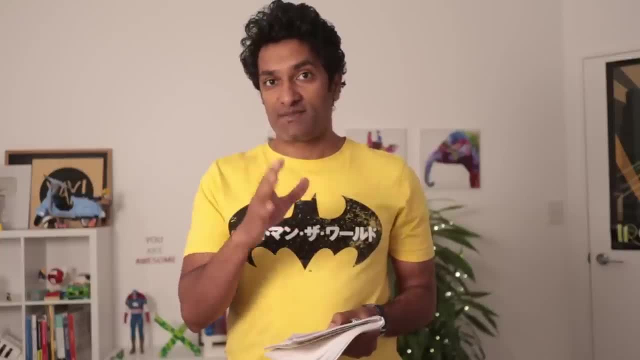 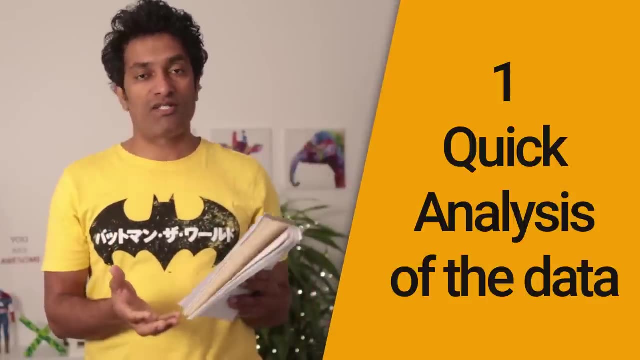 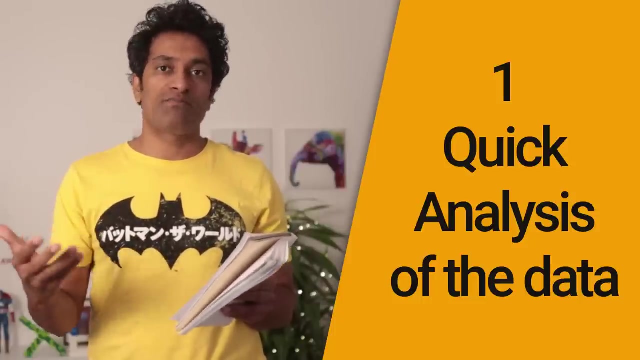 I have got five business questions for us to answer as part of this section of the video. these are a quick analysis of the data, so we have got all our consolidated employee list here. I just want to know who are these people? how many are there? what are some quick statistics about? 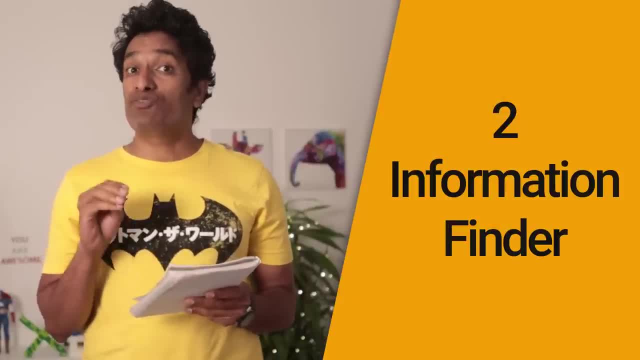 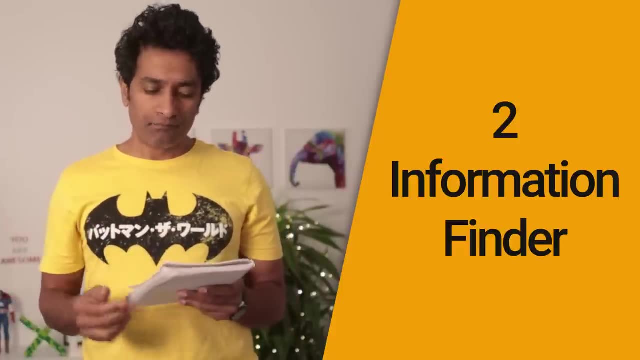 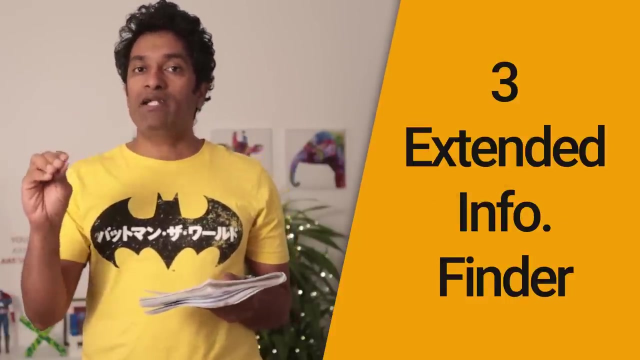 them. the second question is: we would like to build an information finder. it is where I can put in a name of an employee and I know everything about them. and then the third one is: we want to extend this information finder so that we can ask about a department and get the entire results of. 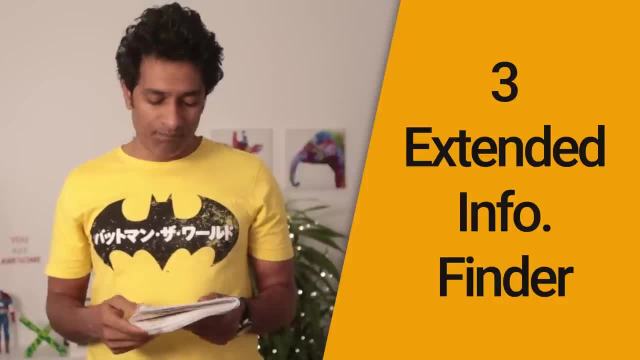 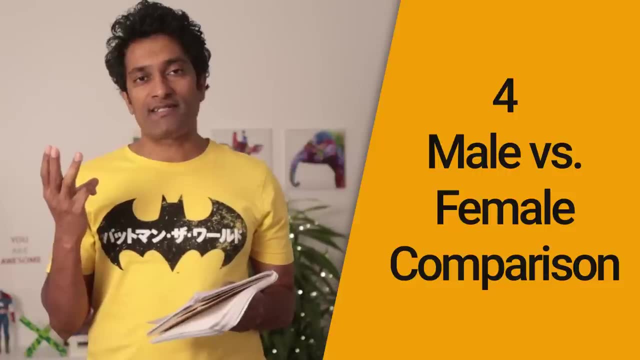 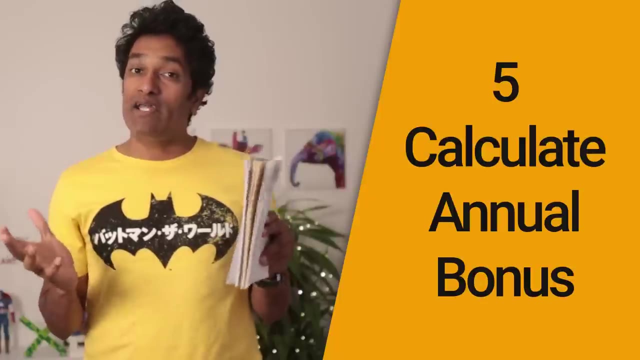 that department as a clean view for us. and then we also would like to do a male versus female comparison of the data. we have got three genders in the data, but for this purpose we have just got to look at male versus female. and then, finally, we have had a very good year of chocolate sales. 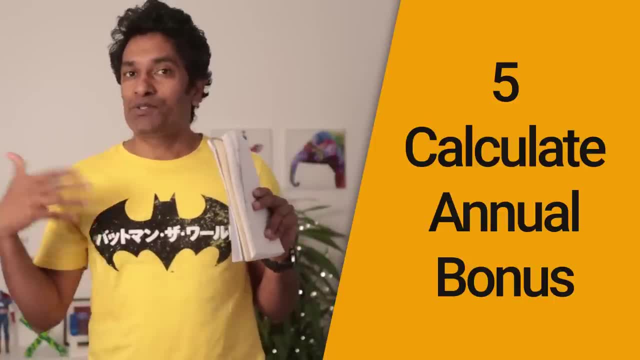 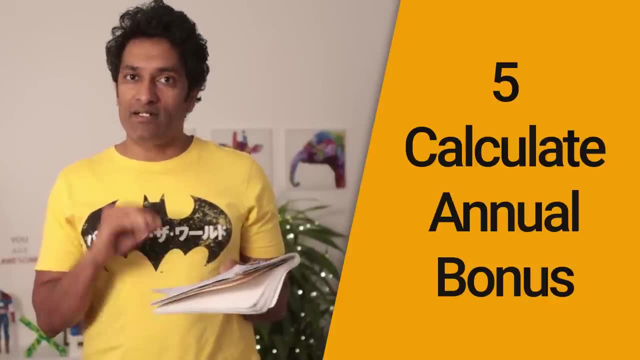 in 2022. So to celebrate that in 2023, Awesome Chocolates would like to give a bonus to all our staff, so we want to build a bonus calculator using excel and then understand the process for calculating the bonus based on the employee data. 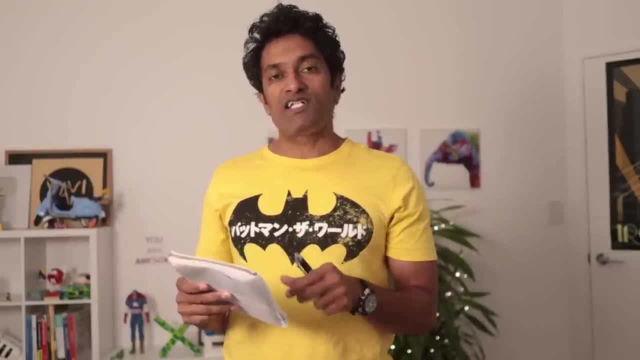 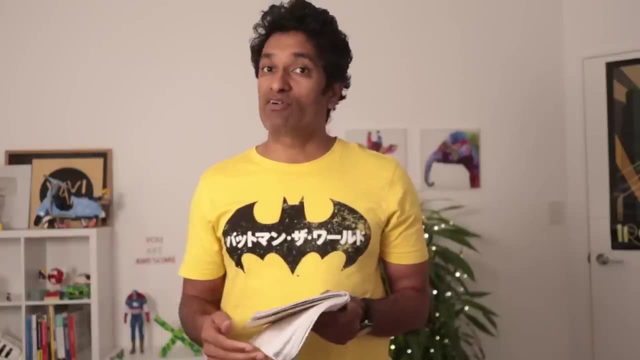 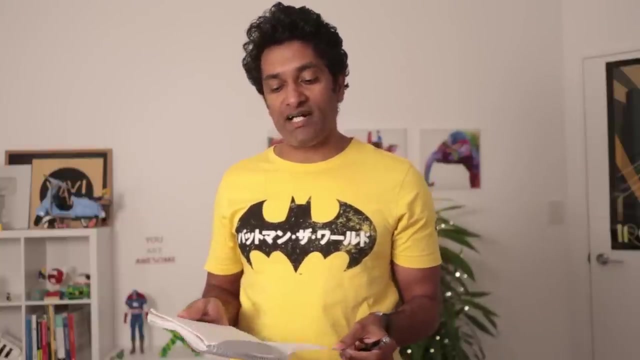 so that is the second part of this video. in this process we are going to learn some cool excel functions, Excel pivot tables and other simple tricks and powerful useful things in Excel. Once we finish this, then we are going to do some analysis of the data. 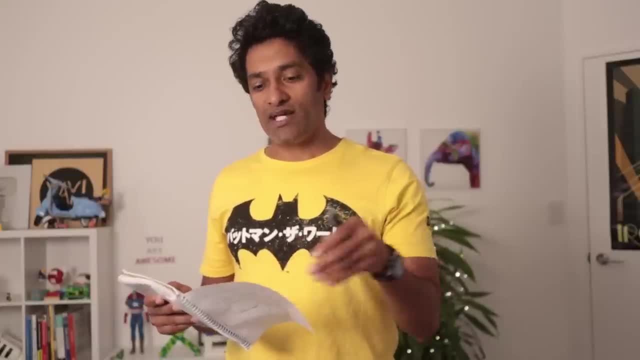 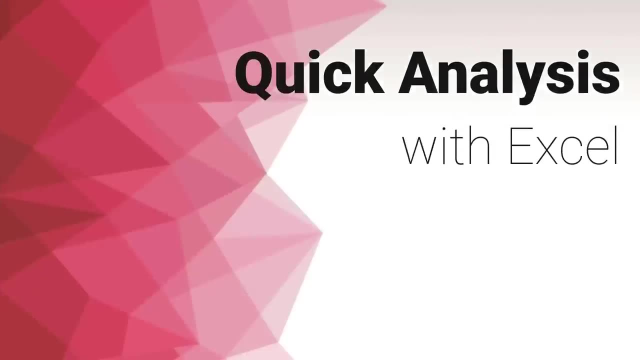 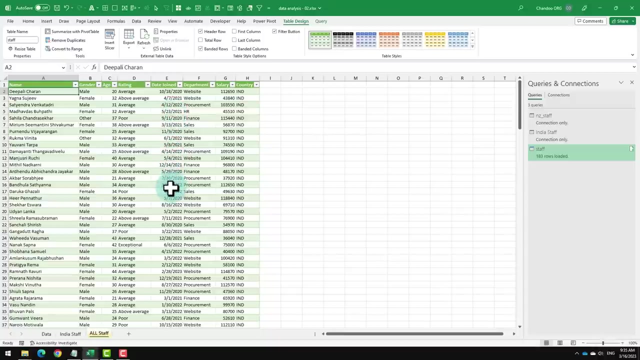 using a different set of questions. We'll go there. after we finish this, Let's go. Our first question is a quick analysis of the data to understand what is it that we got here. We could do this with either pivot tables or formulas. I 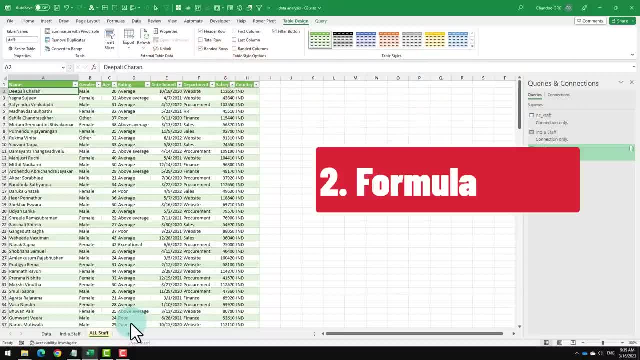 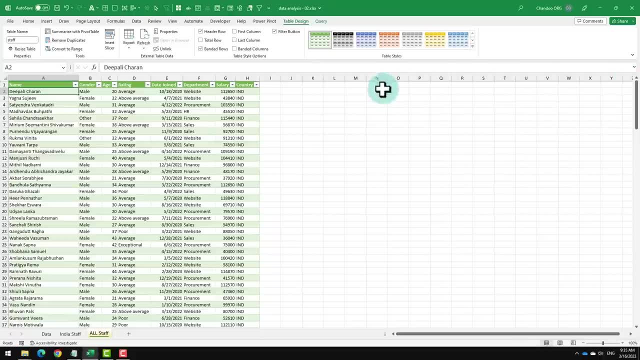 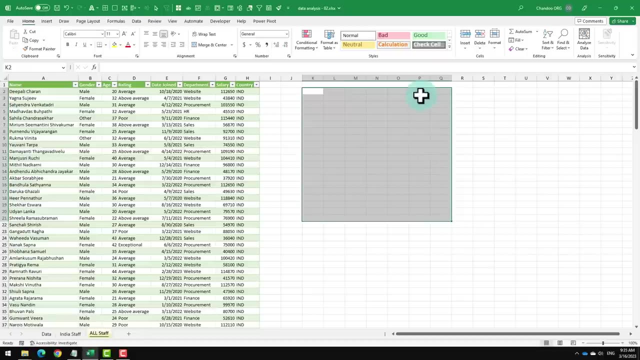 recommend using formulas because that way we get to learn some of the cool and helpful functions in Excel. For the sake of simplicity I'm going to build our formulas right next to the data. That way it's easier for us to kind of cross check and verify the results. But in usual business situations you may want. 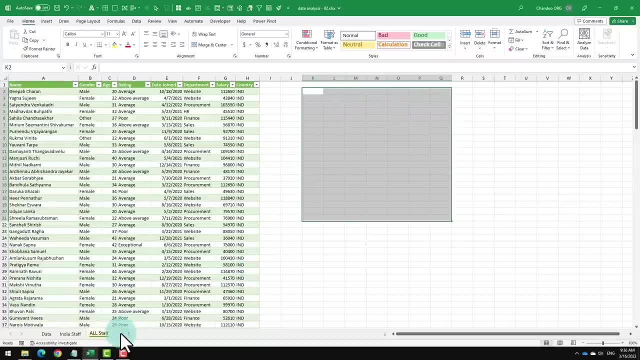 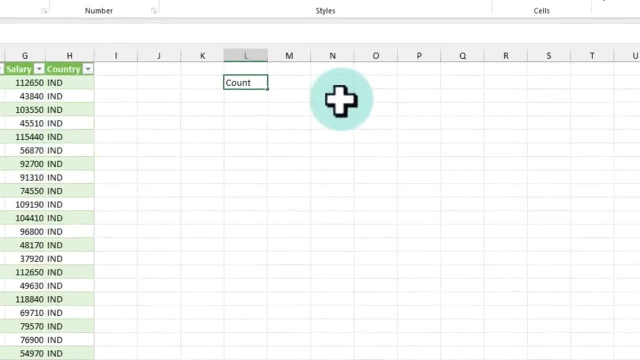 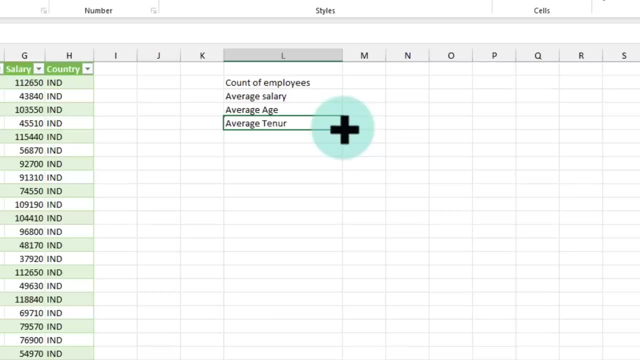 to build these formulas in a separate page or a tab, rather than everything being here. So the things that we want to calculate are count of employees, average salary, average age and then average tenure. Tenure refers to how long an employee has been with us. Given that we know the 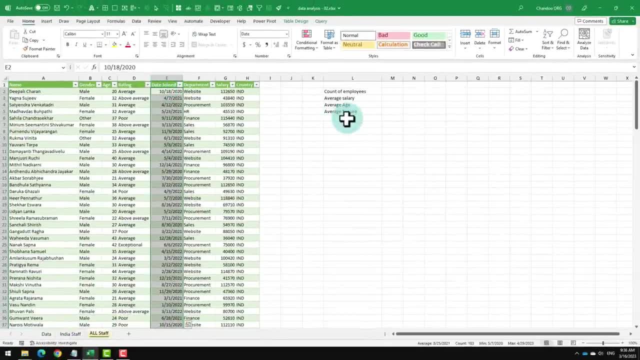 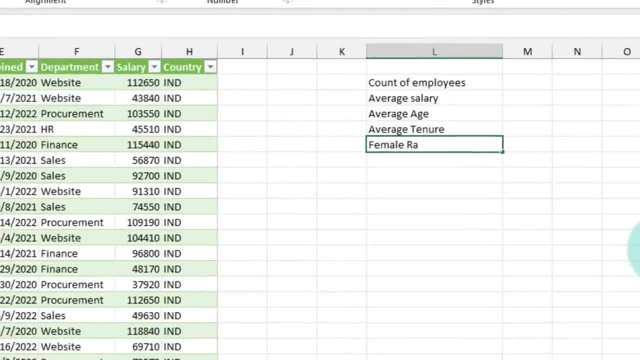 date joined and we know what current date is, we can calculate how long a person has been with us. And then we would like to calculate female ratio. This is percentage of female staff as against the total staff. To get a count of employees, we just want to count how many values are there in one of the 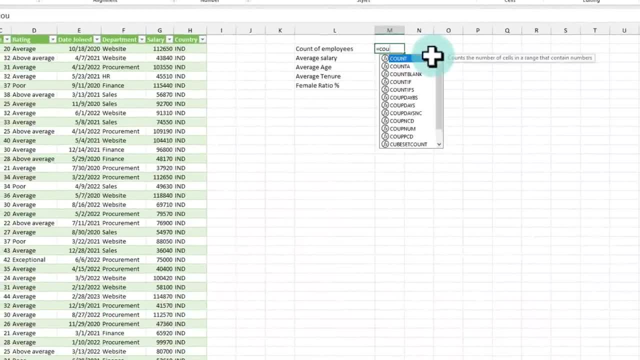 columns. Let's pick the name column, So this one. we could use the countA function. Excel has two kind of counts: count and countA. Count refers to count of numbers. Because we are looking at the name column, we should refer the countA. 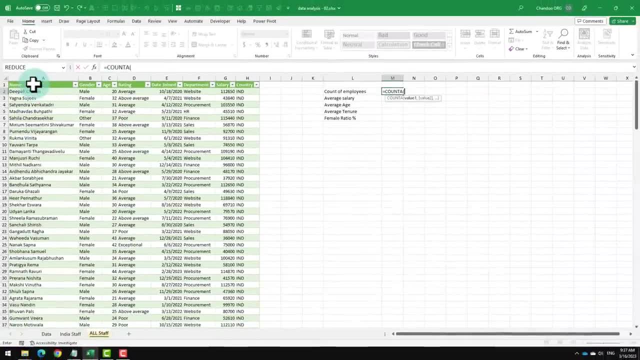 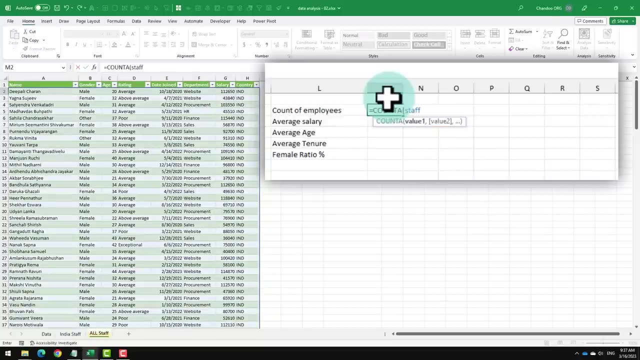 function. So countA of the name column. here You can use the mouse pointer and point to the column, like using that black arrow trick, or alternatively you can also type the name. here You simply type the table name, which is staff, open the square bracket and then point to the name column with n letter and then tab. 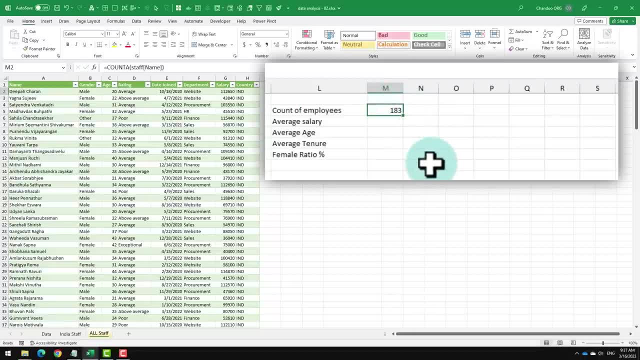 to complete that. So we have 183 people in our data. Make a note that this is after we have removed all the duplicates. So if you actually count how many people are there in the original data sets, this number will be a little less than that, because some people are. 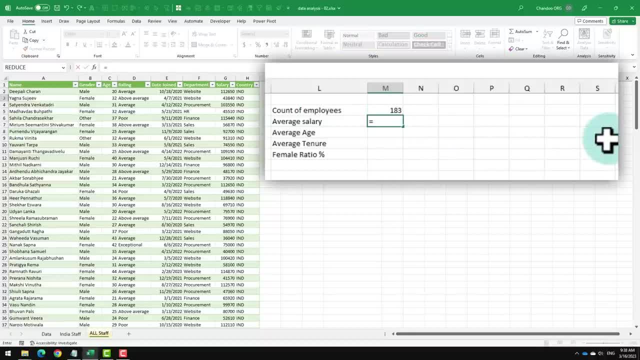 removed due to duplication. Next up: average of the salary column is using average function, Average of salary column. So select like that. Average salary is 77000.. This is the average of the salary column. Normally, when we calculate summaries in business situations like this, it's a good idea to 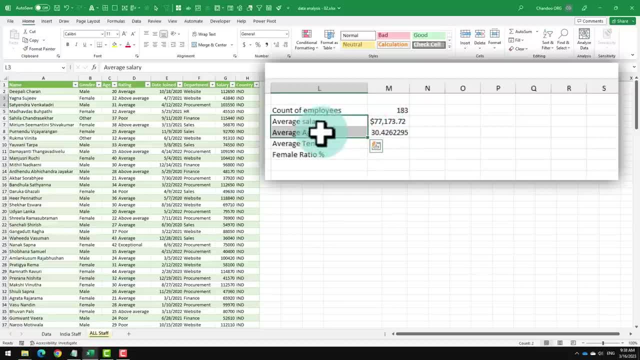 not just calculate the average, but also calculate the median. That way you will understand if the data is a little bit too wild. Average is sum of all the numbers divided by count of the numbers, whereas median refers to the midpoint, if all the salaries are arranged in ascending or descending. 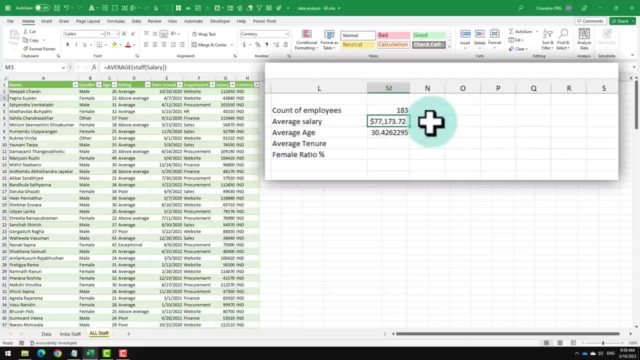 order. what is the middle point looking like? so let's calculate median here. the median can be done with median function and again select the column and we can see that. so for example, here my average is 77 000, whereas median is 75 000.. this kind of a difference indicates that there 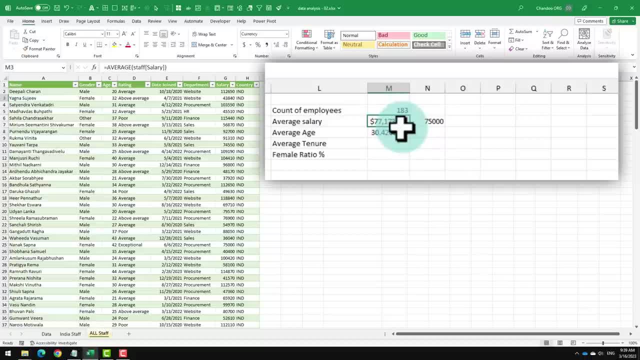 are probably a few people who have very high salaries, and hence the average is getting pulled towards the other side, not by much, but a little bit. let's do the median for ages as well. median of staff age. the average age and median age are pretty much similar, so that distribution. 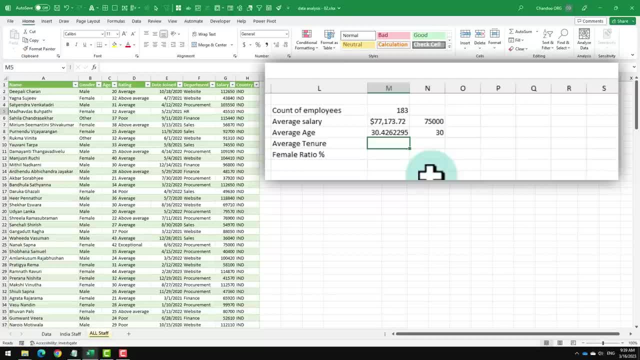 looks all right to me. how do we calculate the average tenure? we only have the date joined, but we need to calculate tenure first before we can average it out. we could, of course, write a big, complex formula that does all of it in one go, but that kind of 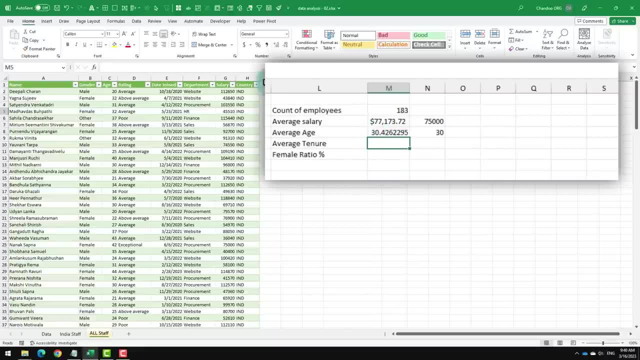 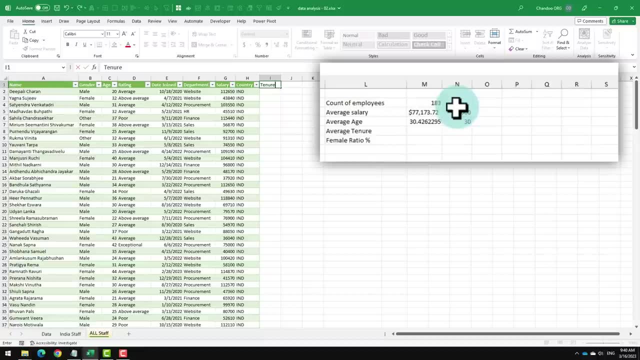 thing is not recommended. it's a good practice to add the tenure column first and then average it out. so let's add a tenure column to the table. when you have a table, if you type a value right next to it and hit enter, it will add a column to the table. the tenure can be: 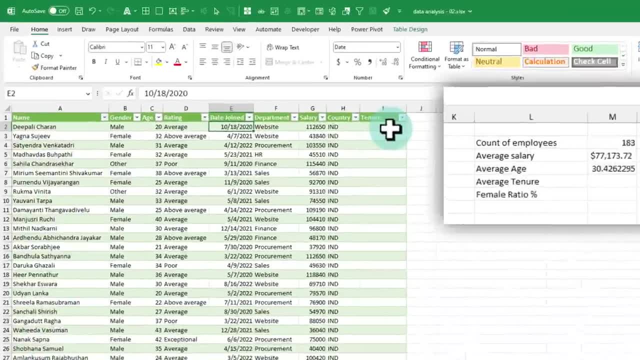 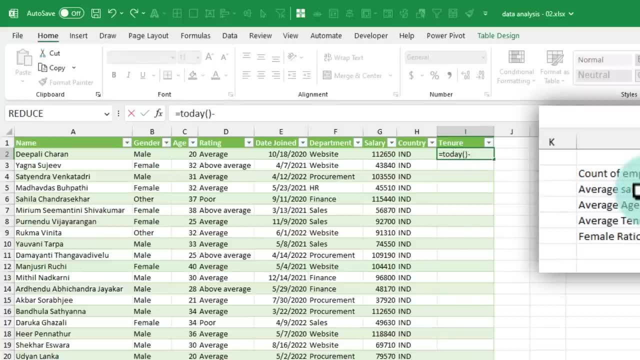 calculated by taking this date and subtracting that from the current date. to get the current date we can use the today function and then, minus of this, that will give you a number. unfortunately here excel has formatted that number as a date. but if i select the column and then change the formatting to general, 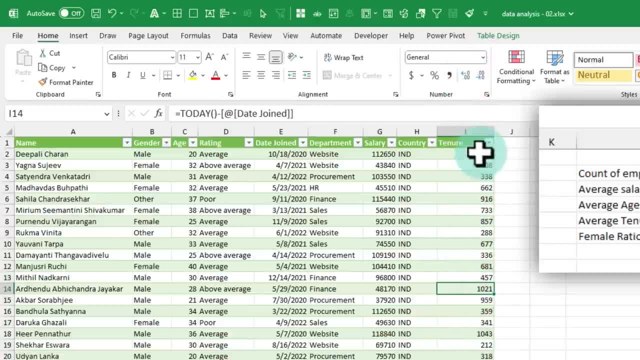 we can see how many days each of these people have been with us. for example, this person, pali charan, has been with us for 879 days. now, this kind of a number looks a little bit ridiculous, so what i want to do is do this calculation and then divide that with 365 so that we can get that. 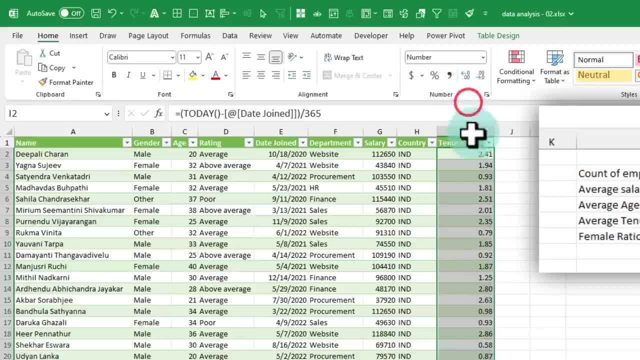 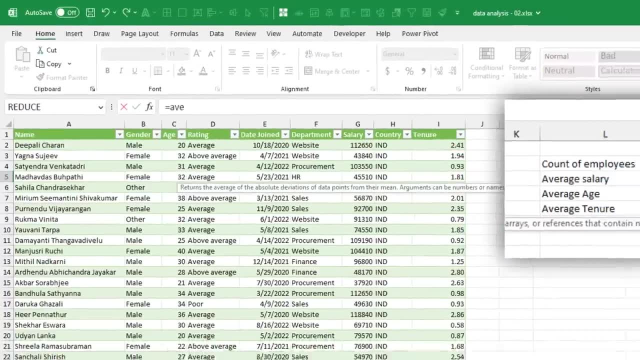 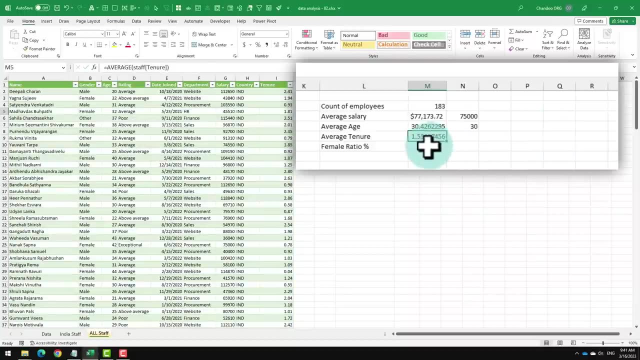 in years, and then let's just apply number formatting here: 2.41 years for this person, 0.93 for that person. now let's calculate the average of that average of staff tenure column and then finally, we want to do a female ratio, that means count how many females. 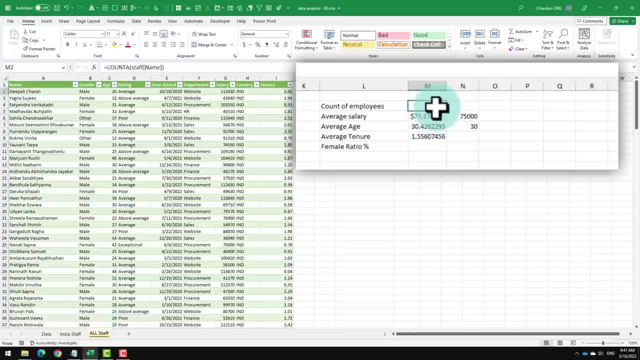 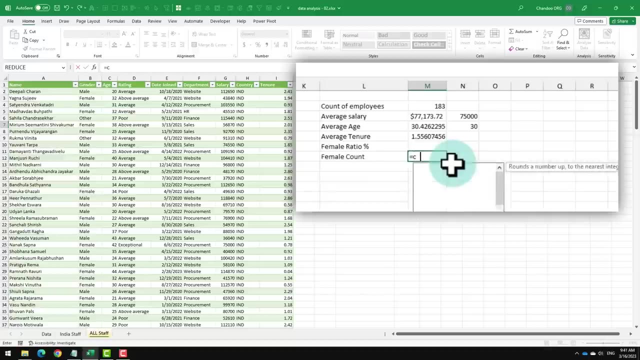 are there and then count that as a percentage of 183. we'll do that in two steps so that it's easier to see the process. first we'll do a female count. this is where i want to count how many gender values are female, so we could use the function count ifs to do this kind of things. 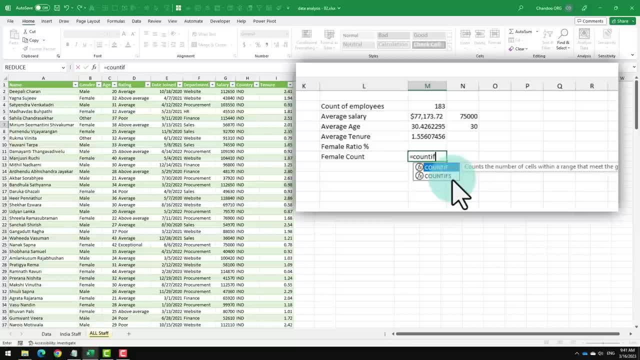 excel has two sorts of functions: count if and count ifs. i always use the ifs functions wherever possible. this way it's one function to remember. we don't need to know what the other one does anyway. so count ifs, gender column, and then, within double quotes, we can type female. 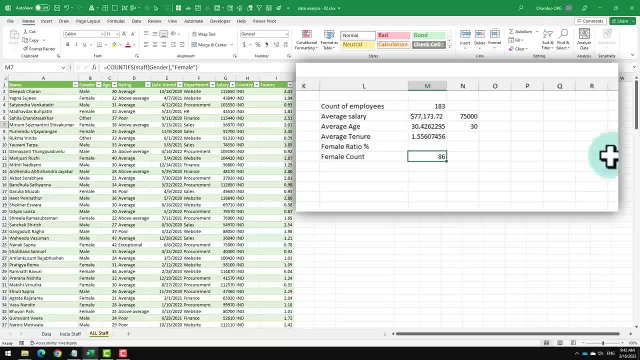 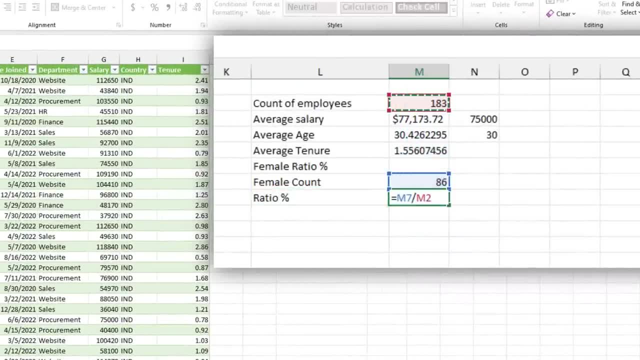 so we have 86 female employees. hence the ratio would be 86 divided by 183.. to apply percentage formatting to this, you can press the ctrl shift 5 for this ctrl shift 5 or ctrl percentage symbol on your keyboard and that will apply the percentage formatting to this 47 female ratio. pretty good, almost one in every two employees. 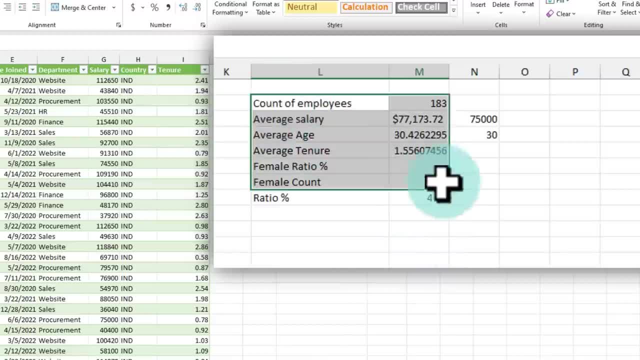 is a female at awesome chocolates, so we've computed that in our imperialурl engagedاد. So this is a quick summary. Like I said, we could use either formulas or pivot tables to build these kind of things, As I plan to introduce pivot tables later on in this video. 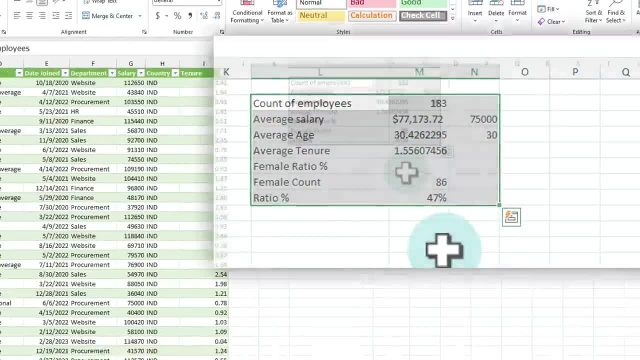 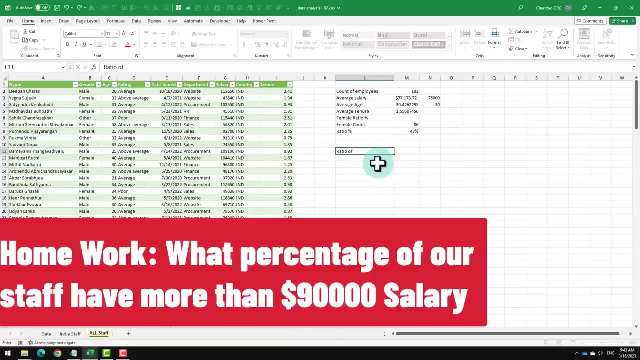 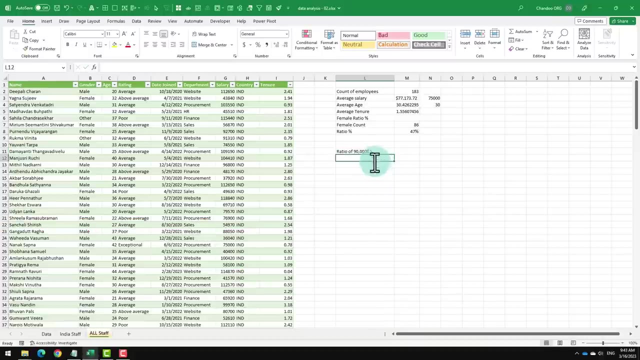 I thought we can learn some of the formula versions of this and do that. Here is one homework problem for you. I want to calculate the ratio of $90,000 or more people. So some of our employees have salaries. The salaries start from $33,000 all the way up to $119,000. 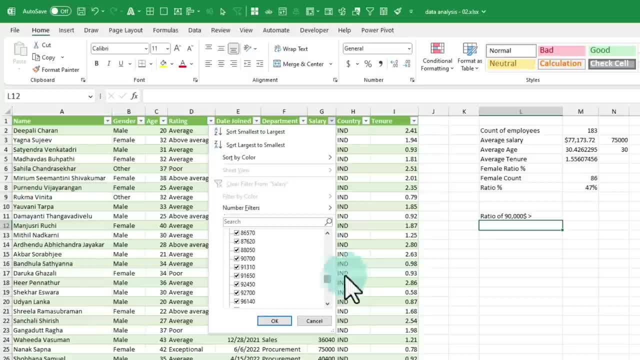 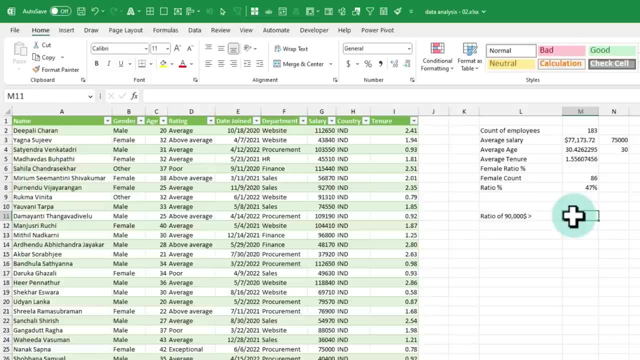 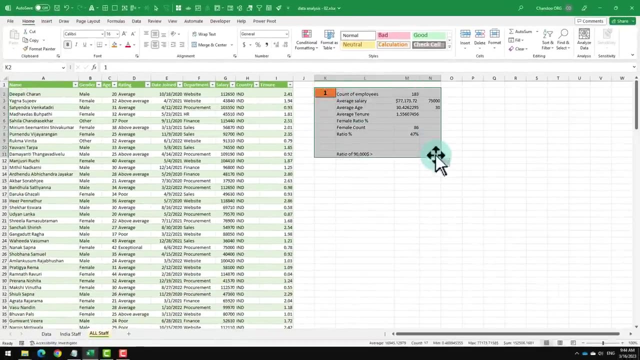 And we just want to see what percentage of our staff have more than $90,000 as salary. So calculate this using a formula- either one formula or a bunch of different formulas- and then print that value there as your homework. So that is the first section of the business. 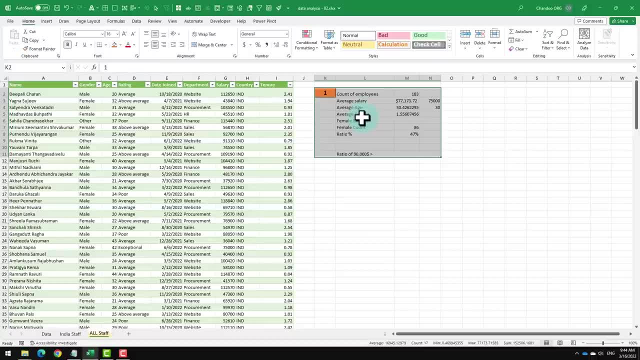 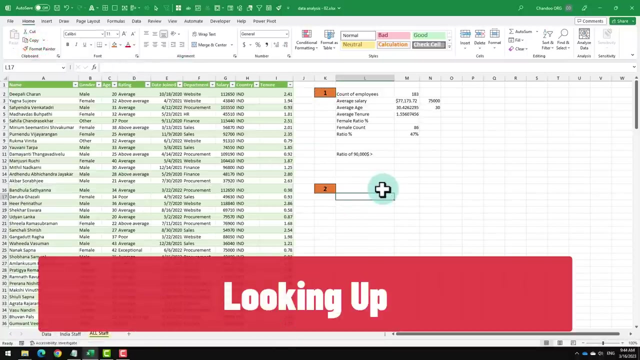 question, which is doing a quick summary of our data. For our second section, we would like to build a information retriever or information finder wherein if I type an employee name, I would like to see their entire details printed to me neatly underneath. This sort of an operation is called looking up and we can use the lookup. 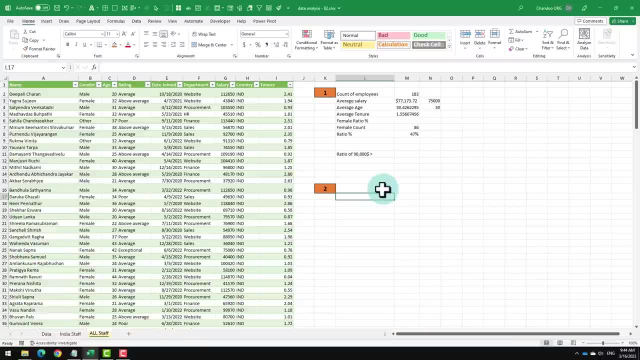 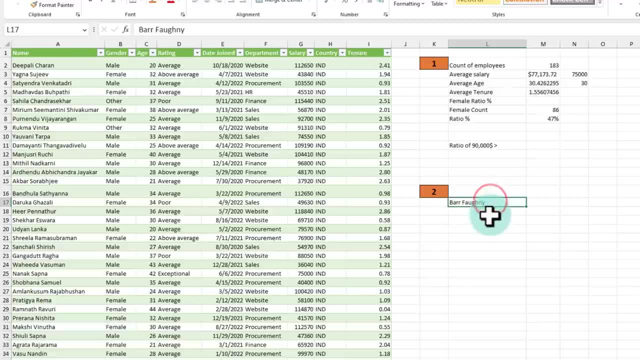 functions in Excel to do this. We can also do it manually. For example, if I have a name like Bar Forney and I just want to know where this person works when they have joined our organization, how much salary we are paying them, etc. I can use the filter button here and then just type. 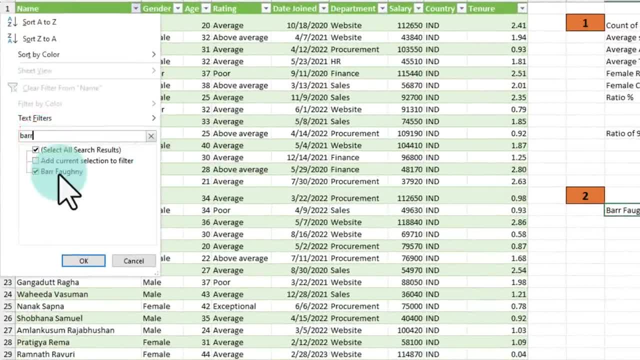 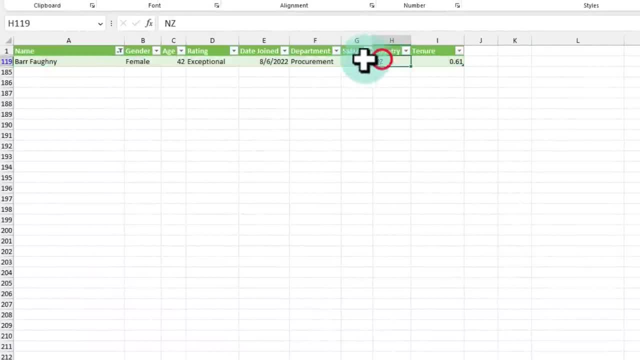 bar And you know we can see that the name shows up there and then click OK and then quickly see all the details about them. They work in New Zealand, $75,000 in the procurement department. They have been with us for 0.61 or less than one year. 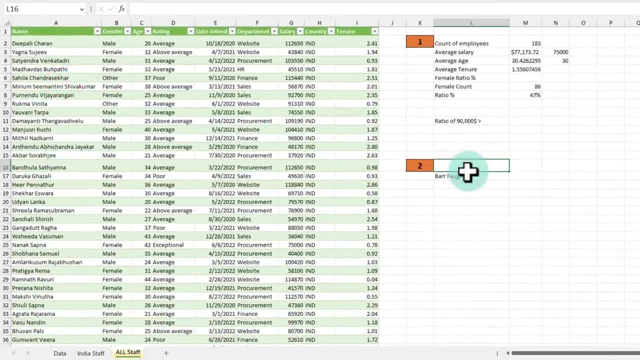 But that is quite manual And if the name changes you have to reapply the filters. So this is where we could use the lookup functions in Excel to do this kind of a job, And we are going to learn the basics of these lookup functions. 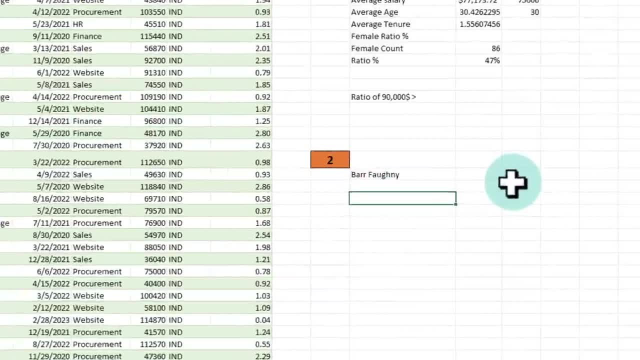 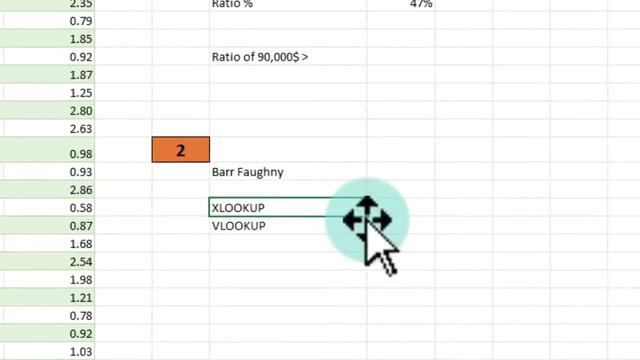 There are two kinds of lookup functions that we could use. We could use either XLOOKUP or XLOOKUP. If you have Excel 365, I highly recommend that you use the XLOOKUP function, But if you do have any other older version of Excel, use the VLOOKUP. 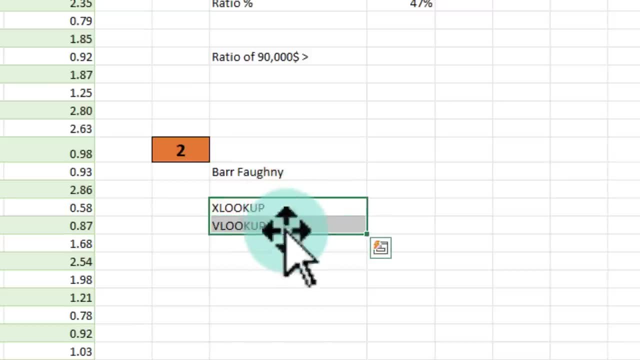 I'm going to build the formulas with both of them so that you're familiar with it, But later on we'll just stick to one of them, because it's that way it is simple and the video will move faster. So what we want to do is for the cell here. this is L17.. I'm just going to print some. 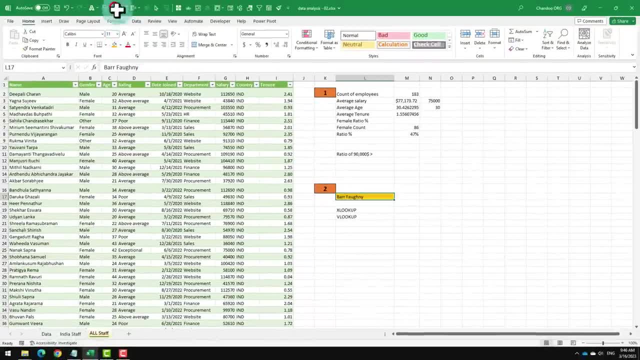 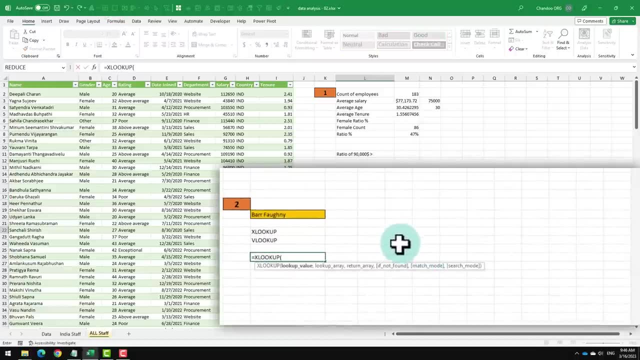 color there And for that cell we want to lookup and get their entire record here So we could use XLOOKUP like this: XLOOKUP lookup bar phony, so the L17. And then you need to specify the lookup array. Where is this name? It's in the staff table name column. And then what? 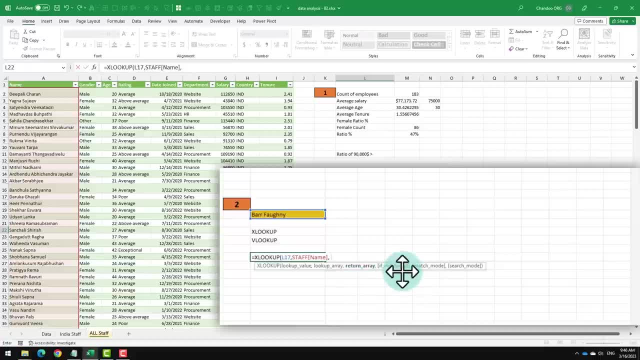 do we want? We want their entire record. What is their gender, age, rating, everything. So I'm going to say staff, staff table, and then we can say: from gender, colon tenure. So we want all of these columns for that person and then, when you close, you're going to get. 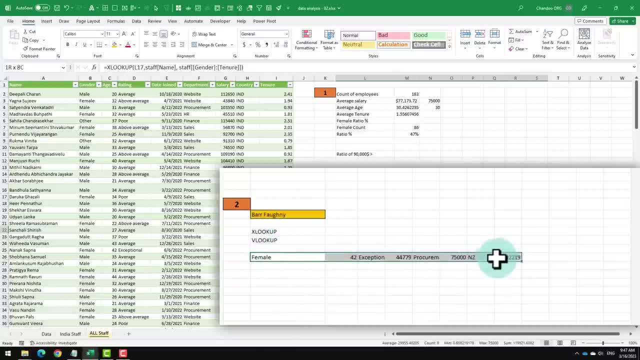 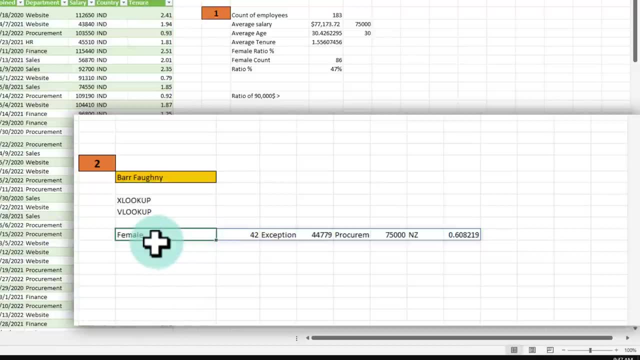 their entire record here for Barfony. this is their record because there are multiple values returned by XLOOKUP. it's going to spill the values in this direction because the data is also in the horizontal direction, so the XLOOKUP will also go in, like this many. 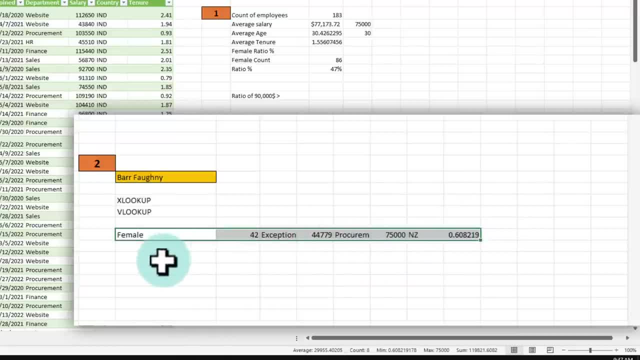 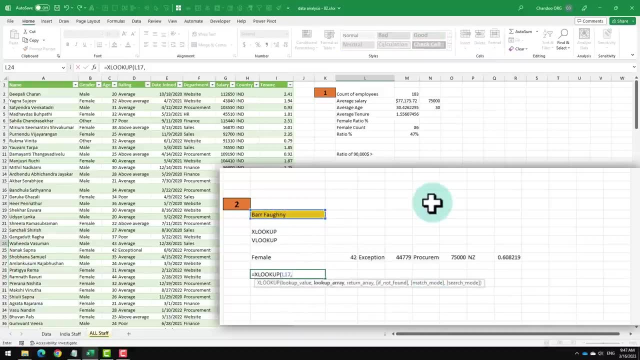 times. this format may not work. from a presentation perspective. you may want to see the results like this, so in that case, what we could do is we can say XLOOKUP Barfony in the staff name column and then return array instead of typing it. you can also select the. 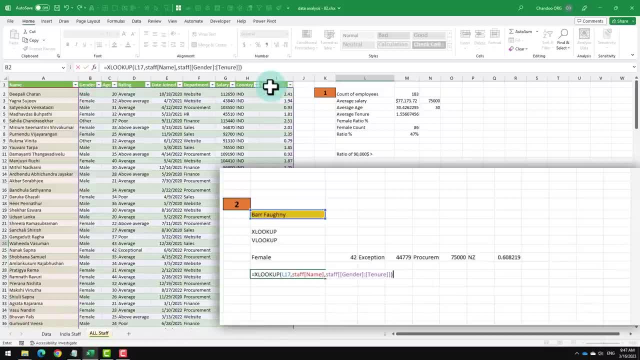 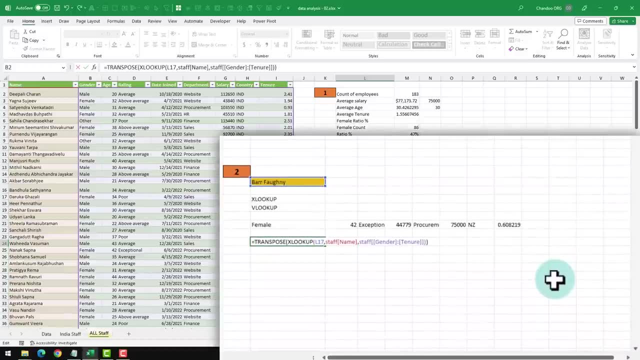 column. so I'm just going to select like that and then, instead of just doing XLOOKUP alone, we can use the transpose function around it so that it will be transposed, so the horizontal data becomes vertical and we will get a format like this. let's do a quick formatting for. 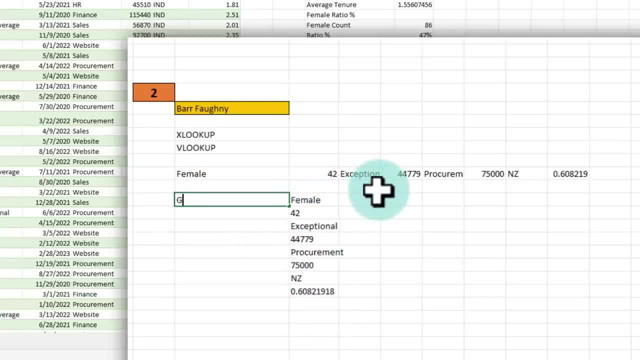 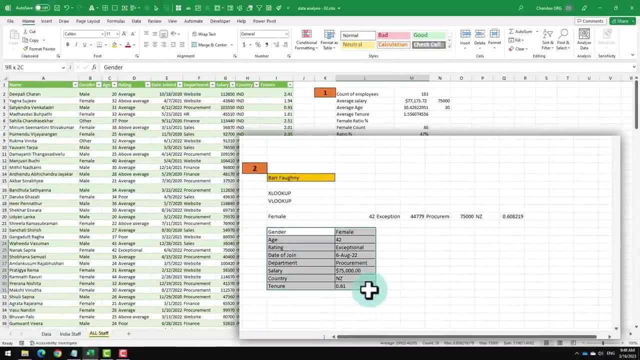 this. I'm just going to move this here and we will get the information for Barfony. The beautiful thing about this is it is all dynamic. so if I change this and I want to find, for example, Darukha Gajali, I just type that name. 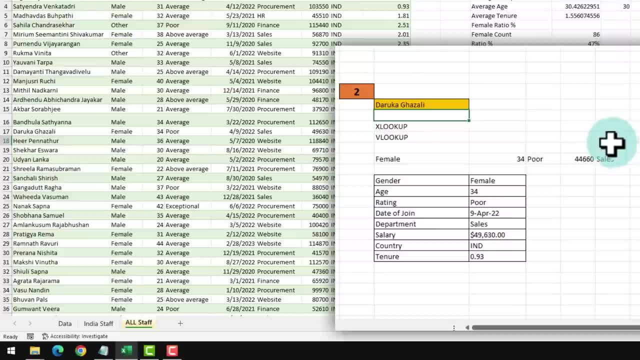 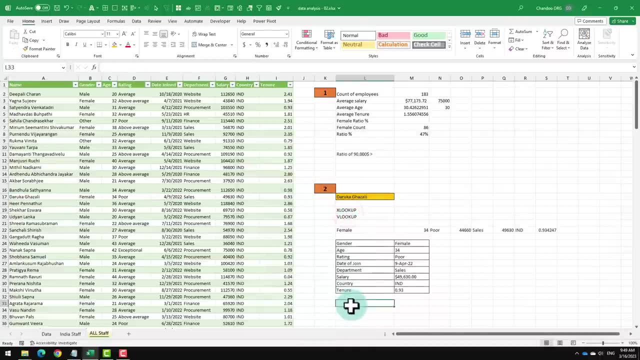 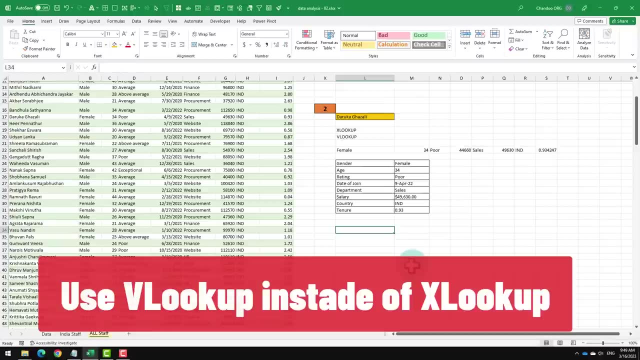 and then it I will get the information for such a person. here is that person. now let's see how to do the same with VLOOKUP. like I mentioned, my preference is to use XLOOKUP, but if you do not have XLOOKUP, then you can use the VLOOKUP, so we can say the same thing: VLOOKUP- look up. 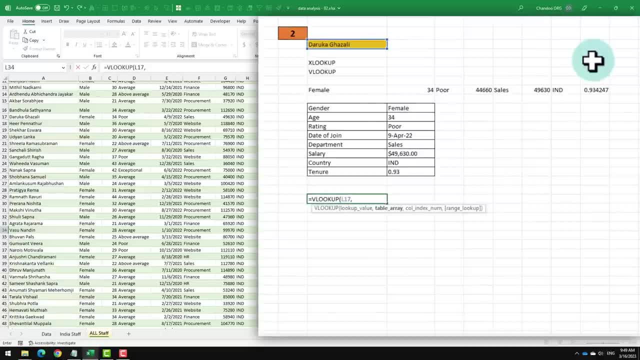 this name in this time you just say the whole table, so staff table. and then what is it that we want to return? now the lookup will happen on the left, most column, which is the name column. but return you have to specify which columns you want. so let's just say I want to look up their salary. salary will be one, two, three, four, five. 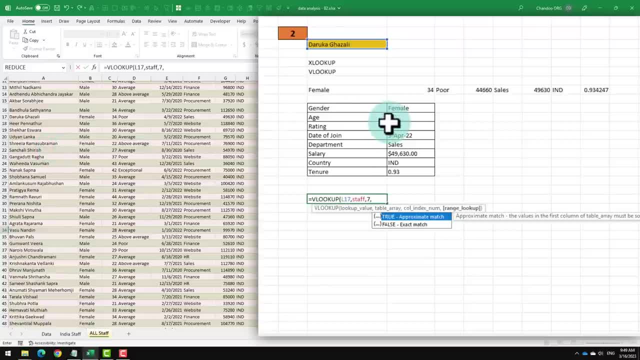 six, seventh column. so we're going to say seven, and then you have to also specify that you want an exact match. so this is where you will need to say false, and then you will get the salary for that person as forty nine thousand six thirty, same as here, if you do want to. 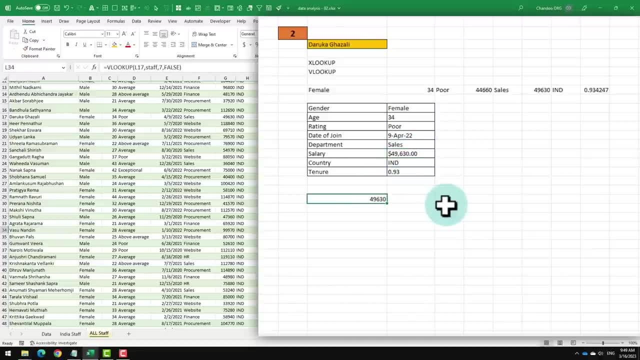 get all the columns Rather than just one column alone. you need to specify that as a list of numbers here, and then you need to do something else in older versions of Excel to be able to see the entire column list. this is also why I like XLOOKUP, because it's simpler formula. 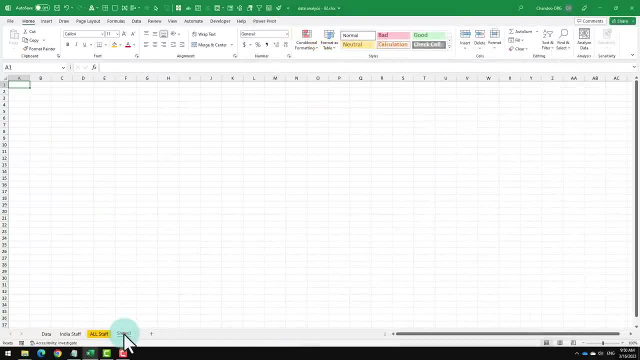 one formula gives me everything that I want. For our third one, we need to build an information finder version two. point. oh, this is where, if I provide a department name, I would like to see who is working in the department, what are their salaries, how old they are and few. 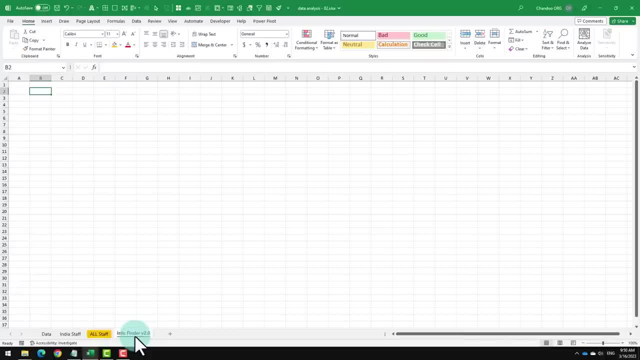 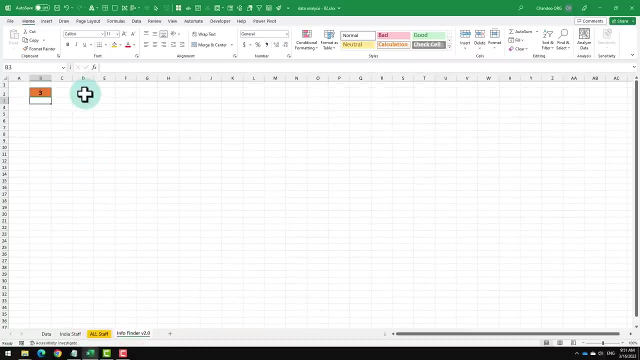 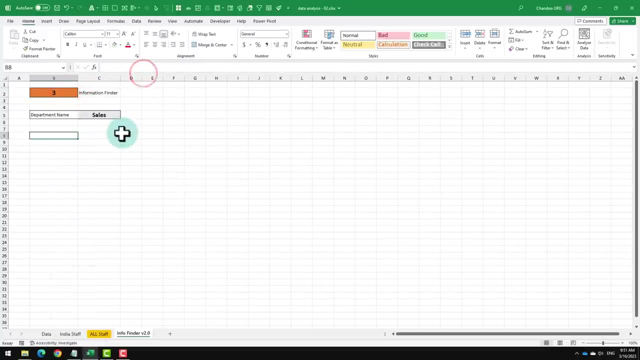 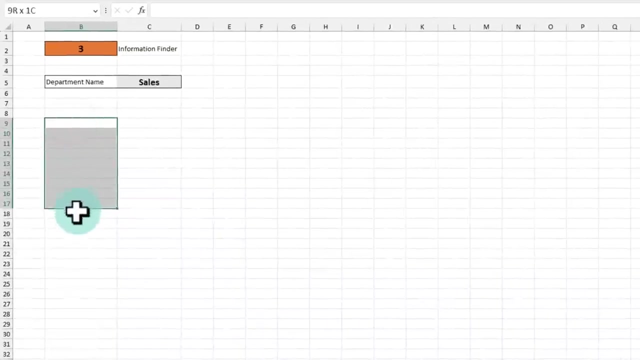 other details. we're going to do this in a separate tab. this way it's easier to work with this without getting confused with so many other details that are on the other page. So here, if I put a department name in this cell, C5- I would like to see who are the people. 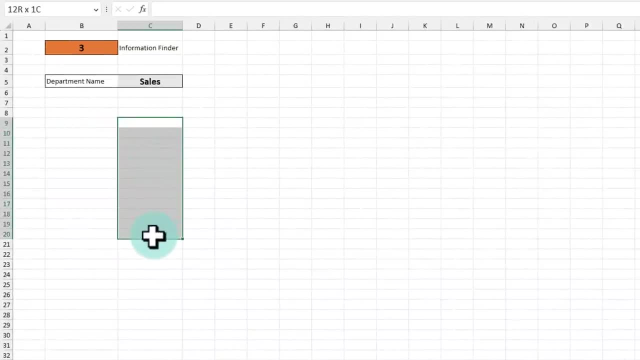 that are working in the department, what is their salary and what is their rating? just three columns. I don't want to see the whole history of them. I want to know the names, salaries and their employment rating information. Okay, and i would like this information to be sorted in the descending order of salary, so whoever is? 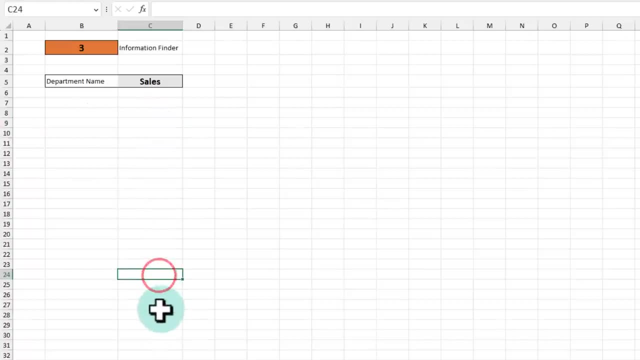 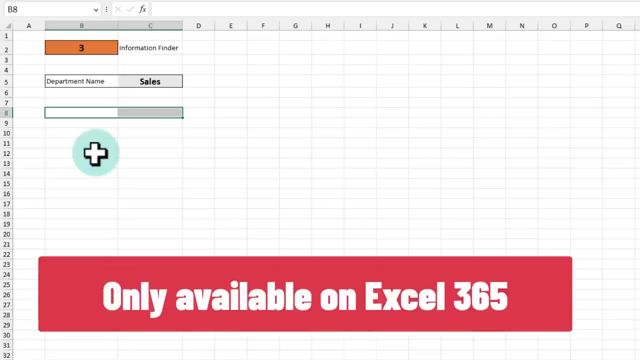 getting highest amount, they'll go on to the top and the lowest salary goes to the bottom. apart from that list, i also want to know up top. how many people are there? what is the head count of that department? sounds good, so to build this kind of a thing, we need to use new functions. 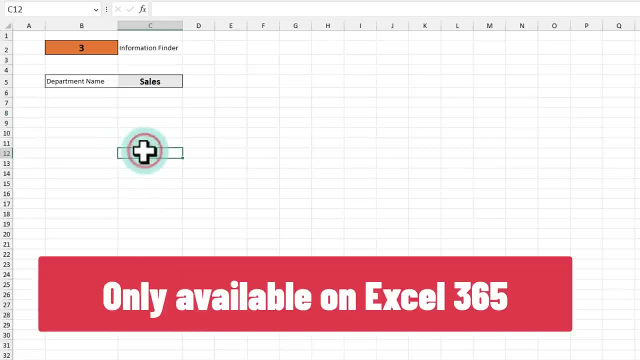 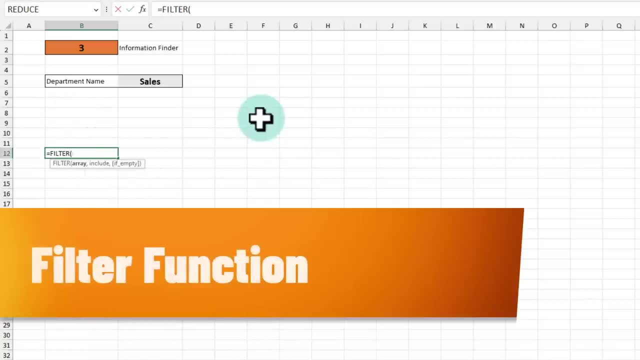 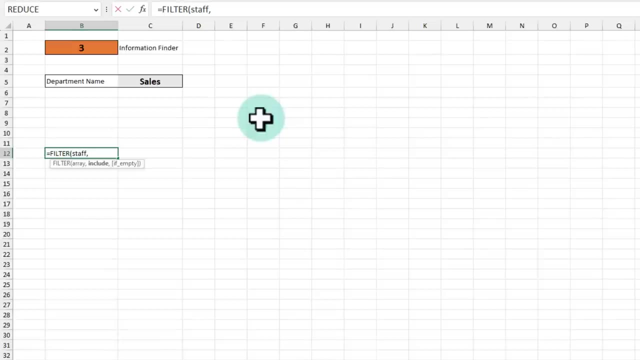 available in excel 365, so this part of the video will be very hard to follow if you're using a old version of excel. so here we can use the filter function: filter staff table. initially we'll just get everything. later on we'll figure out how to get only the required columns. so staff table. 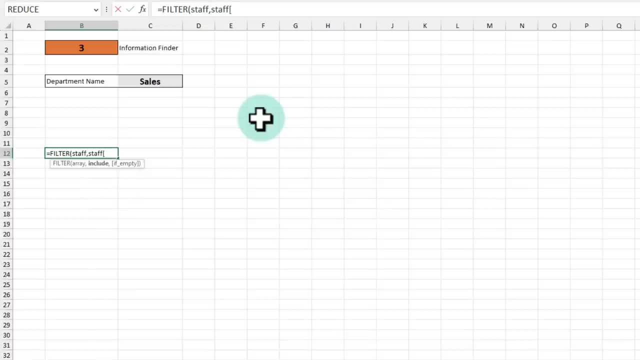 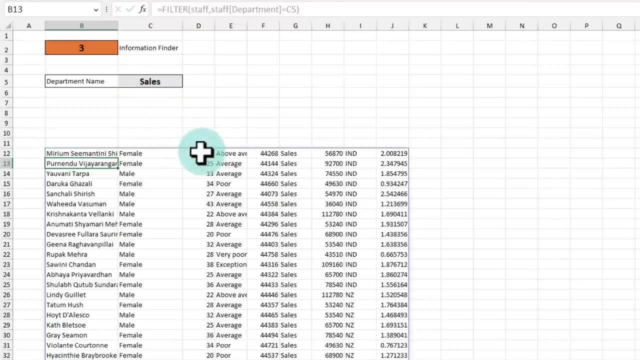 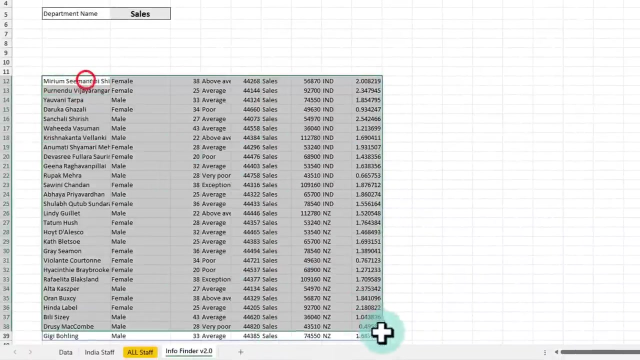 include by saying staff table department is equal to C5. If I say this, then this is going to take the staff table, filter it down to just the sales department and give me a list of all the employees in the sales department. You can see that everybody here is salesperson only. So this is the data. Like I said, we 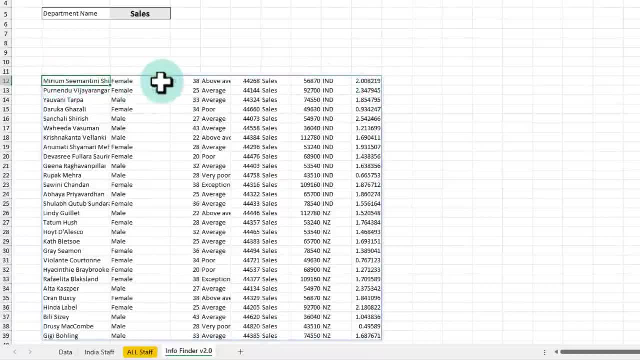 don't want all of this. What we want is name, salary and then the rating columns. So if I see put a number here, then essentially we want column one, column seven and column four of this data. So instead of just filtering, what we want is we want to choose the columns. 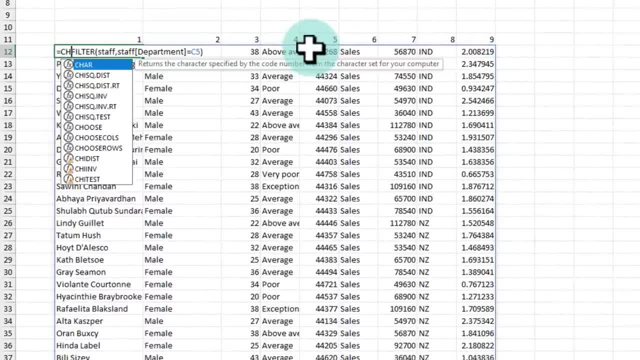 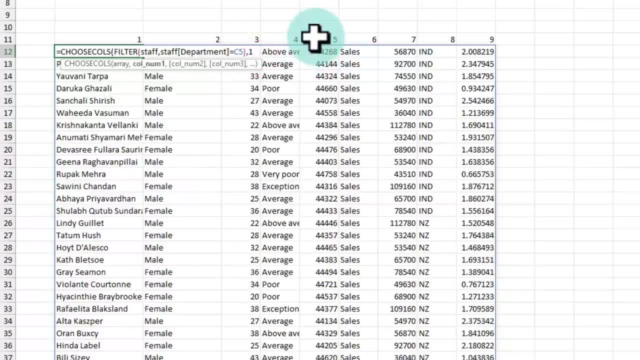 column one, seven and four. This is where a new function called choose columns comes into picture. choose columns from the filter result, And then we want column one, seven and four, in that order. So this is a different model. Besides this, we want to add the number of employees and 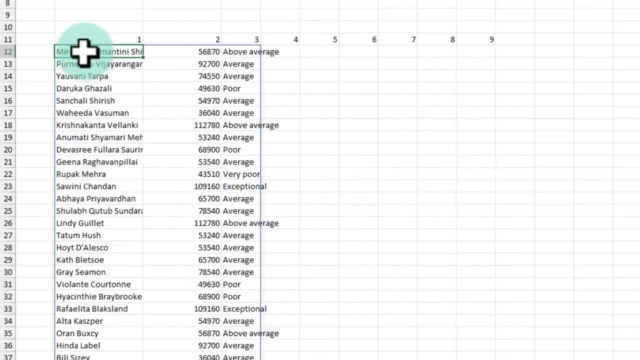 this is my target number, And now it's been created and I know that the number of employees, to just take out that entire thing, shrink it down to these three columns. rearrange them in this order. once this data is there, then what we want is we want to sort this by the salary column, so that 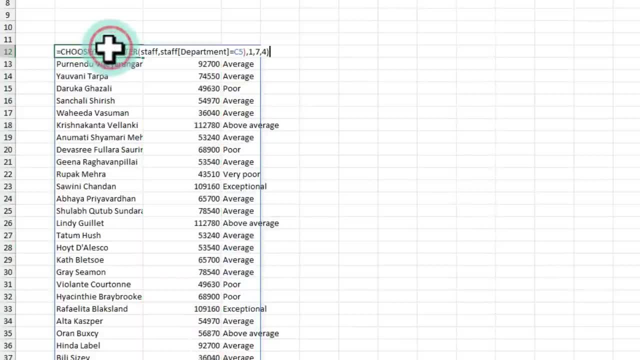 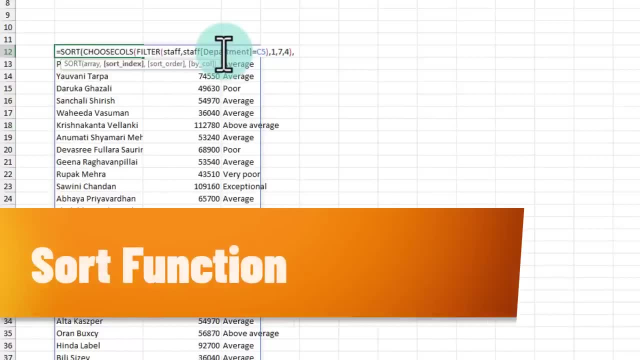 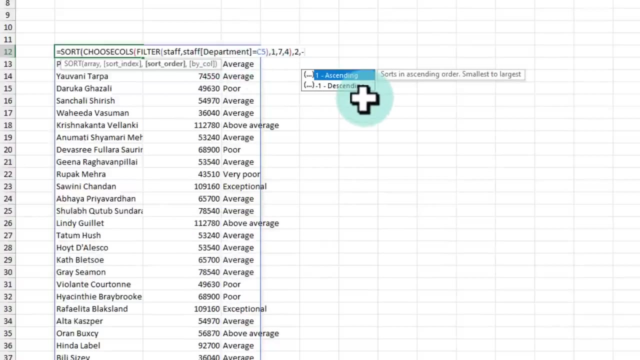 the highest salaries goes to the top. for this. we can then send this output to the sort function, so sort this entire thing by the second column. second column has my salary in the descending order. descending order stands for minus one here, so like that, and then we will get the information. 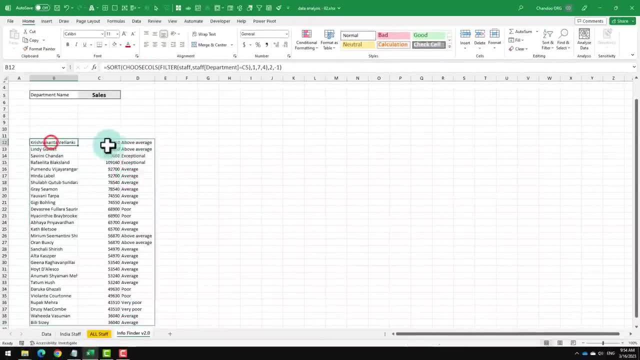 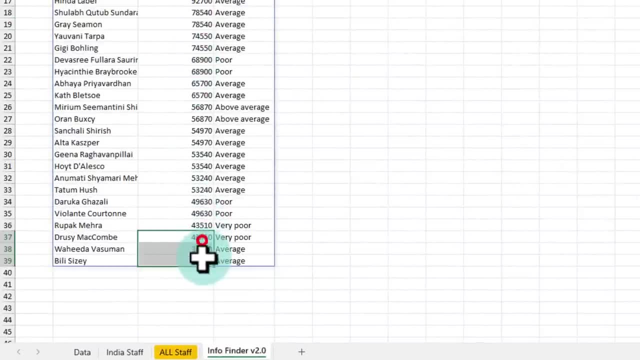 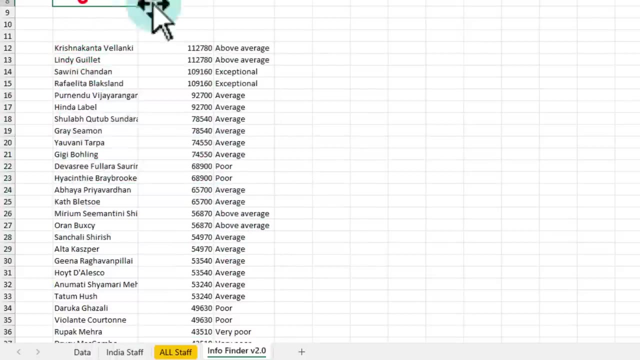 so these are our sales people names, salaries and their rating. quite a few people are making more than hundred thousand there, but we also have some people that are at thirty thousand forty thousands next up. we would like to count how many such people are there so you can say number of people. 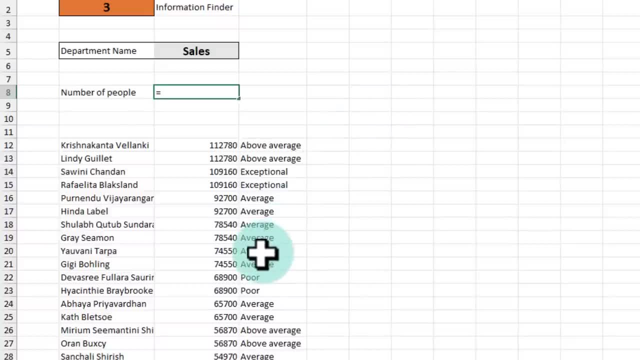 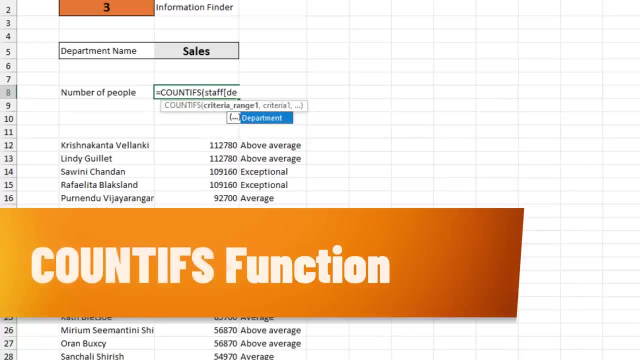 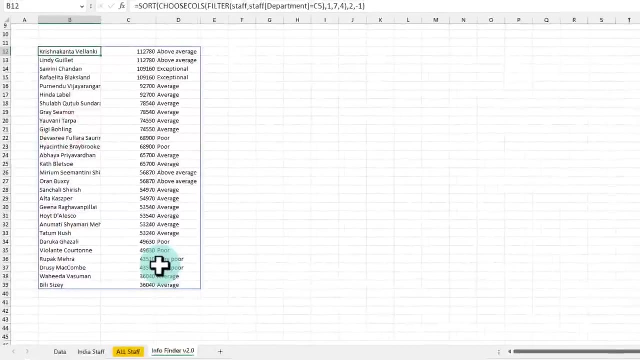 and then we can either directly refer to this or we could do something else. so i'm going to use our good old count ifs function count. ifs staff department is c5, so we have 28 people and these are the 28 people and this is all dynamic. so if i put something else like website here, i'm going 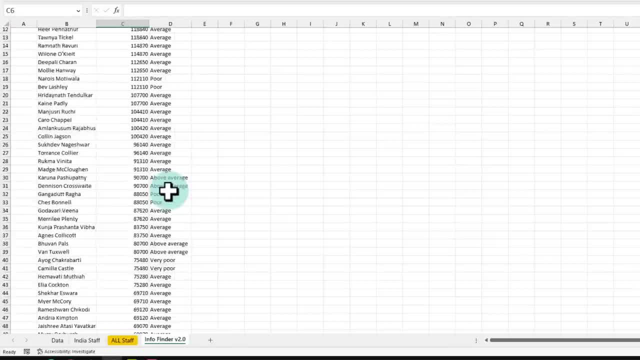 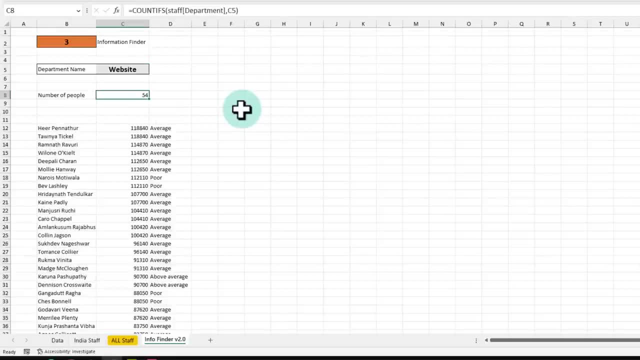 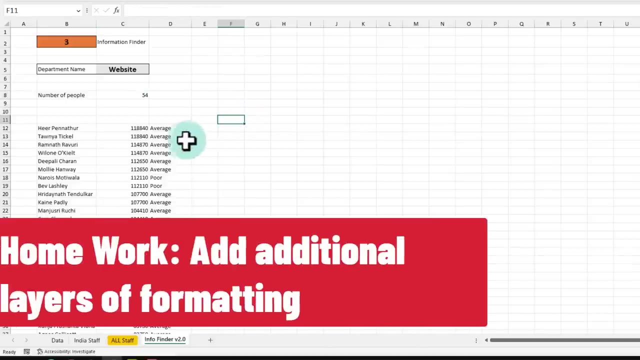 to get the website people neatly arranged in the descending order here underneath and all the 54 people, and this is the head count there. so that is our information finder version 2.0. if you want, you can add some additional layers of formatting or other things on top of this. i leave all of that for your imagination and homework. 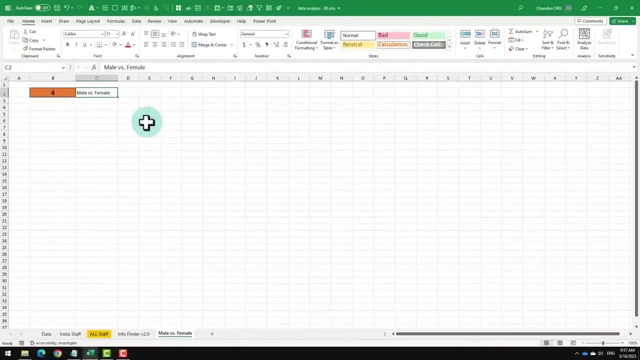 for our next question, we would like to do a quick male versus female comparison and understand the how many people are there by each of these gender groups. what is their average age or average salary or some of the other stuff? we could again use formulas to do this, but we have already used. 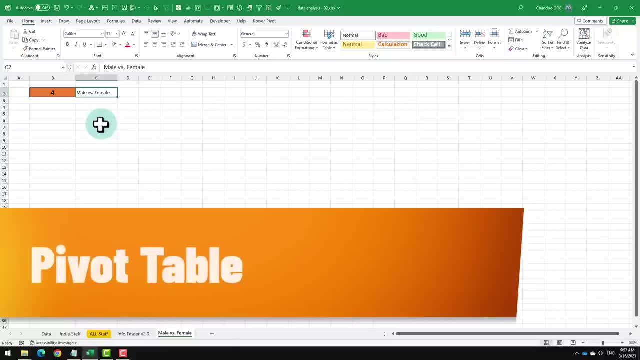 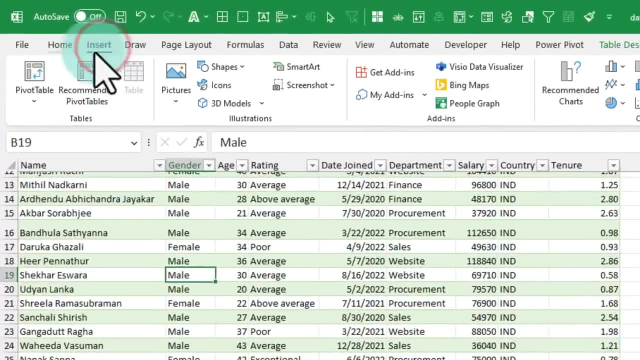 in a formulas. so i'm going to introduce the pivot table approach to do this analysis. we can go to the data set here, select any cell and then use the insert pivot table option to introduce a pivot table to do this analysis. so i'll tap on this. 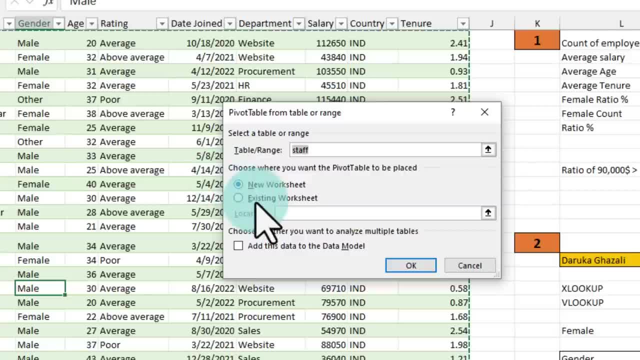 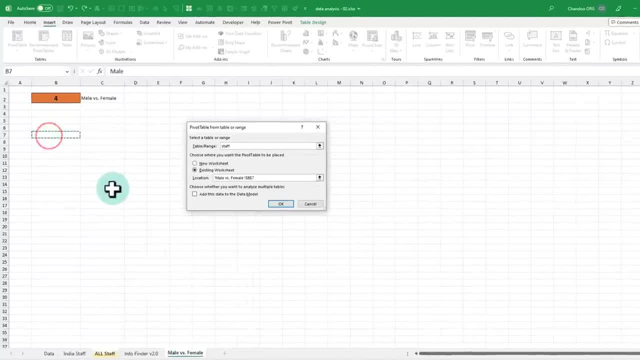 and you can straight away go and do a new worksheet or pick an existing worksheet, since i already have an existing thing set up. i'm going to select male versus female and put the pivot table here. one additional thing that you may want to do, and i personally like to do this every time. 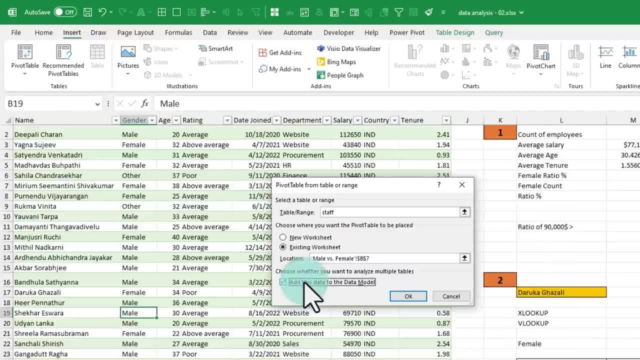 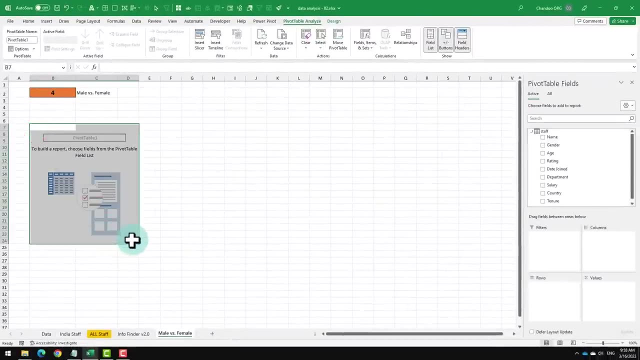 is: add this data to the data model option. what this does is it enables some special features in your pivot tables so that you could answer some very interesting questions quickly as well. let's click ok and we will get a canvas here for you to build a pivot table. 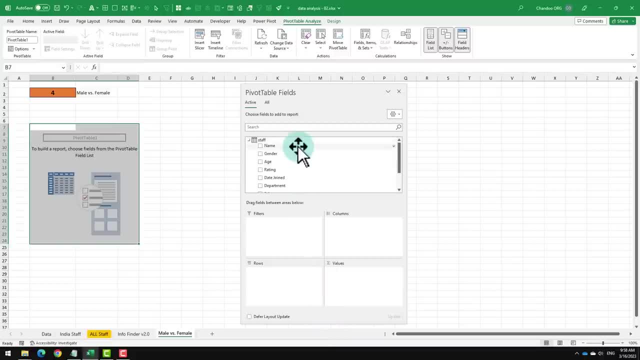 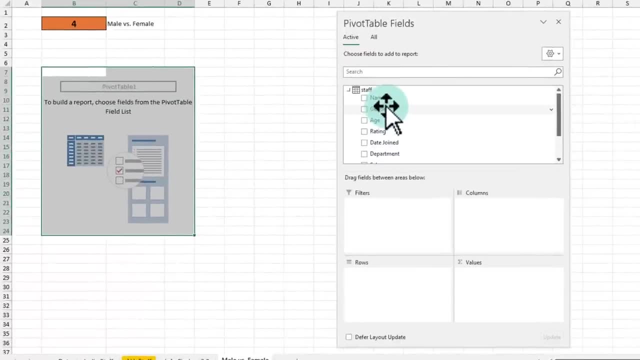 you will also have this pivot table fields option here, using which you can construct the pivot table. if you have never built a pivot table in excel, think of this like a quick and easy reporting system built into excel. we can use pivot tables to answer many business questions or build reports. 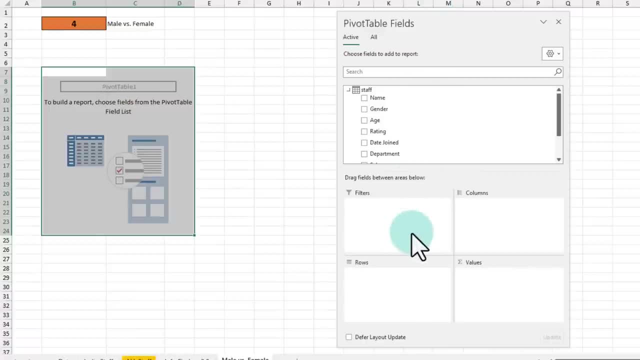 quickly from your pivot table. let's click ok and we will get a canvas here for you to build a pivot table data. i do have many other videos on the channel that go in depth into pivot tables, so here i'll build the pivot table and hopefully it all makes sense if you have already been using pivot tables. 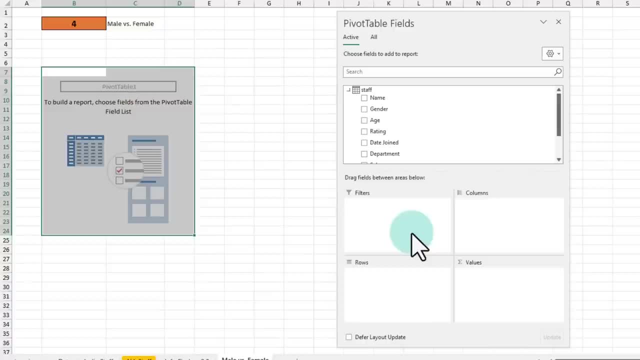 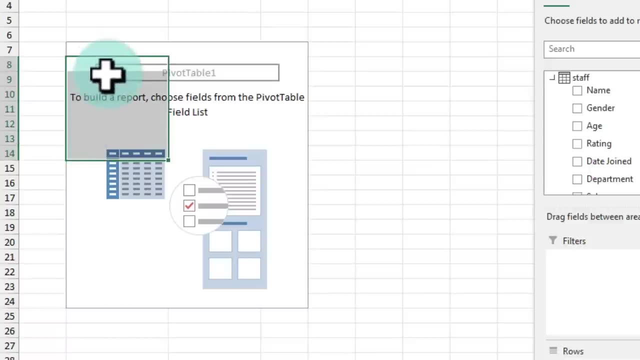 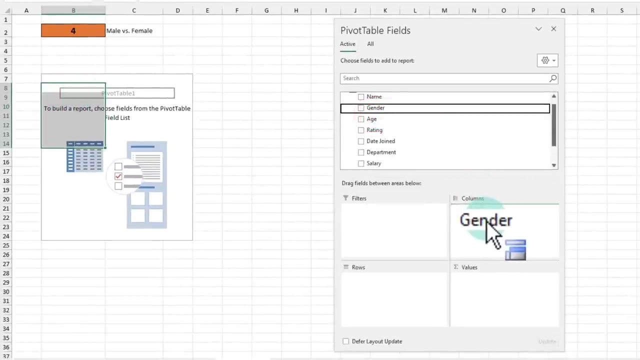 for some other purpose, then it all will make sense anyway. so here, what we want is we want two columns, one for male, one for female, and then we would like to see how many people are there, what is their average age, etc. so i'm going to take the gender and put it into columns, because we want one gender. 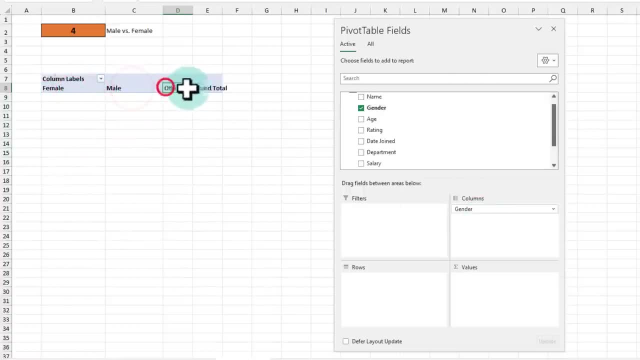 per column. so this will have female, male and other, as well as grand total. we'll worry about what to do with this other gender and grand total a little later, but for now, what we want next is we want to see how many people are there. it could be a count on the name column, so i'm going to take the name. 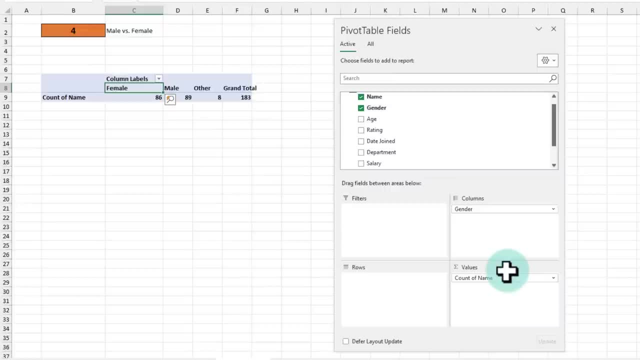 and drop it into the values and it's just going to count the name. so we have 85 females, 89 males, etc. you might already remember that number 86 from the earlier portion where we calculated the female percentage. next up we'll take the age and put it into the values again. 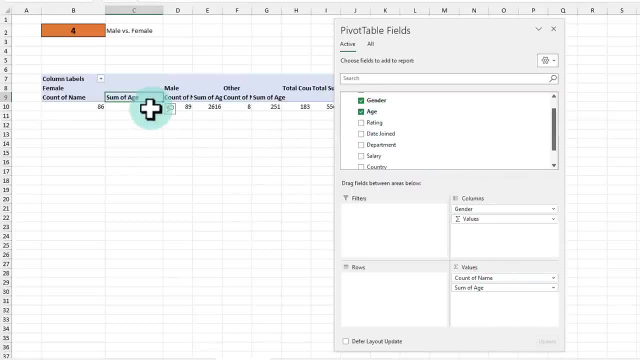 by default because age is a number. excel is going to sum up the age. so sum of all female employees age is 2701 and all female employees age is 2616. this number is useless, so i'm gonna right click on the number and change the summary from sum to average. 31 is the average female age. 29. 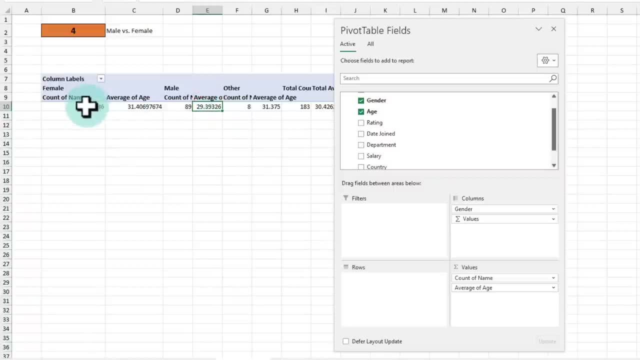 is the average male age. next, you can see that this pivot table is kind of growing horizontally. what we want is counts in one row, averages in next row, like that. so we'll take this values option here, click on it, drag and drop it into rows so that you will pivot table gets restructured. 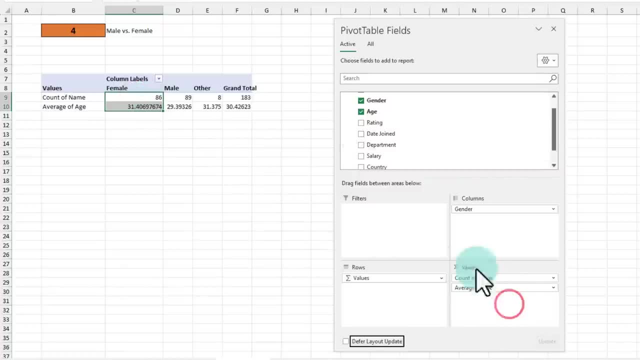 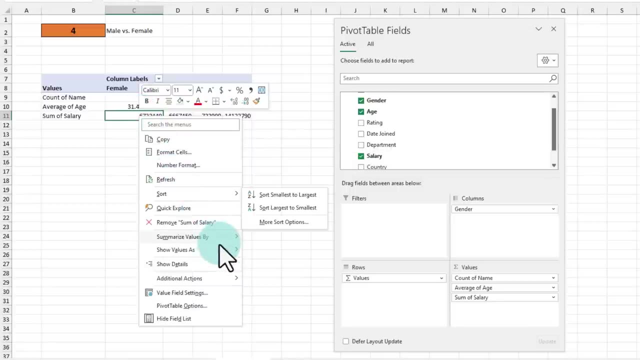 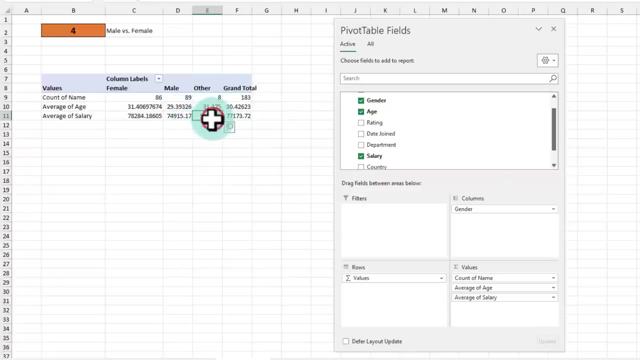 like this. this looks better. next up, we are going to take salary and put that into this again. it sums up the salary. right click on it and then say summarize by average so we can see what is the average female salary, male salary and other gender salaries. we could do the same. 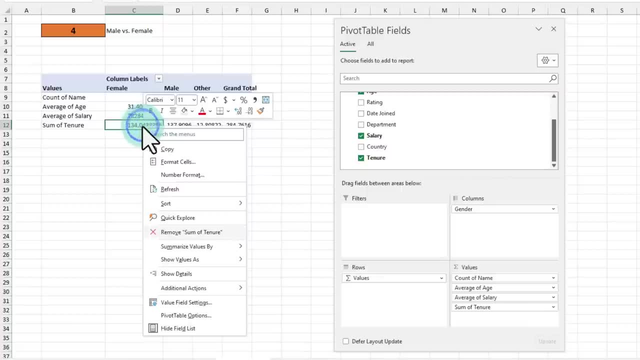 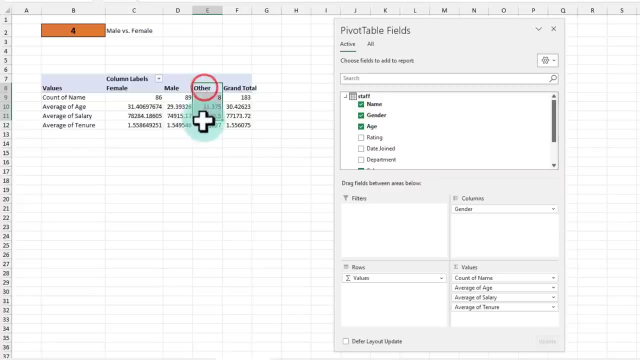 for tenure. and now that the information that we want is there, let's see how to take out these other gender so that we can just look at male versus female. so for this purpose, because we only have few people with other gender, that kind of skews the analysis. so 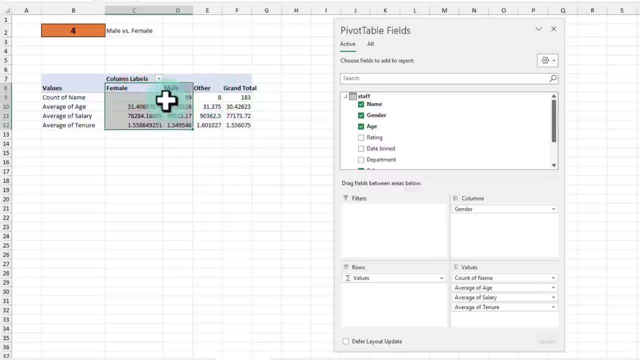 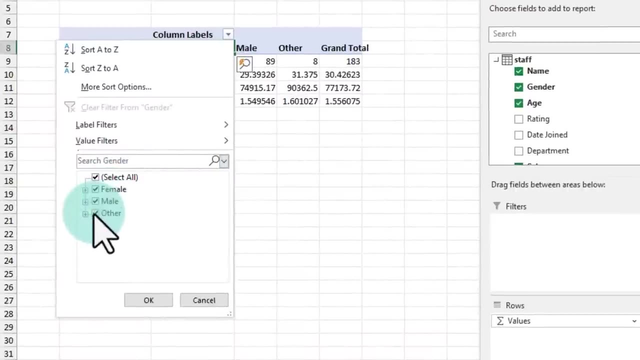 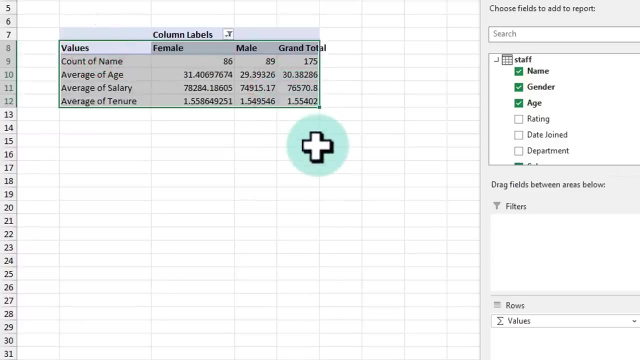 it's better to focus on the two larger groups when you are doing these kind of comparisons. to do that, you can click on the column labels arrow and then uncheck the other option and click ok. so this is how the information looks across the countries, both countries, let's. 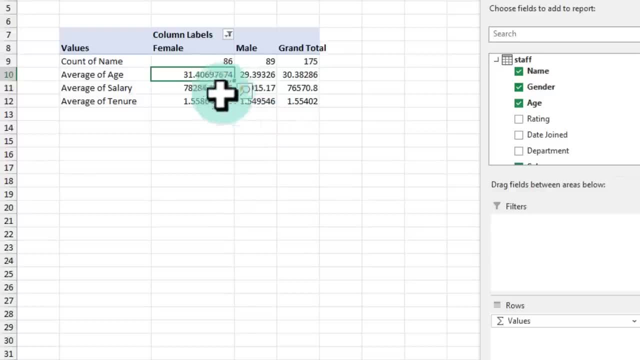 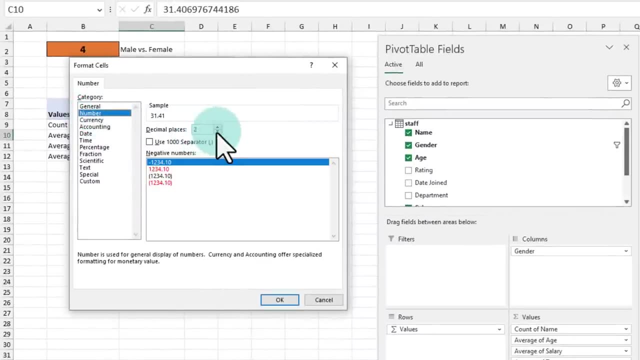 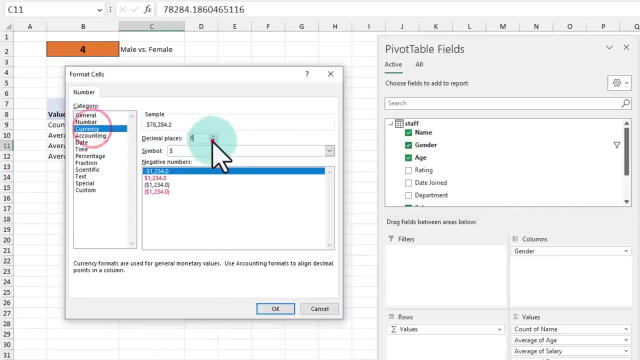 apply some quick formatting. to format the values in the pivot table, you can right click on the number and then use the number format option and select the appropriate format that you want. click ok. if you don't want to see the grand total, you can also go to the pivot table design. 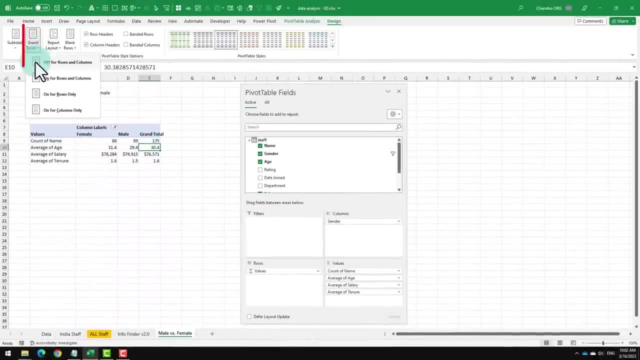 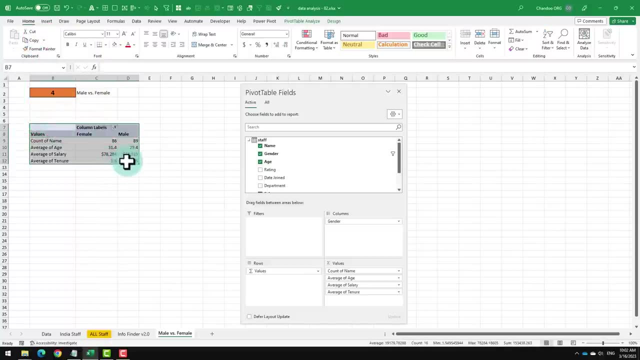 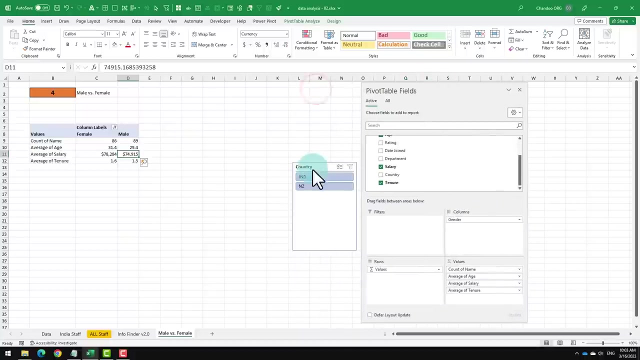 ribbon and then from here, grand total and you can turn that off. ok, as i mentioned, this is the information for both countries. let's say, i want this, but only for new zealand. what we can also do is right click on the country option here and then add it as a slicer. this will give you a slicer which will give you two buttons for. 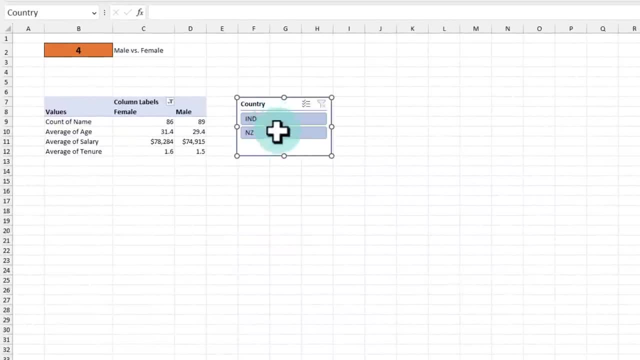 one for each country, and these are interactive. so if i tap on new zealand i'll see the next country section is generated and then if i go to the next country section i can give a type that says country menu. so this is the information that is provided to me here in. 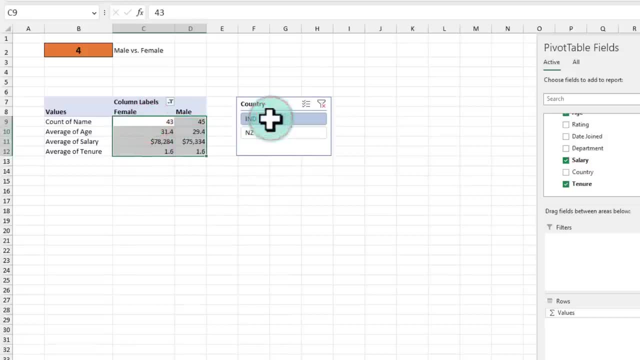 numbers for New Zealand alone. If I tap on India, I'll see the numbers for India. So this gives me a quick sense of how our staff are in both countries. With slicer we get to see one country at a time or if you want to see both, you can clear the filter and then select both of them. 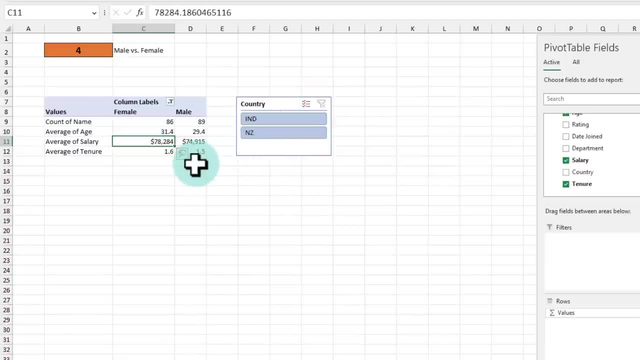 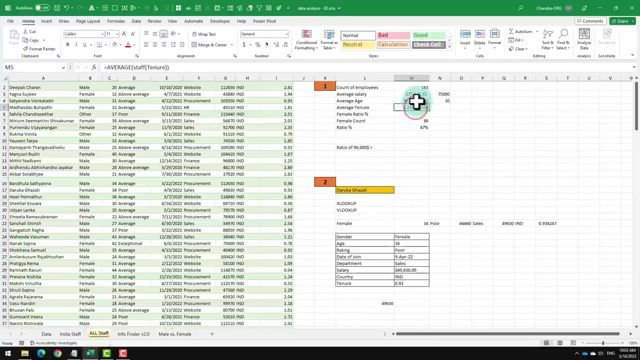 to see how it is happening. Together with slicers, pivot tables become so much more easy to work with and answer any kind of question without writing complex formulas. Imagine, to get these kind of numbers earlier we had to write some not so complex but still complex formulas. So this is 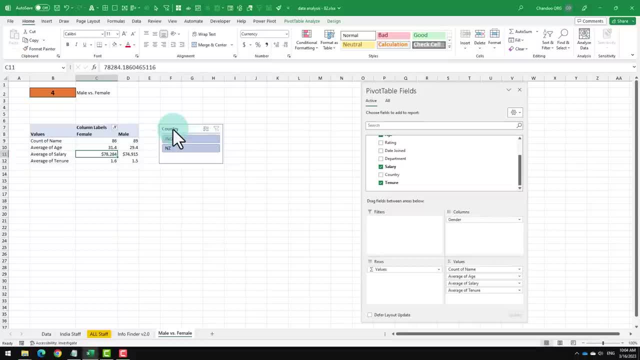 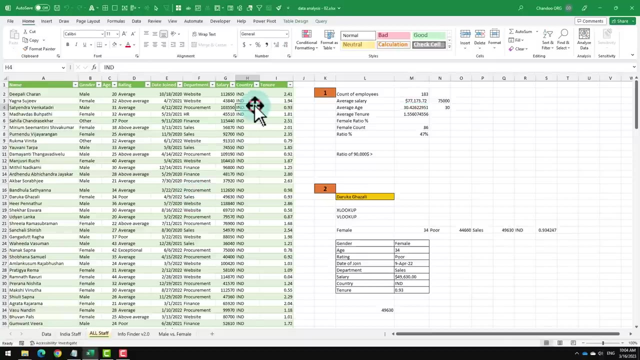 why I do like pivot tables to do some of the ad hoc analysis. That said, I like the flexibility of Excel functions because that lets me build more complex answers or control things in a better way as well. Now let's go back to our data, and our last thing is to do a bonus calculation. The bonus: 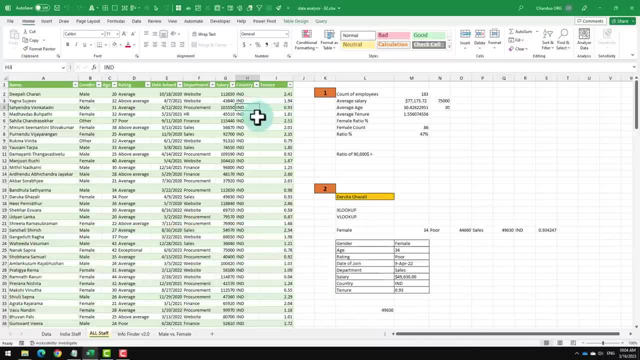 calculation is really simple. We would like to give 3% bonus on salary. So whatever is your salary, your bonus would be 3% of that, assuming you have been with the organization for at least 2 years. If not, your bonus would be 2%. So it's a simple rule at Awesome Chocolates. Have you been with us? 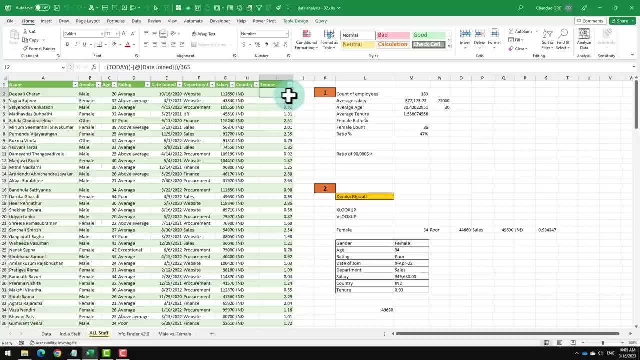 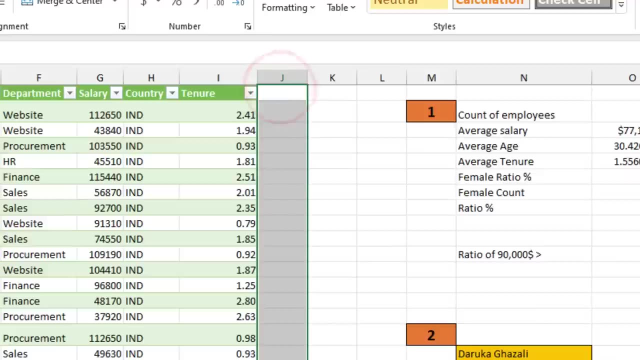 for longer than 2 years. Then you get 3%, else you get 2%. We can calculate the bonus as a new column here, because everything is touching each other. I'm going to introduce some columns here so that there is a little bit more room for our table and we can calculate the bonus as an extra column now. 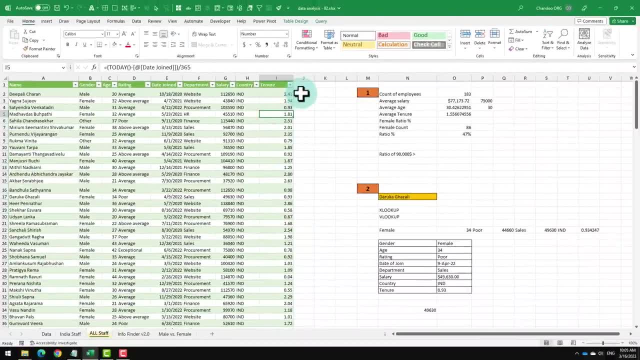 You can do it in two places. You can add a column to your table or, if you're comfortable with Power Query, you can also do this as a step in Power Query too. I'm not going to show you the Power Query option right now, but that is something that you can try. 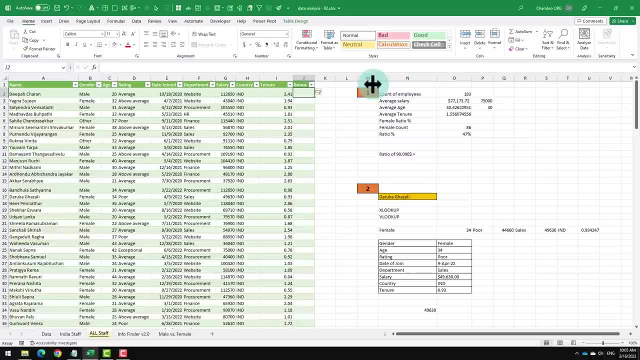 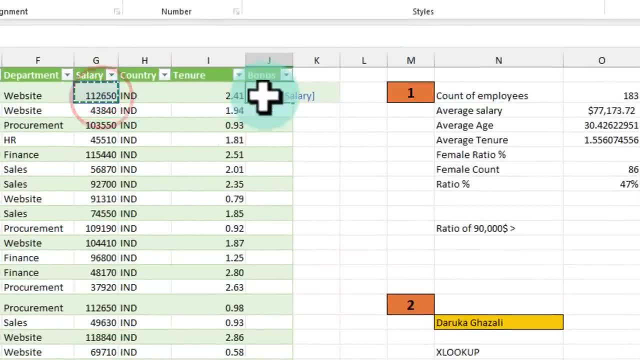 yourself. So let's do the bonus percentage here. Bonus calculation: Like I said, bonus would be 3% of salary, but it can't just be 3%. It would be 3% only if your tenure is more than 2 years. 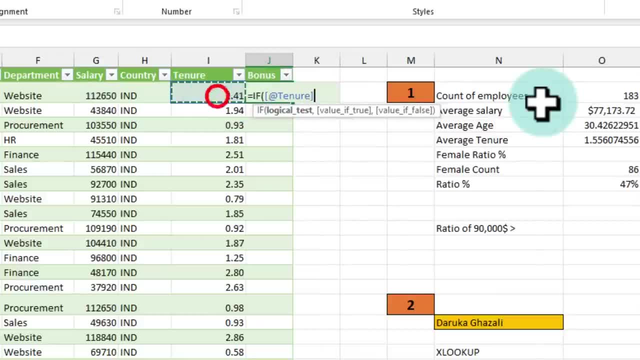 So this is where we could use the IF function. If my tenure is greater than 2, because tenure is already in years, then I can do a bonus calculation. If I do a bonus calculation, then I can do a bonus calculation. We just say 2, then it needs to be 3%, else this will be 2%. 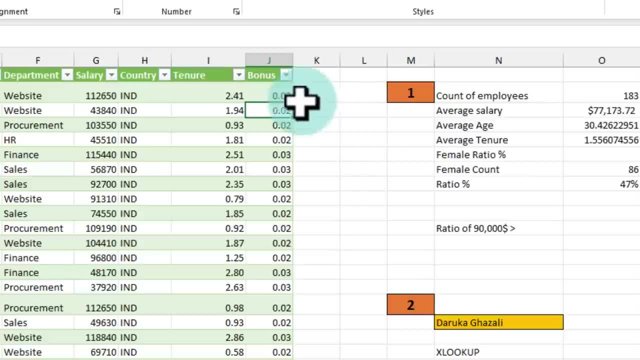 So this IF formula tells me what the percentage is. This is not enough. We need to now take that percentage, multiply that with the salary, and then that will give me the bonus value. If you want, you can round this bonus, So I'm going to round it up to the nearest number. 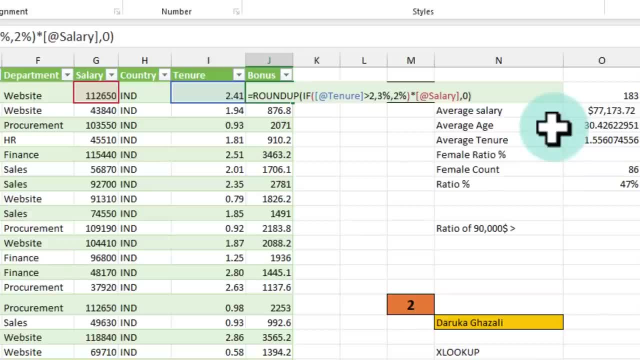 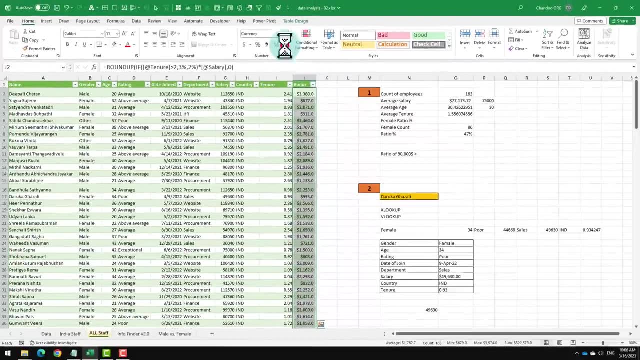 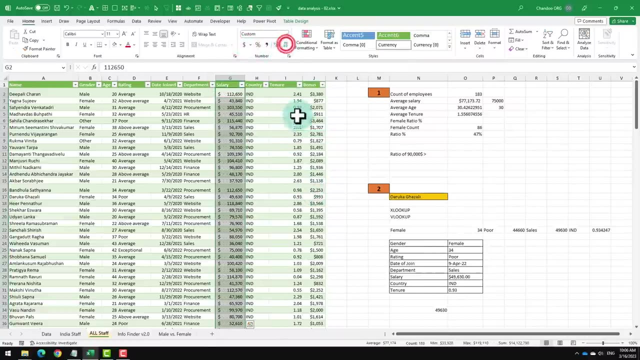 So round it up to zero means no more decimal points. just take it up to the next highest number and then that will give you the bonus. Let's apply some currency formatting on this little thing and we will get the bonus values. Let's say, as you are looking at this, your boss suddenly comes up and then says: 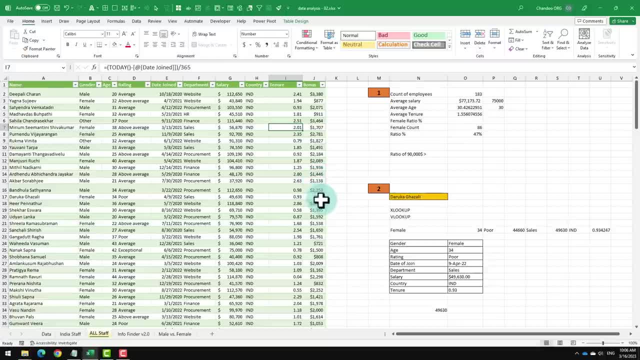 oh, you calculated the bonus, Good job. Can you tell me who are the employees that are getting the highest bonuses? I just want to know the top 10 names. You can do lots of the different things. You could write a formula, you could do a private table and all sorts of things. 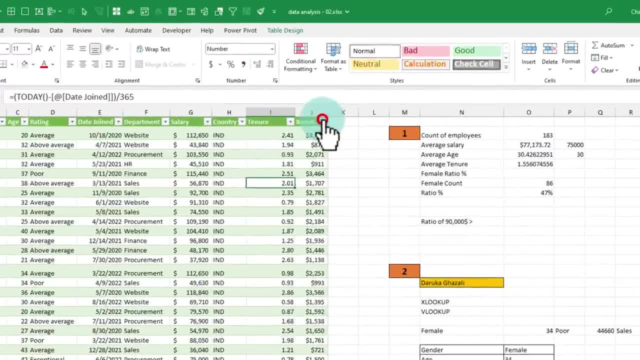 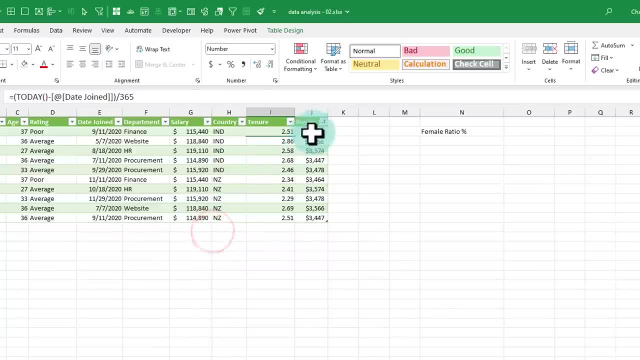 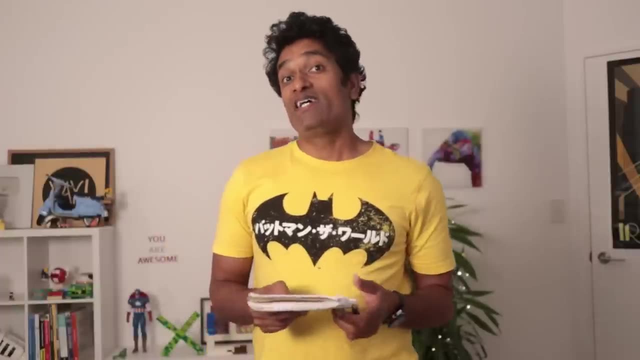 but I'll show you the quickest way to get there. Click on that little arrow number filters and then select top 10, just click Okay And you will see the top 10 employees making highest. All right, So now that we have answered those business questions. 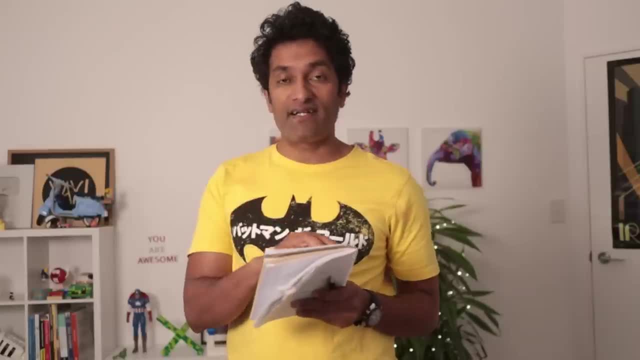 let's understand how to use charts and other data visualization options in a business So you can use them over and over and over And you can be pretty freshened up by this business solutions capacity: It 검 cars. you see, when you type on this in here, Now put it for that and keep it in and start consuming. So let's find a number from the top 10 and then turn it on number 10.. 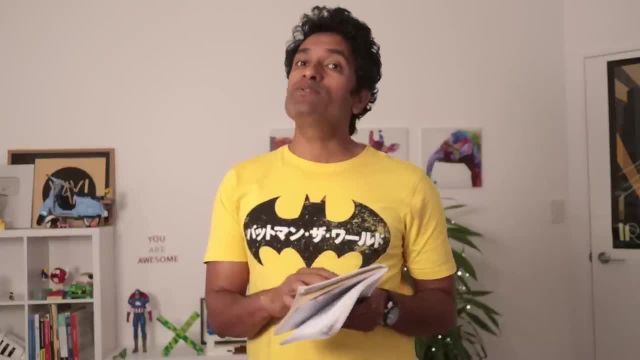 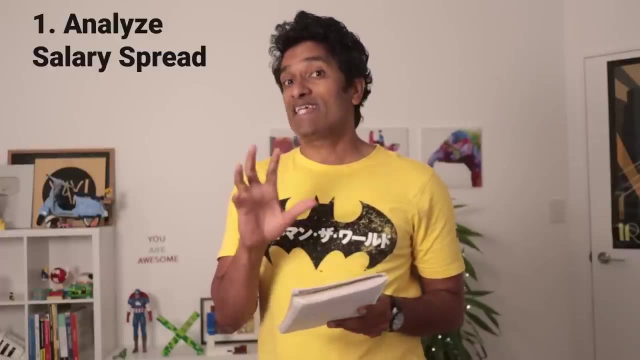 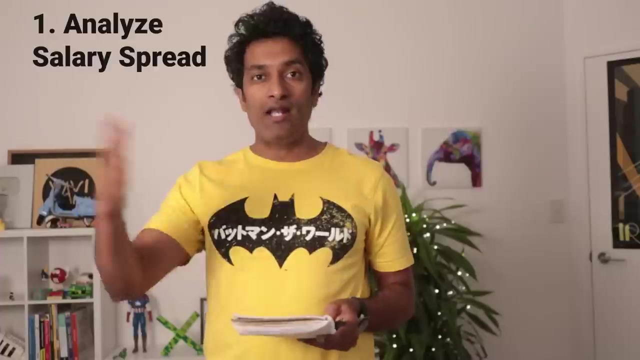 data visualization options in excel to do some data analysis. i have got four topics for you in this section, so we are going to look at the salary spread to begin with, how the salaries are spread, what the distribution looks like. are there some extreme values or not? so that is the first topic. 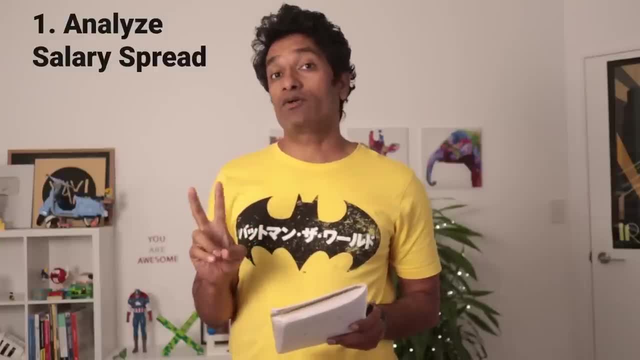 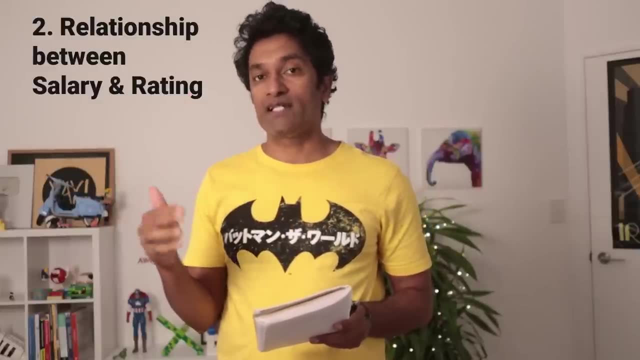 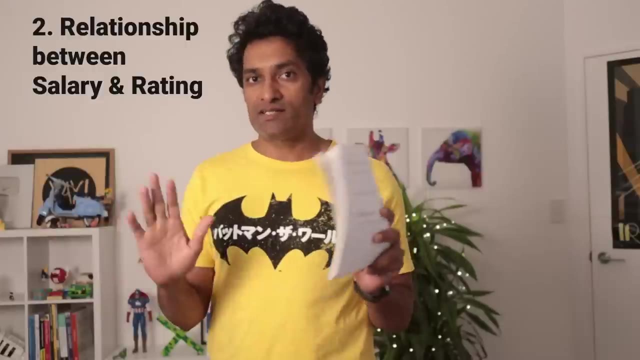 for our data analysis. and then the second question that i would like to answer is: is there any relationship between salary and employee rating? for example, are the exceptional people getting paid more or are the poor people getting paid less? you know that is. is that something that exists? 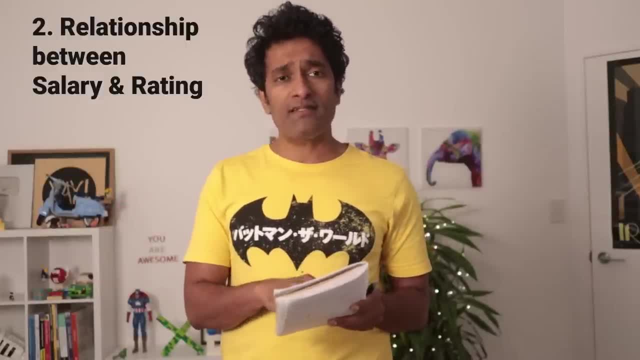 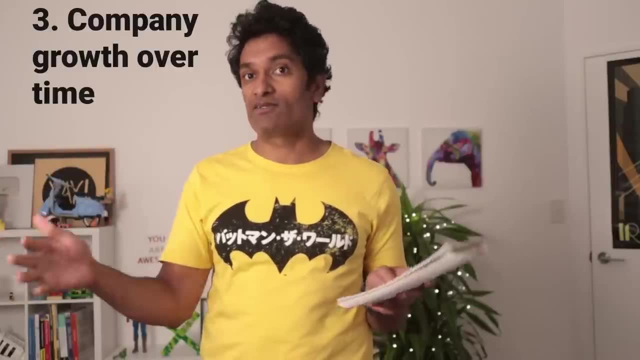 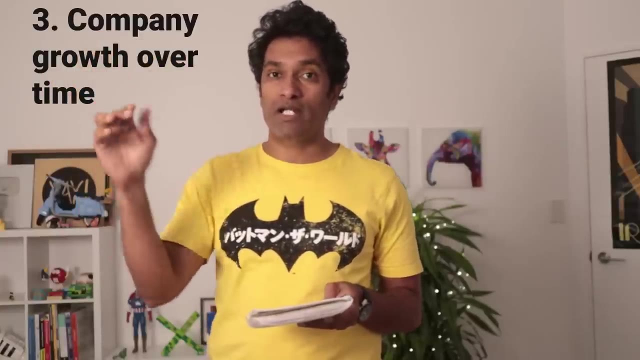 within our organization or not? and then the third one is: how did our company group, from the very first employee up until the 186 or 83 employees that we have now? what was the trajectory like? how was the our headcount over a period of time? where is it heading, you know? can we tell anything about the future based on that? 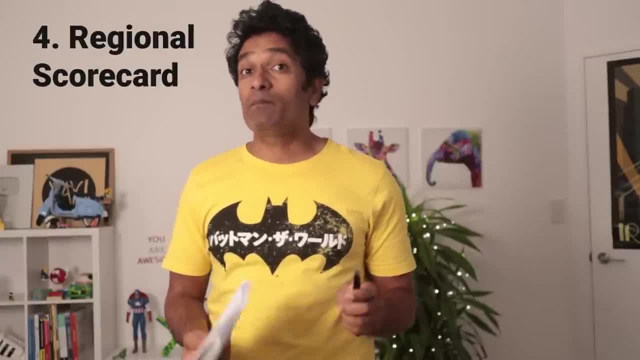 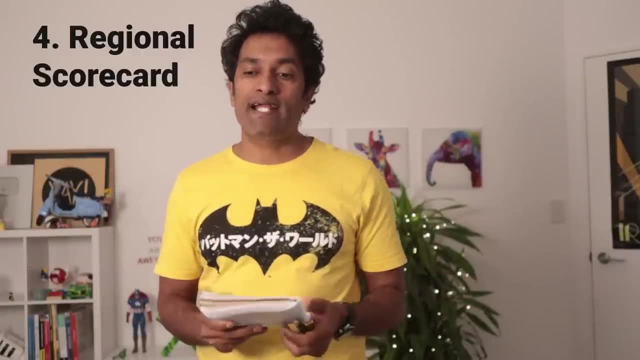 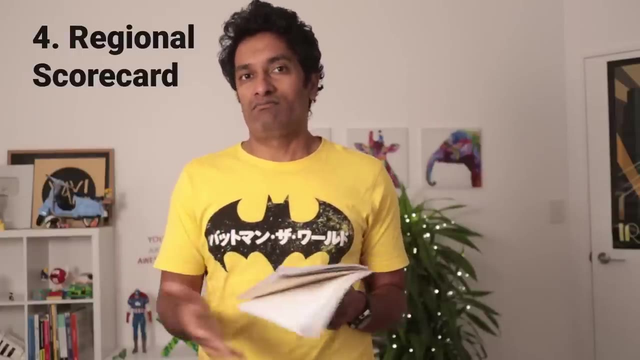 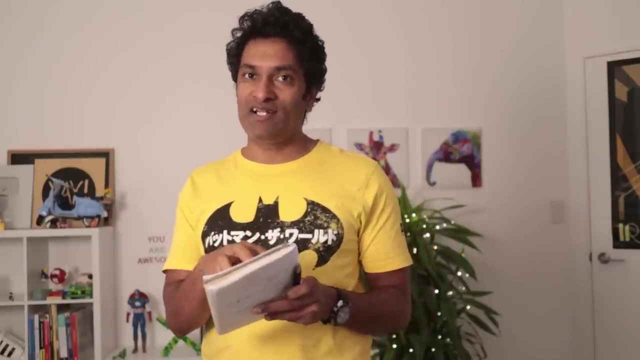 information. and then, finally, i would like to prepare a india versus new zealand report card so that we could compare both countries and understand various key statistics and business metrics from the hr perspective. and you know, make it fun. so that is the scope of this part of the video. uh, again, we are going to introduce some very fun. 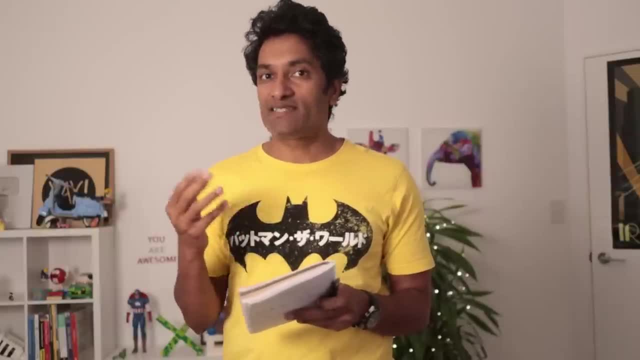 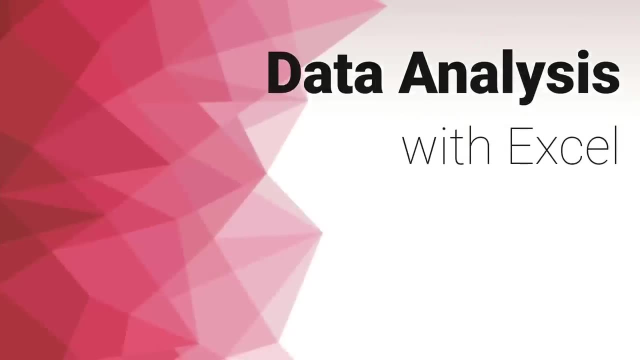 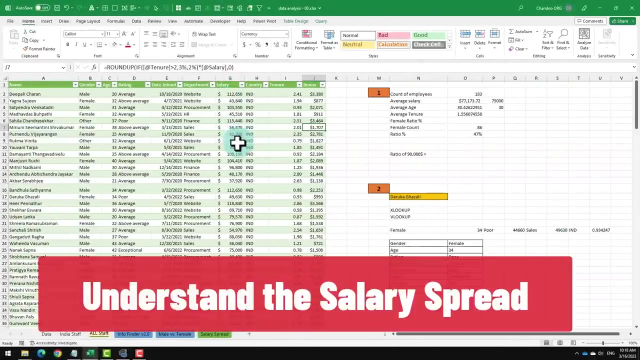 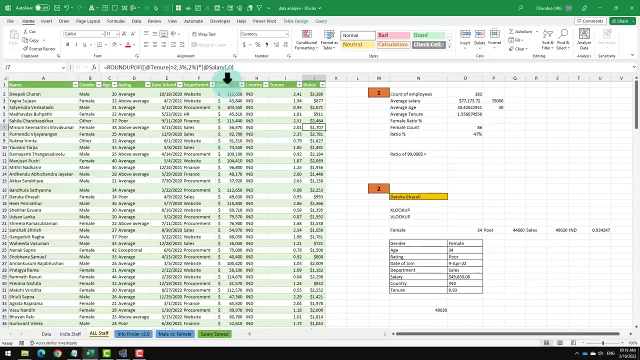 and useful chart options in excel, as well as conditional formatting and data validation. let's go so. our first topic in data analysis section is understand the salary spread, and you could do this in few different ways. so if you want to do it quick and dirty, here is how i would do it: just select the salary column and from 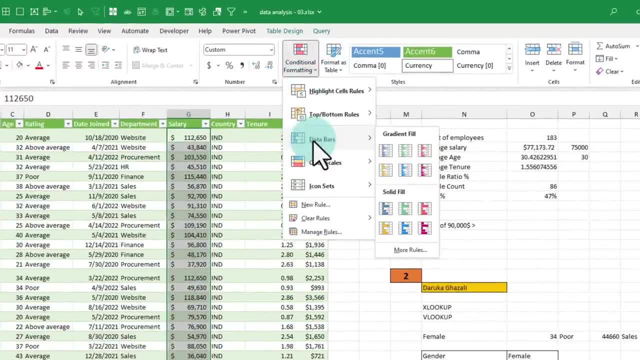 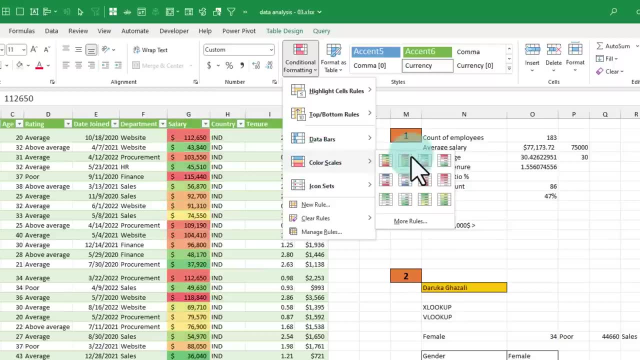 conditional formatting, apply either a color scale or a data bar. let's go with color scale because i think that is better suited for this situation, and we can pick a color scale like green to red- green being higher salaries are green color and red being lower salaries are red color. 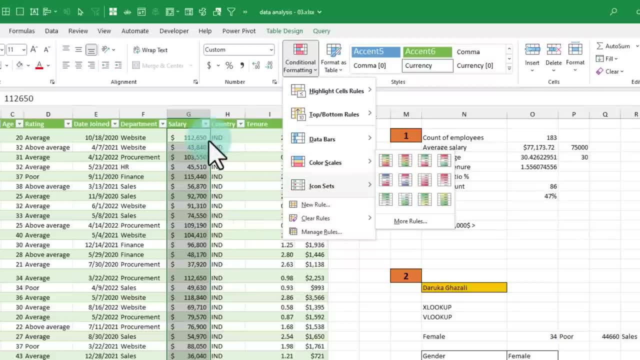 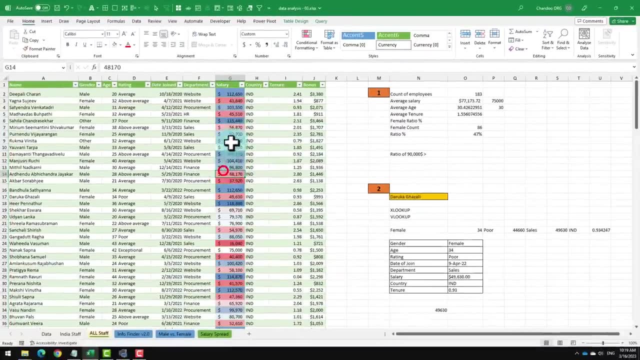 if you are thinking that green kind of coincides with my table formatting, here you could also use blue to red, which kind of contrasts well with our data. so let's go with that and that kind of shows you how the values are spread. but this is a quick and dirty one and 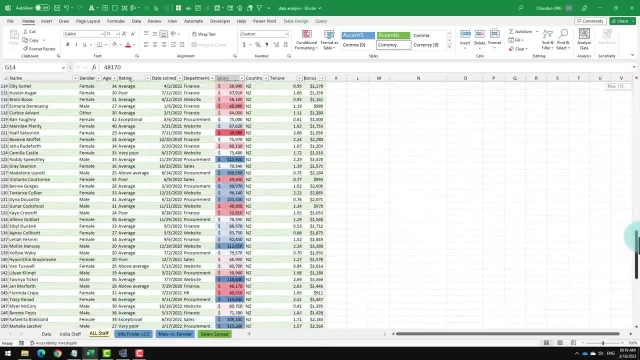 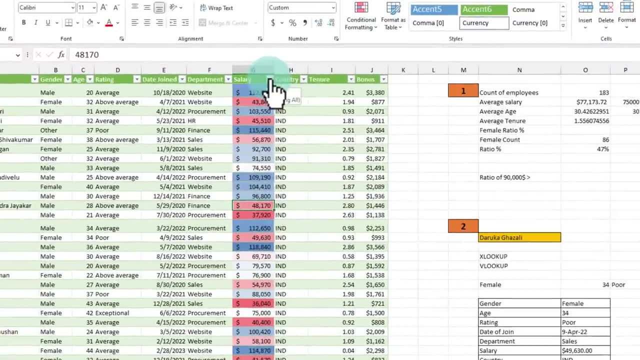 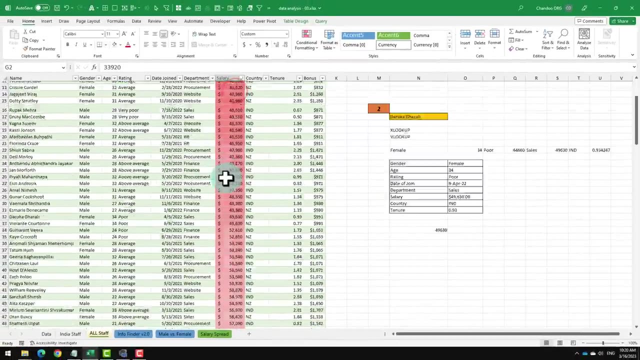 when you have hundreds of rows of information, it might be hard to get a visual sense of your data. once you do have this, here is one other handy trick that you can apply. you can also apply a sort order, so if i do smallest to largest, i'm going to get a nice spectrum going on here. 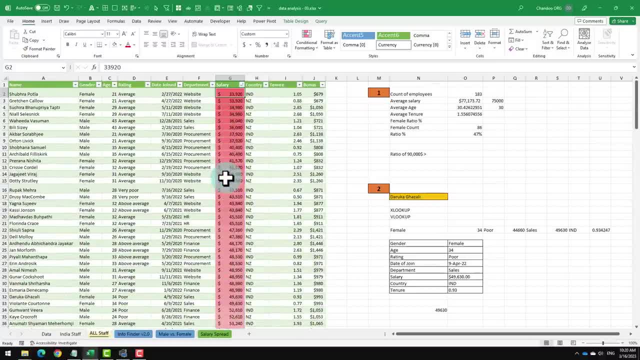 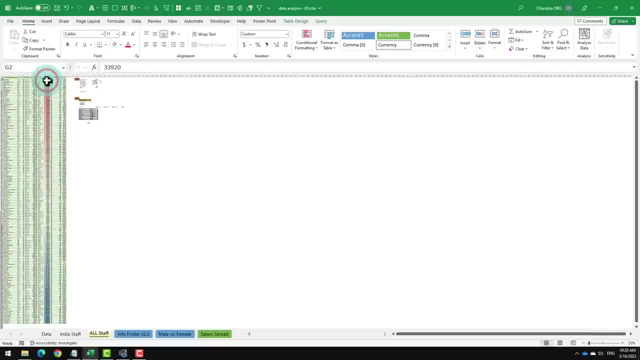 that shows the spread of our salaries. so let's zoom out a bit. now you can kind of sense how that spread is looking. it kind of looks up fairly, even to me, but i'm not really sure if there are some extreme values or not. so let's go back and try something else. 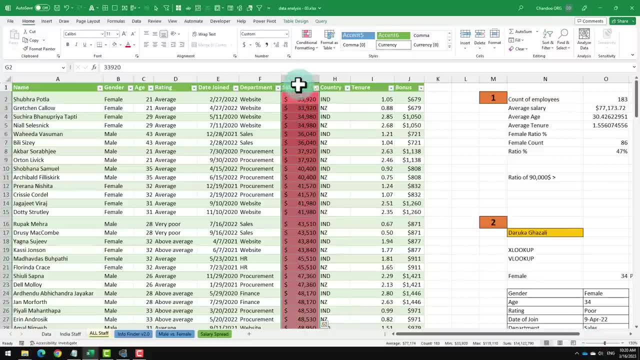 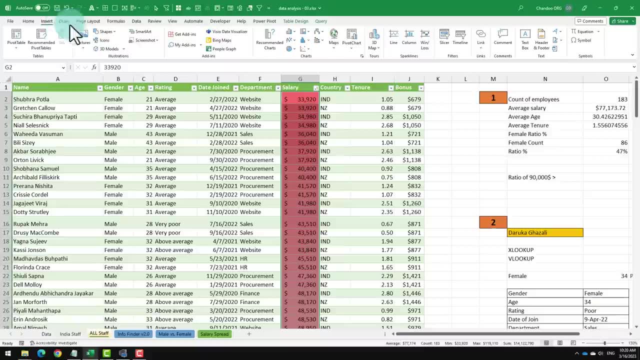 the next option is we can select the salary column, that entire column, and then we can go to the insert ribbon and use one of the statistical charts to quickly do the analysis. These charts are newly introduced into excel 2016 and 19, so if you are using a really old version of excel, you will not find them in. 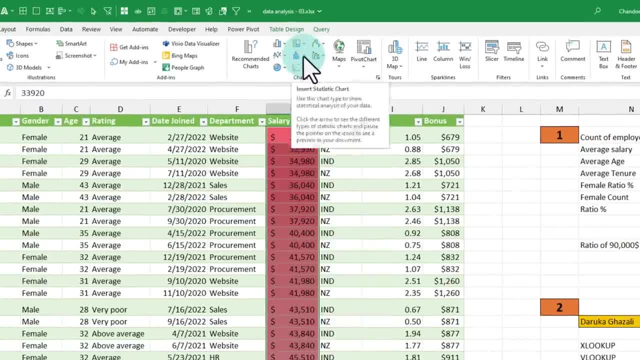 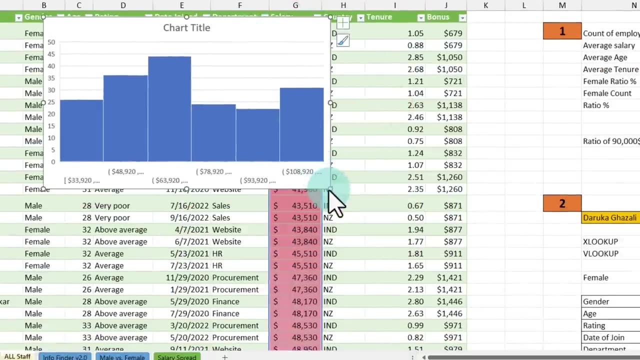 your excel. So from insert you are looking for this histogram or statistic chart option and from here you could try either histogram or box and whisker plot. I am gonna try the histogram option first and this will give me a histogram of our salary. spread It kind. 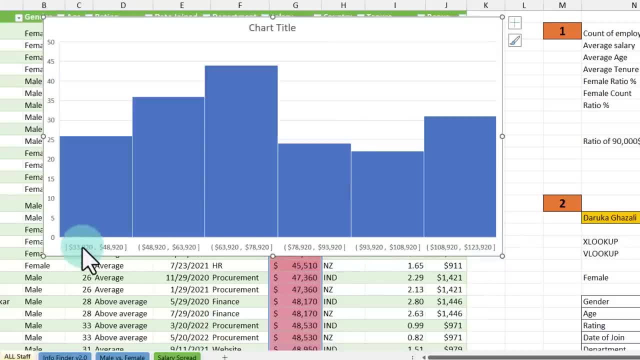 of looks a little bit funny. that's because the initial bucketing of these groups it starts from 33 to 48, 48 to 63, like that. This has no meaning, so I am gonna select this axis and then press ctrl 1 to format it From here. instead of automatic binning, I am gonna specify: 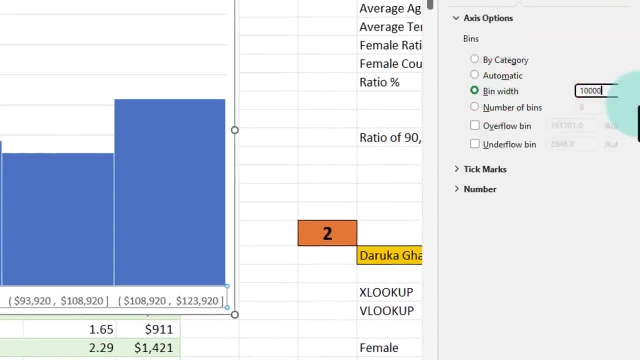 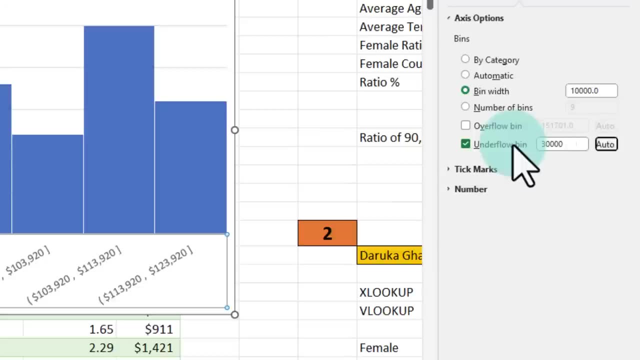 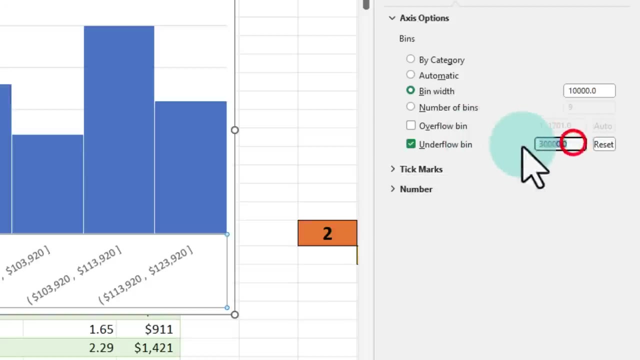 the bin width of. Let's just go over here. Let's go with $10,000 at a time and we'll start an underflow bin at 30,000.. What that does is it will begin the lowest salary at 30,000.. 30,000 doesn't seem to work. Let's 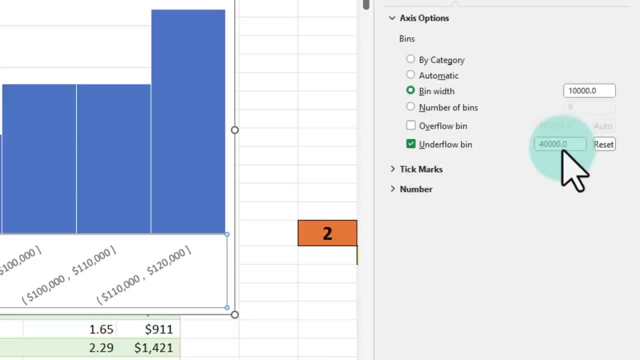 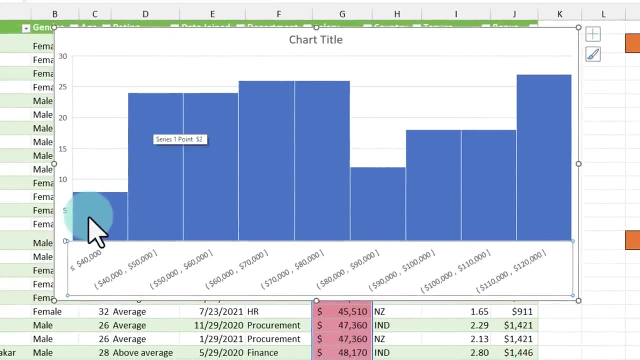 go with 40. So from 40, 40 to 50,, 50 to 60, like that, and now we can kind of get a sense of our distribution. We have very few people under 40,000. Just about 7, and then most of the majority of our employees are between 40 to 80,000. 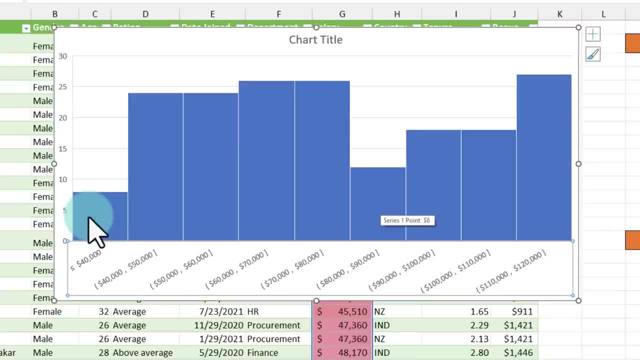 and then between 80 and 90. we surprisingly have very few people, But then it picks up again and we do have a significant number of people, between 110 to 120.. So this kind of tells a story of what is happening and with about just 180 people there is not much. 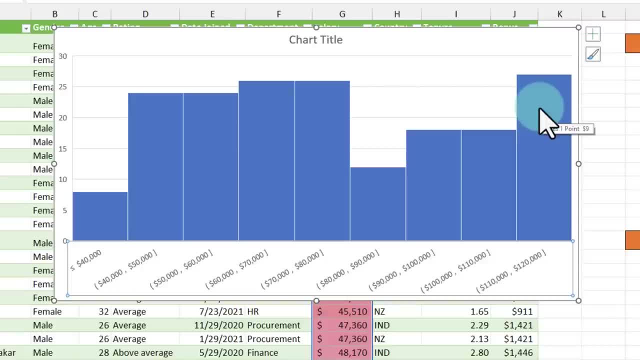 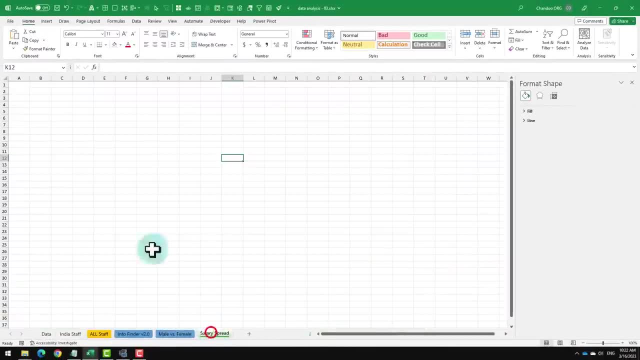 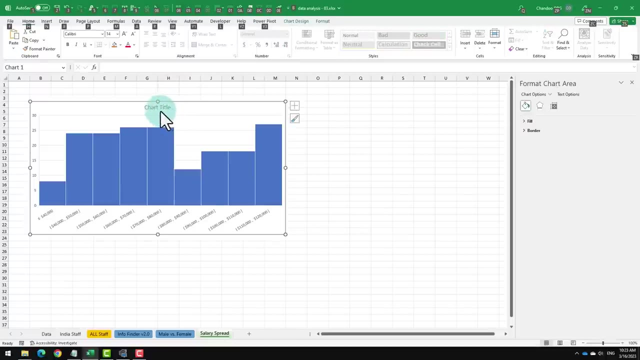 but if you apply this technique over a large set of groups, Set of data, then you can quickly get a sense of how the values are spread. Let's cut this chart and paste it into our salary spread page. So this is our salary spread by $10,000. 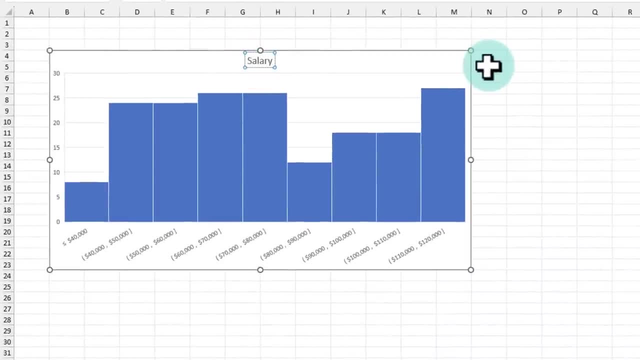 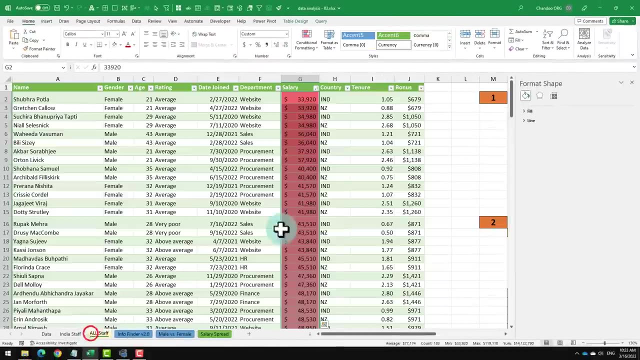 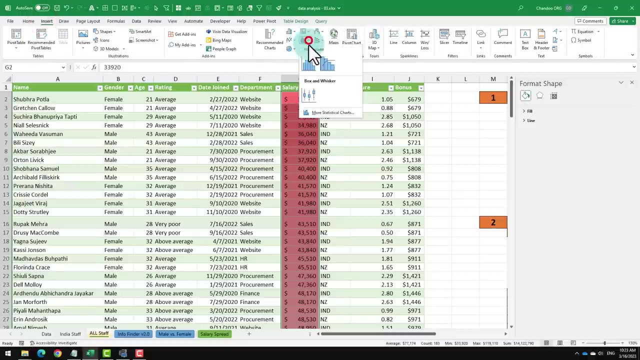 and you can apply that as a title. So this is one analysis. Now let's go and see what else can we do to understand the salary spread. While keeping the salary column selected, you can again go to insert, and let's try the box plot option. 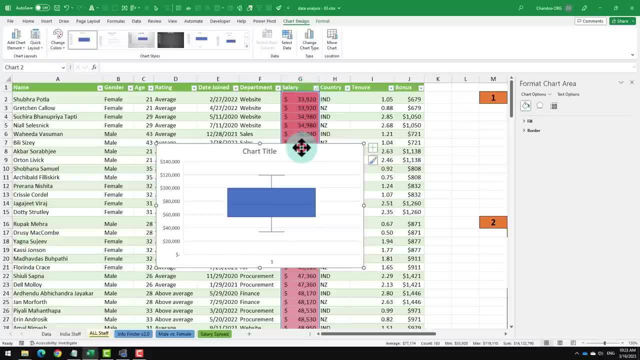 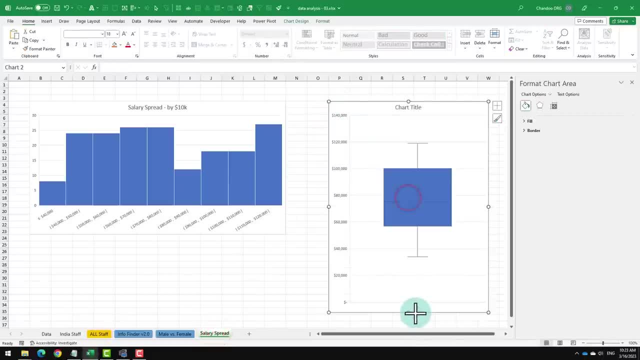 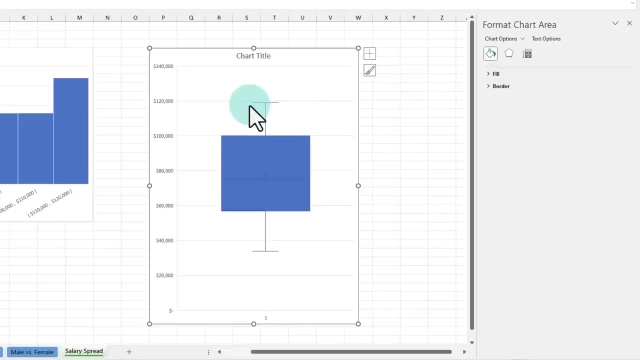 which shows the entire salary in a box plot diagram. I'm going to cut this as well and put it here, and then I will explain what this is trying to do. So a box plot shows your entire salary as a box, with these two whiskers at the end. So the middle chunk is the mid 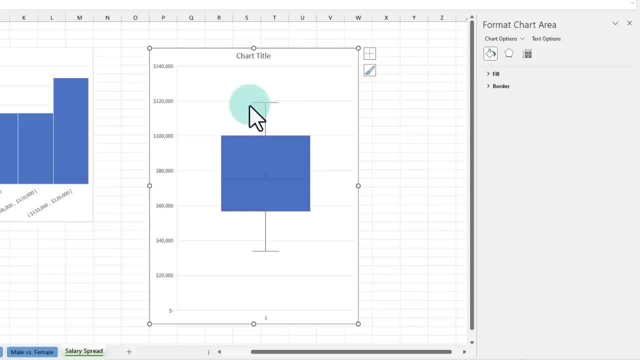 half of your total salary. So the middle chunk is the mid half of your total salary. So the middle figure of the total salary is $9500.. This line refers to the median midpoint of the salary and then the x marked is the average and previously, when we are looking at the 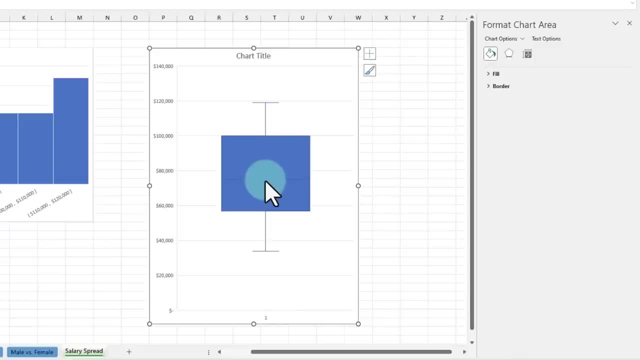 numbers, we kind of knew that the midpoint is less than the average, so that's why the x is above it, And then this box is the 75th percentile and that box edges the 25th percentile edge. So essentially of this kind of tells me that middle class, or the mid-half of our 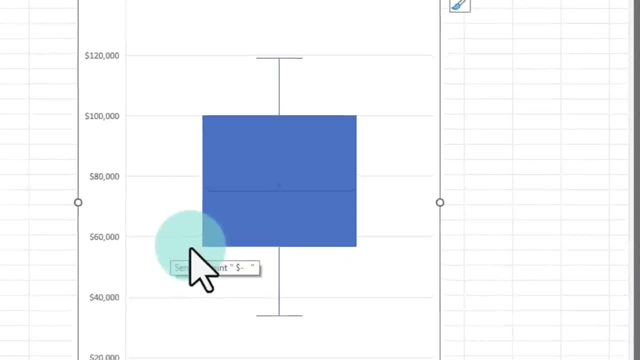 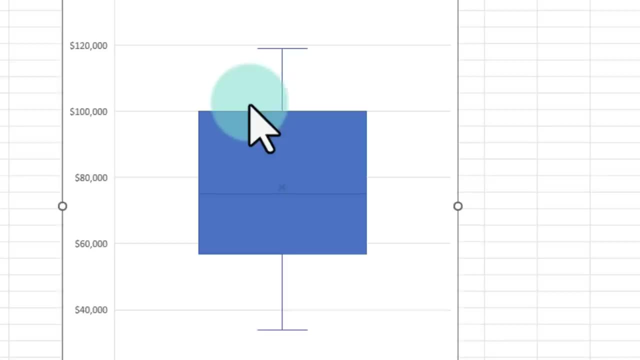 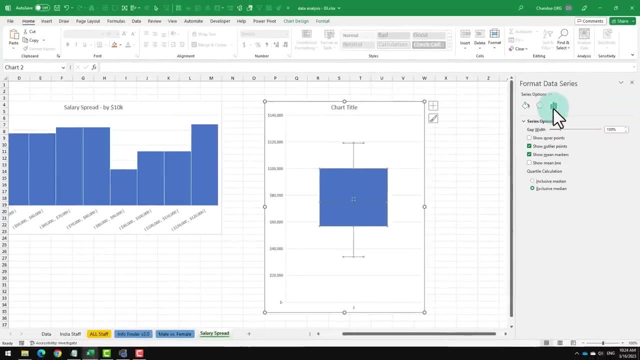 employees. their salaries go from maybe around 55, 50 000, 55 000 all the way up to 100 000, and then we do have some people here, some people there. there seem to be no other extreme values, but i'm just going to select this. go here and, yeah, make sure that show outlier points is checked even. 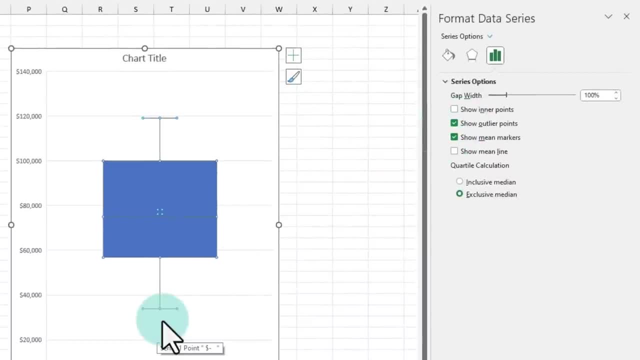 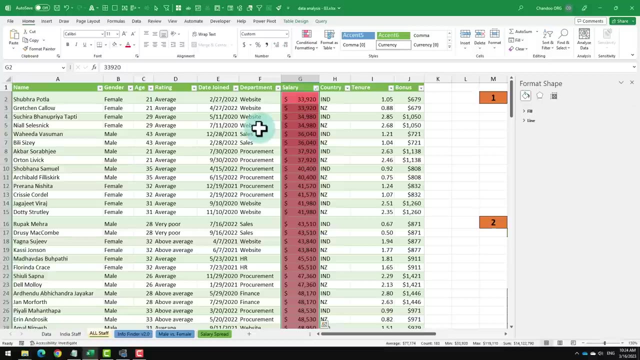 when that is checked, there is no outlier. so no, nobody has extreme values in our data. that's why this looks like this: let's see what happens if we kind of artificially change somebody's salary. so i'm going to take, uh, these two guys salaries and then let's just make this 25 000. 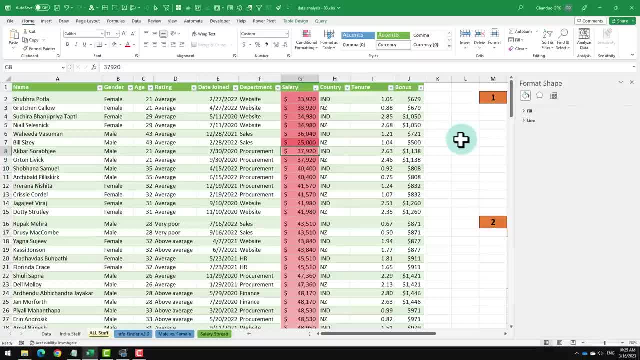 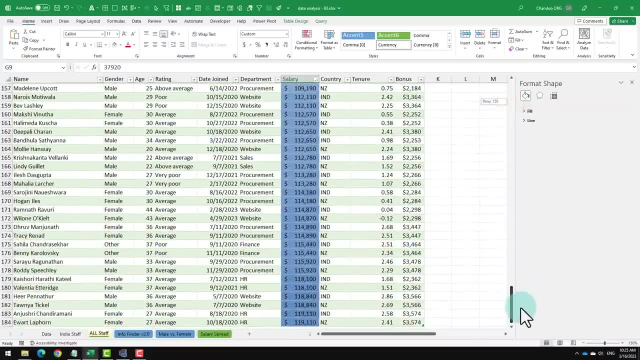 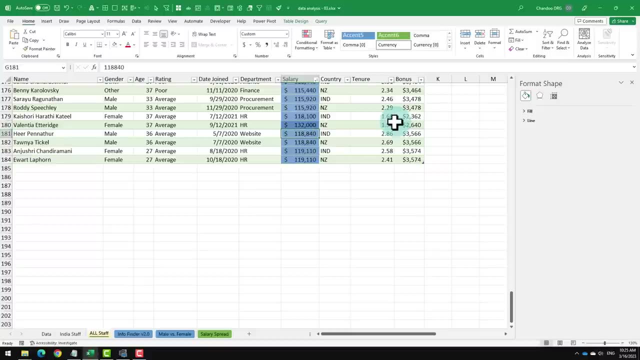 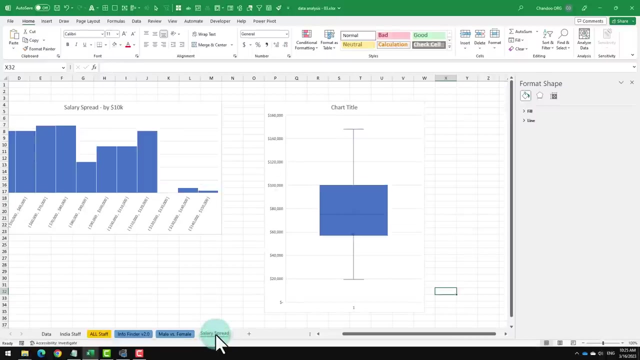 uh for here and then 19 320 for this person. so we introduced some really extreme values at the bottom edge. i'm going to take some of these people and then make them 132 000, 148, 000, like that now when i come. even then they are not extreme, because i think they kind of still. 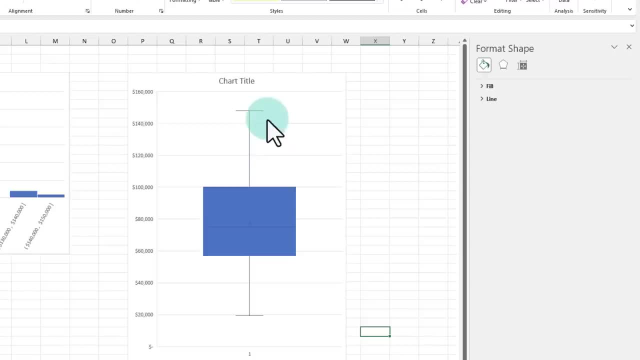 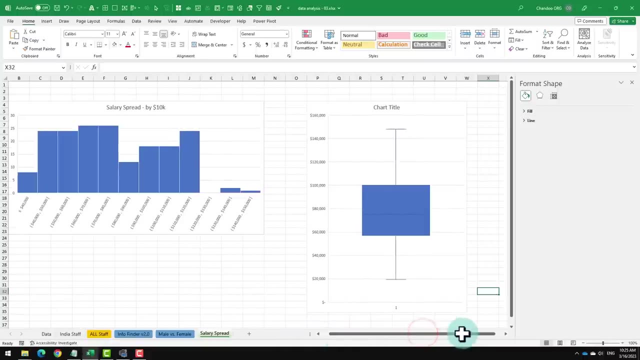 fall within, uh, the natural expected range. but now our histogram change it and it kind of has these extra things at the end. but if you do have some very extreme values, you will have some very extreme values. so i'm going to take some of these people and then let's. 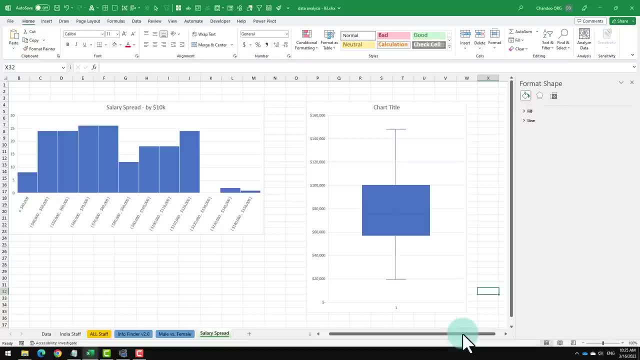 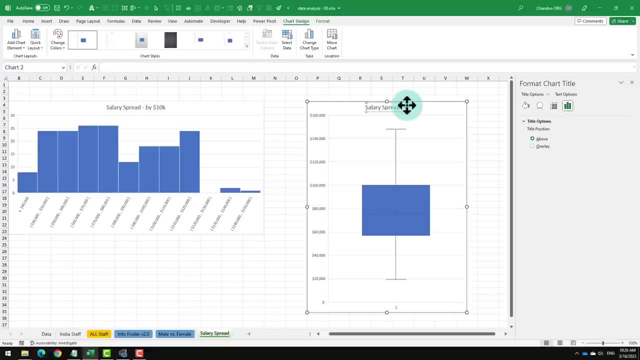 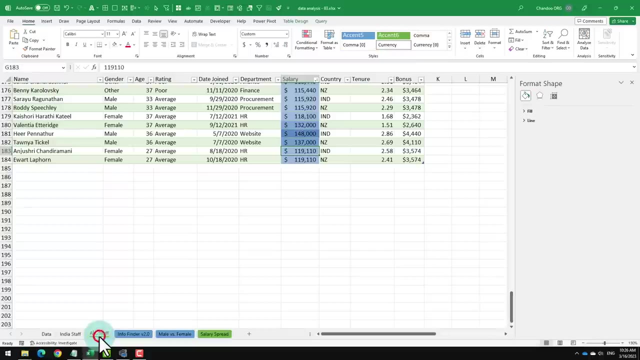 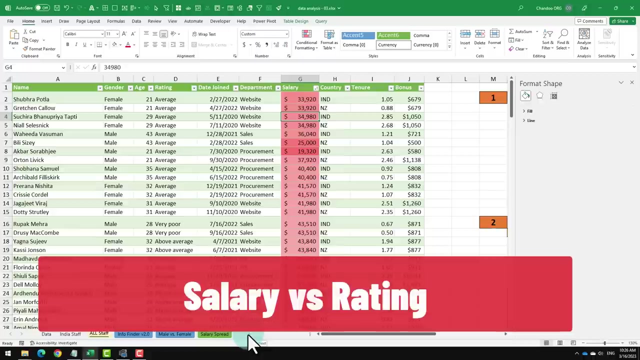 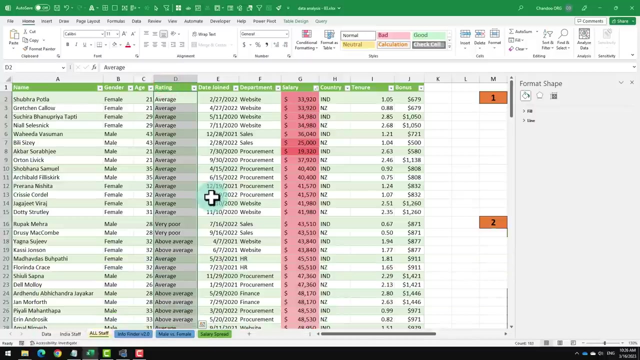 have that as a pointer identified in this box plot. so this is our salary spread box plot. now let's answer the second question, which is: is there any relationship between salary and the rating that an employee gets? we're going to try two different ways to understand this particular thing. one is through a pivot table and another 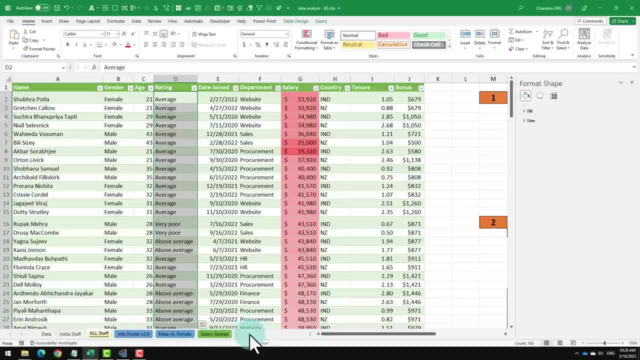 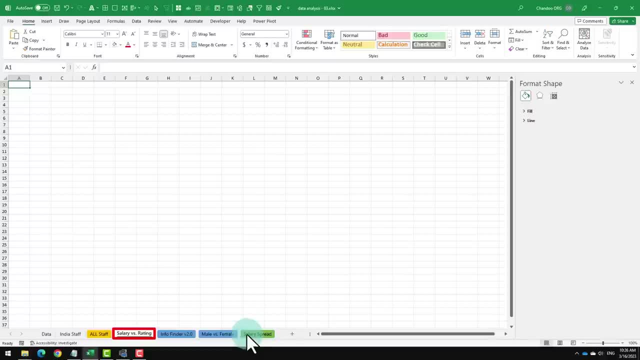 is through a chart. so for our pivot table i'm going to add a new worksheet, salary versus rating, and here insert the pivot table. remember, in the earlier step we have added the pivot table to add this data to the data model option. so now that that pivot table 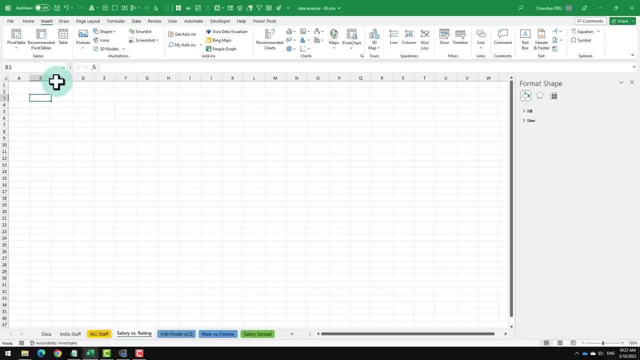 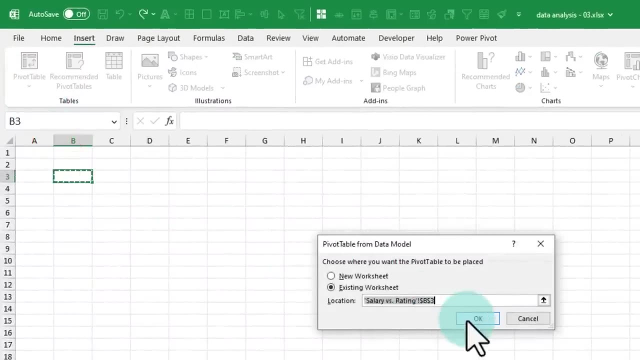 was created and then added to the data model. next time you want a pivot table, you don't need to go back and select your data. you can just go to the place where you want the pivot table and then straight away click pivot table from data model option. this will bring up the original. 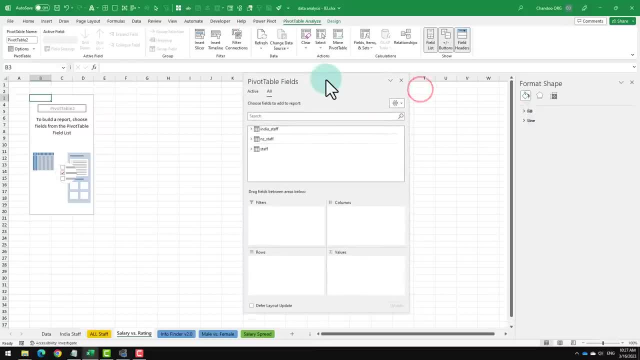 data that you have, push it to the date model and then it will show you that. in fact, it's going to show you even the india and new zealand staff tables. we don't need that, we only need the staff table. so i'm going to use that and from here we are going to put rating into the row label area. 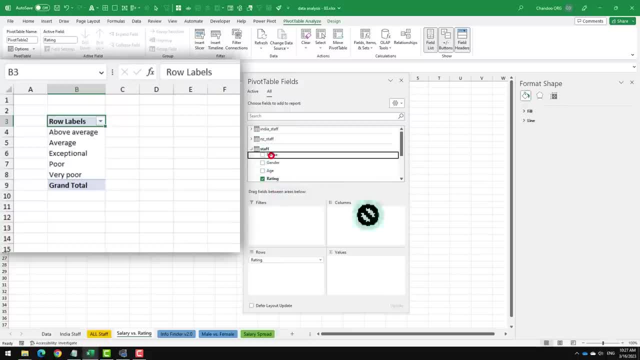 and then take something like name and then add that so that we can see how many people are there. by rating groups, a majority of our employees are average rated. we have only four people exceptional and six people very poor, so it doesn't really tell you much, but you know. 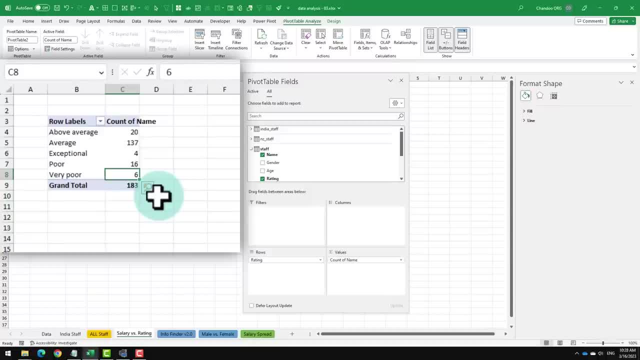 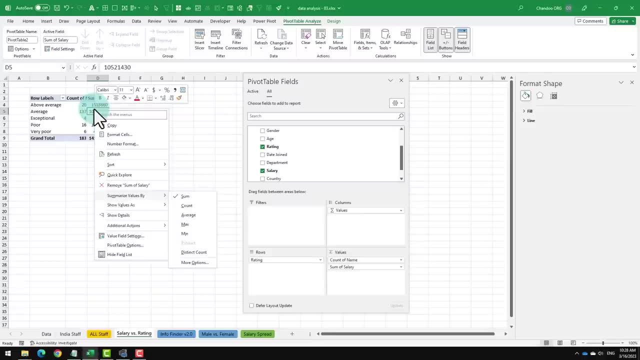 you can still understand what is happening. how many people are there? now let's see how well they are paid. so i'm going to take salary and put that there, right click and then change this to average salary so that we can kind of get a sense of what the 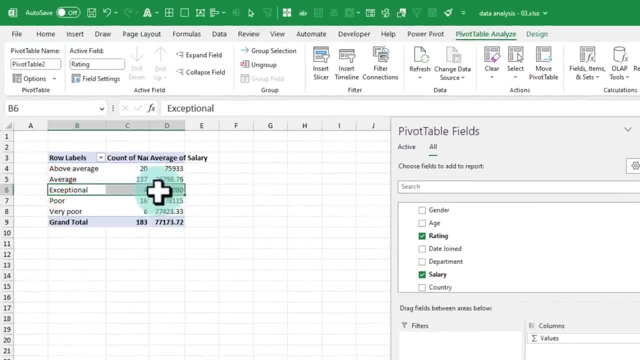 average looks like our exceptional staff are paid really high, so they have 92 000, but everybody else seem to be around the same ballpark. one way to read this better is if we arrange these ratings in a better order. right now they are in the alphabetical order, and that is not a good way. 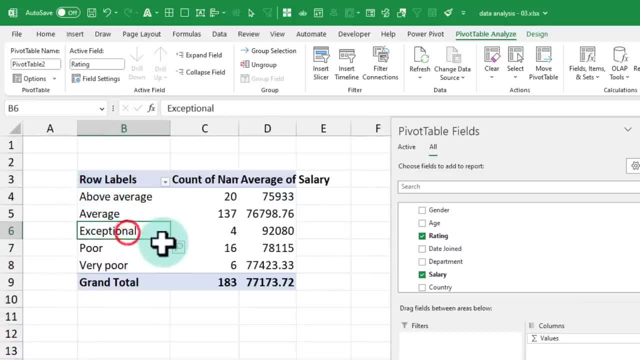 to do it. so to fix this problem, what we can take do is select the label. that is exceptional, and we want this to be up top. so, once you have selected, place your cursor on the edge of the box. it turns into that black colored arrows, click and drag and move it above. so, exceptional, above average average. 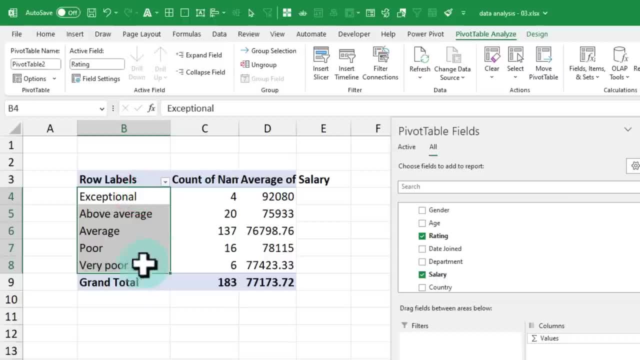 poor, very poor. so this is the correct way of reading this set of information. that is how the distribution looks and that is how the averages look. when you have a bunch of numbers like this, sometimes it may be hard to kind of see which numbers are big or small, given that some of them have decimal points and whatnot. 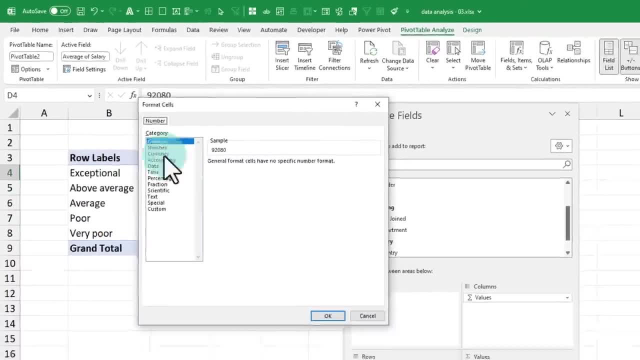 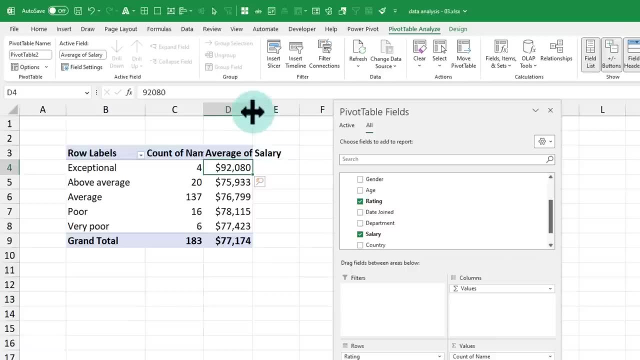 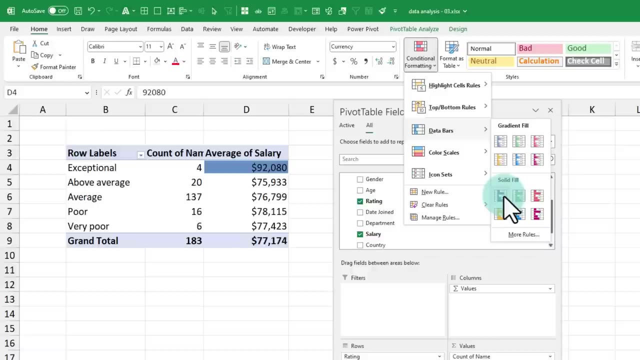 so a good idea is to do number formatting and apply consistent formatting for everything so that you can quickly see the numbers better. the next trick that i like to do is maybe add conditional formatting data bar on this, so when you add a data bar in the pivot table, 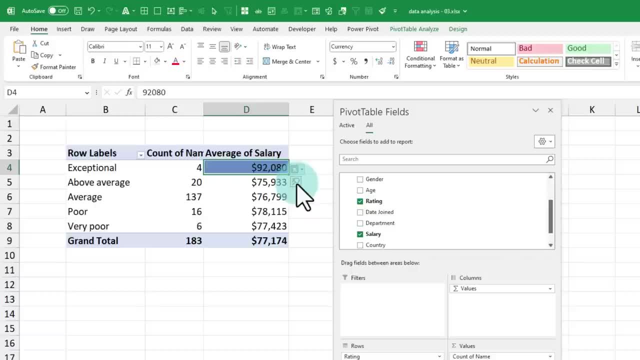 usually it gets applied only to the value that you selected, but you'll have this extra button here and from this you can select the third one so that the bars are applied consistently and you can see what's happening. while the exceptional people have very high salary, these other people, their salaries are all around the same number, in fact very poor, and 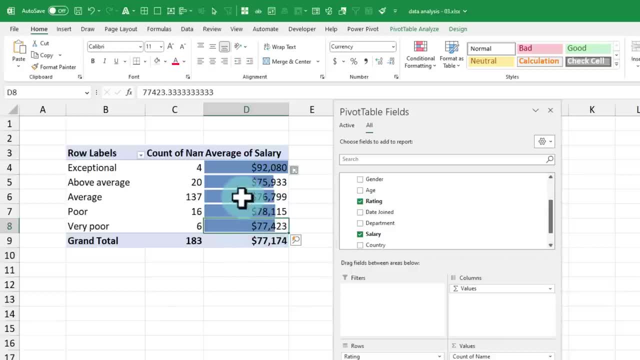 poor people actually have higher average than this group, so we can kind of say that probably not much is going on. with respect to rating versus salary, it's one thing to be rated at a very low level, but you might still be paid higher than on average than the people who are rated. 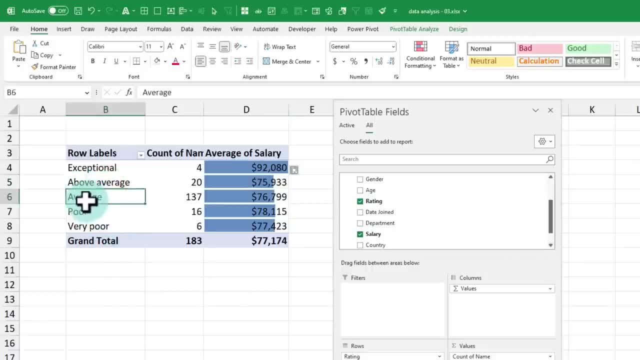 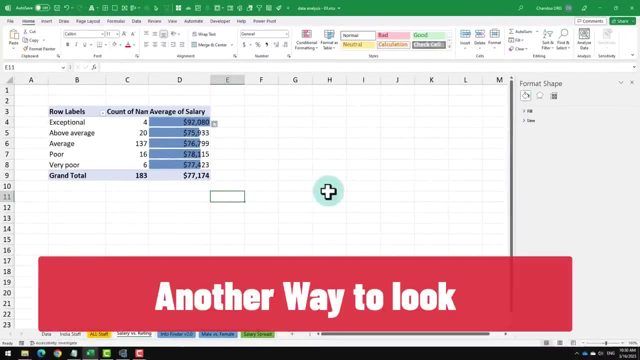 above you, but also because we do have a significant group of people in average rating, it might be hard for us to kind of spot and understand what is going on. now that this thing is done, let's see if there is another way to look at this data and see what is going on, for that to happen, what we 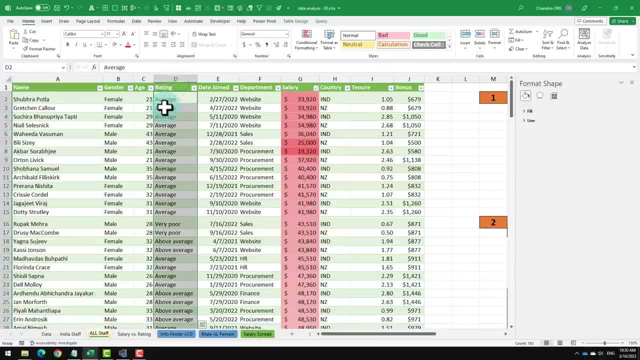 also need to do is for each of our ratings, we need to give a numeric value as well, because these are text values, and we need to give a numeric value as well because these are text values and we need. it will be hard for us to do the analysis correctly. we need to assign a number value. 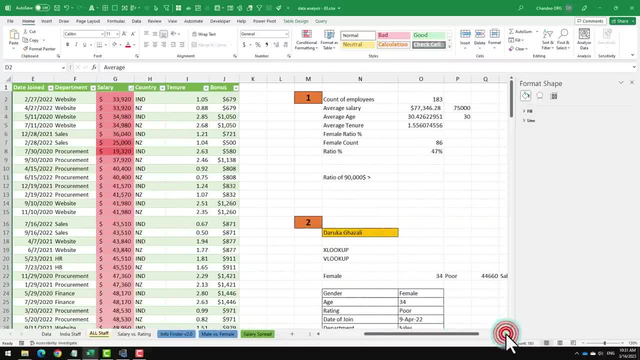 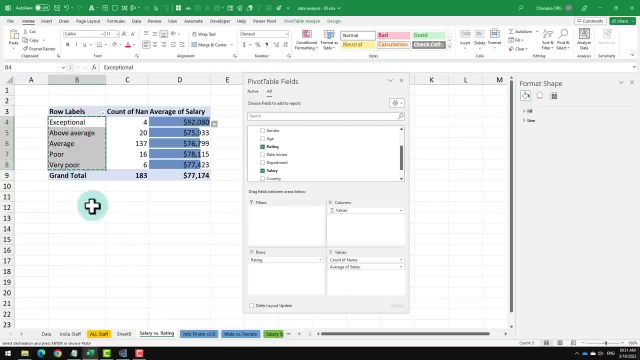 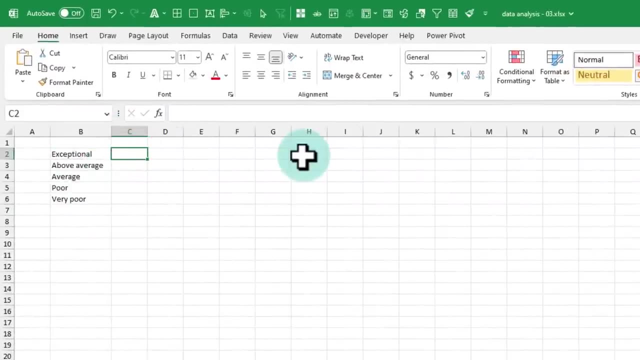 for each of these ratings. so i'm going to first set up a mapping table. we can do this in a new page here. i'll copy these five words from there and then paste them here as values, and then the number for them is: let's just go with five, four, three, two, one. 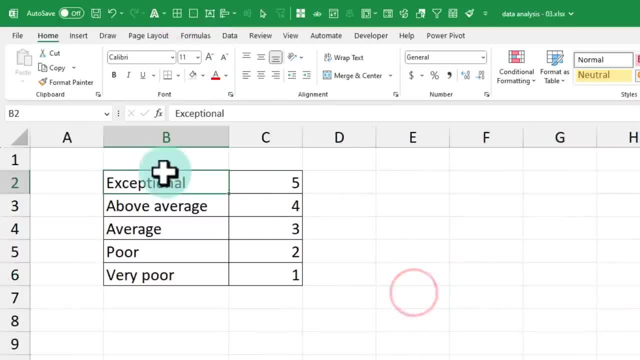 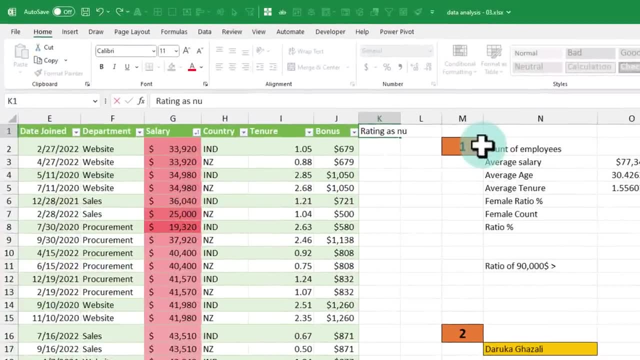 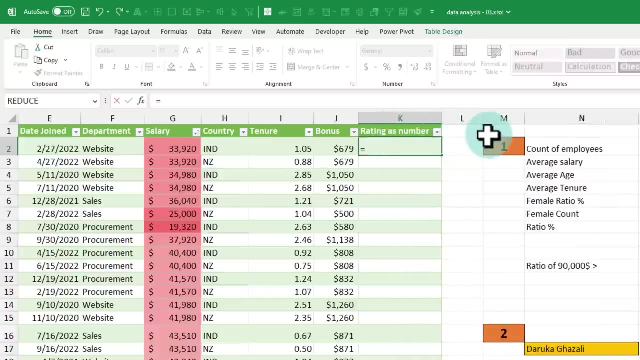 so this is the rating and that's the corresponding number value. and now we can come back here, rating as a number, and then quickly calculate what is the rating as number. this way is where we could either use xlookup or vlookup. i'm just going to use xlookup. 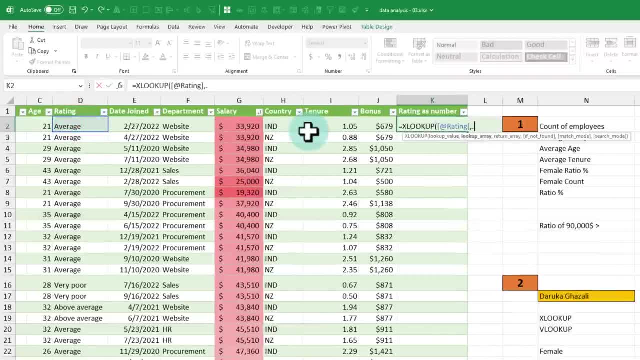 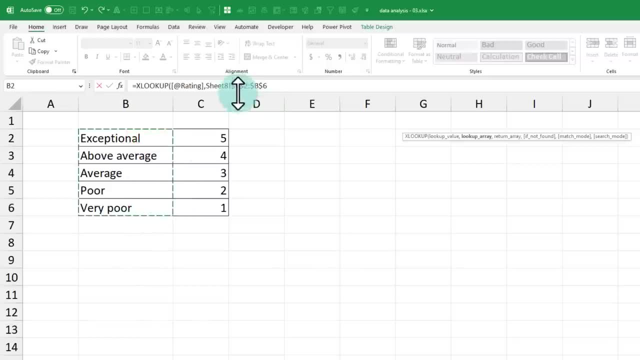 xlookup rating and then go to this column here, make sure that it is absolute reference- so it should be b dollar 2, b dollar 6- and then select this column. make sure that is also absolute. when you have a formula and you need to quickly change the reference style, you can press the f4 key and keep pressing it until 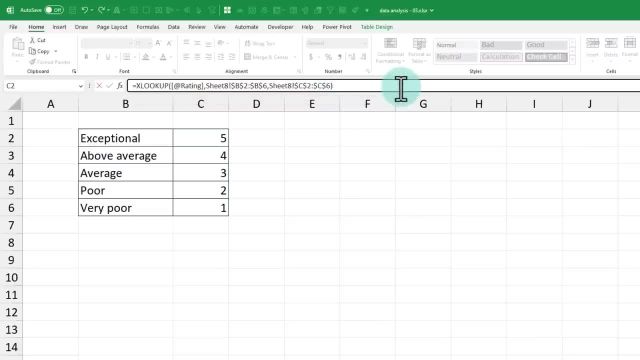 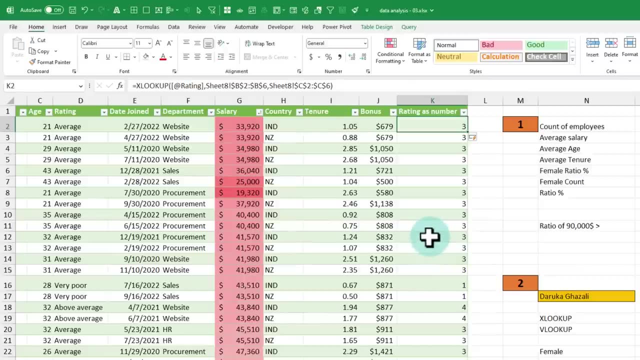 you get the style you want. so now that that is ready, we'll close that and we'll get the number representation for all our ratings. you might think what is the point of this, but you will quickly understand once we make the chart that i want to build now that we have salary as a number and rating as a number. 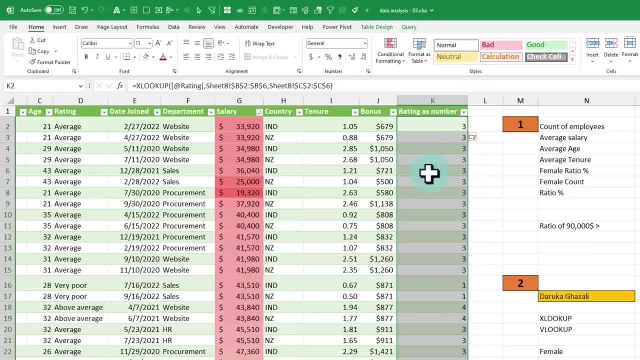 a quick way to visually explore this data is to make a scatter plot. where rating is on one axis, salary is on another axis. that way we could see if there is anything funny going on with these dots. so i'm going to select my salary column, hold down control and select the rating column- both columns. 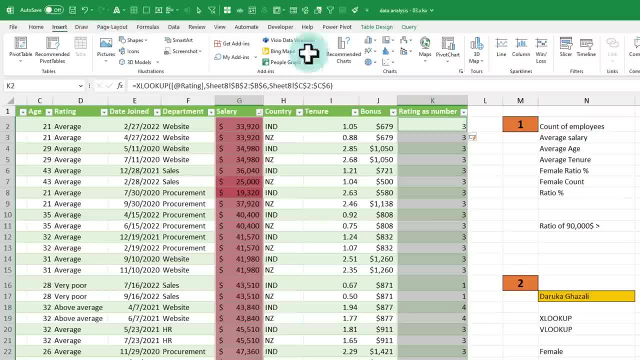 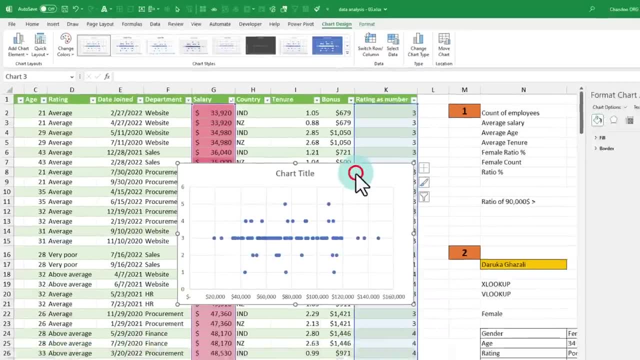 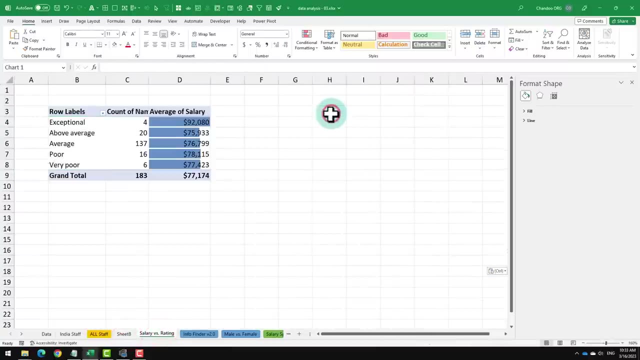 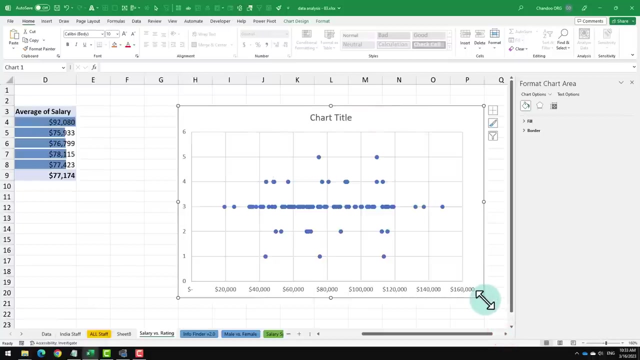 are selected and then now i can go to insert ribbon and click on the scatter plot option here and then add a scatter plot and i'll control x this and move it right next to our pivot table here. so this is how our salary versus rating looks like. 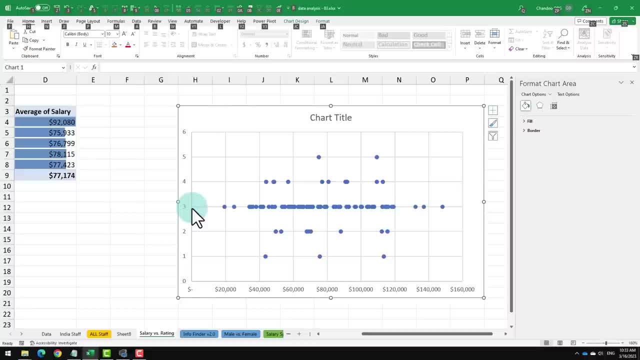 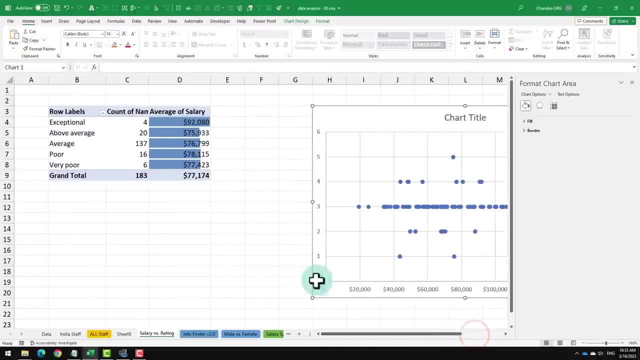 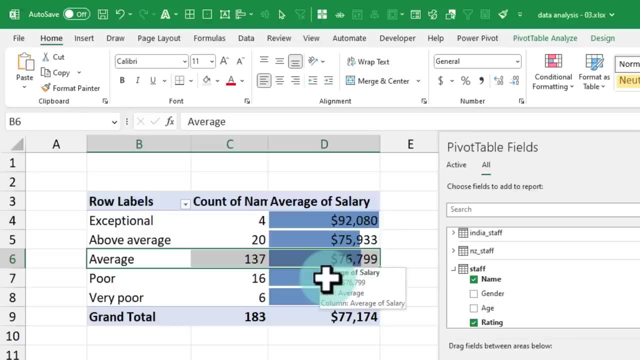 three is the average rating, so that is the middle one. a lot of people are in the middle, some people are on the high, like that. so earlier when we were looking at the average, the average is only 76 799 and we thought on average an employee who rated average has lower salary. but if you look at the actual spread here, 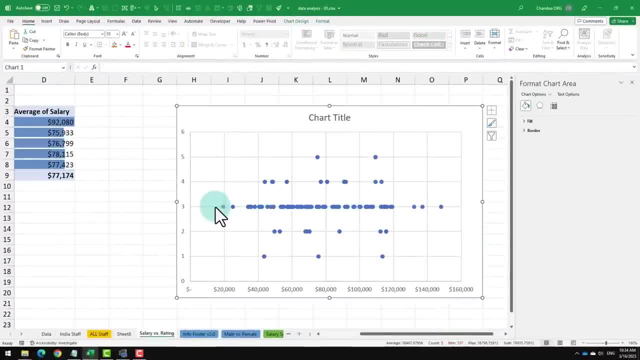 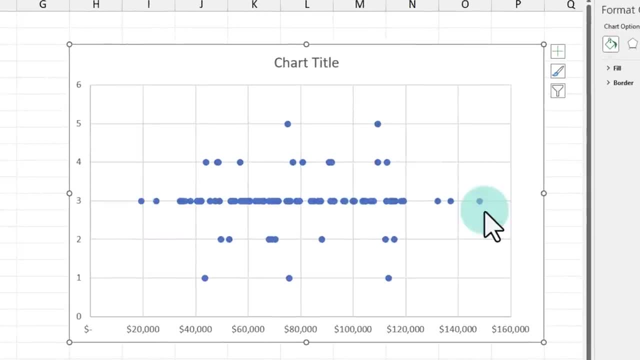 you can see that somebody rated average, that is three. their salary could be anywhere from 19 000 all the way up to 148 000. remember i adjusted some of the values earlier to pull up the box plot, so that's why these three dots are there. so in fact the average group has like a really wide spread, whereas the 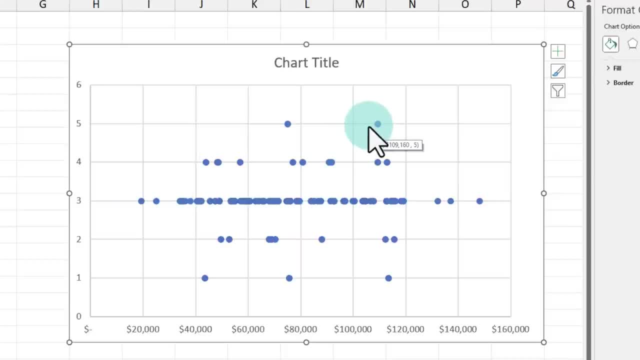 exceptional group has really two salary points, hundred and nine thousand here and seventy five thousand, and probably this is why their average is ninety two thousand, because maybe there's like two people here, two people there, and that's why the average is coming up to be ninety two thousand. 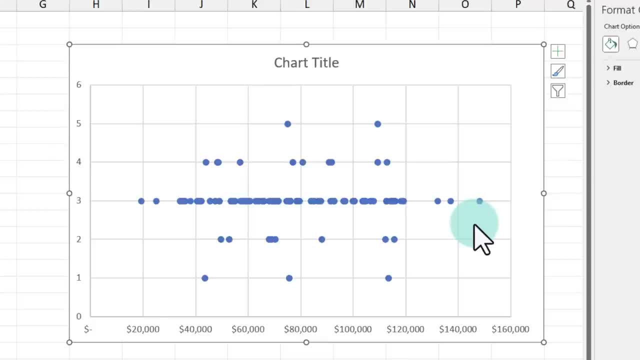 as this spread shows a little bit more wild thing. So using a scatter plot is a really fun and powerful way to quickly see how your data is and understand. The only way we could do this is if both axes are number. Our salary is already a number, but the rating was text. that is why we 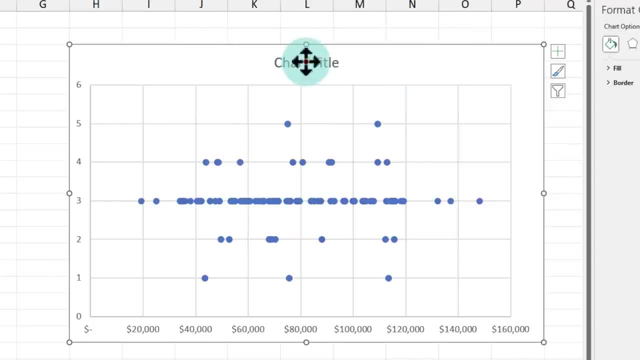 had to have that mapping table to create that. Let's name this as salary versus rating. And again, because of the way this diagram looks, I couldn't really conclude anything meaningful from it. It kind of doesn't tell me much, but if you do apply this technique for some of your business, 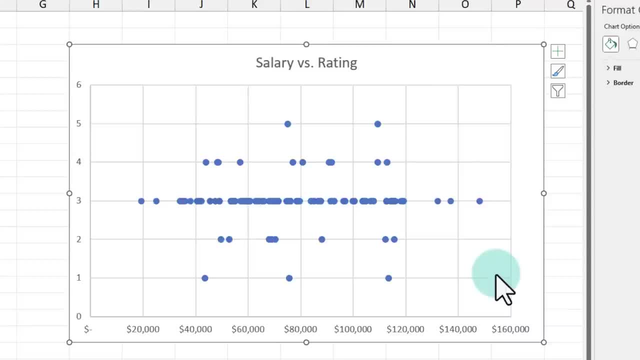 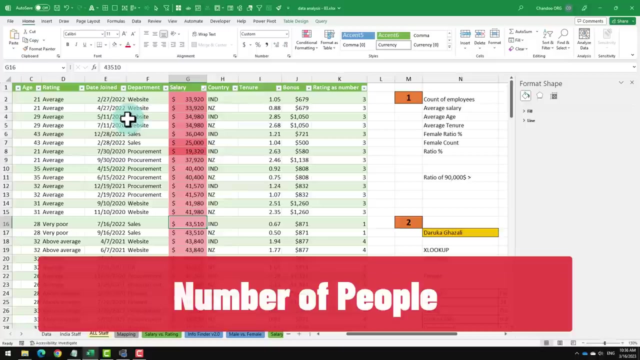 data. you might actually see a meaningful pattern here and then that might help you go and investigate the data a little bit more to see if there is something strange or interesting going on there. Our third question is to understand how our company has grown in terms of number of people. 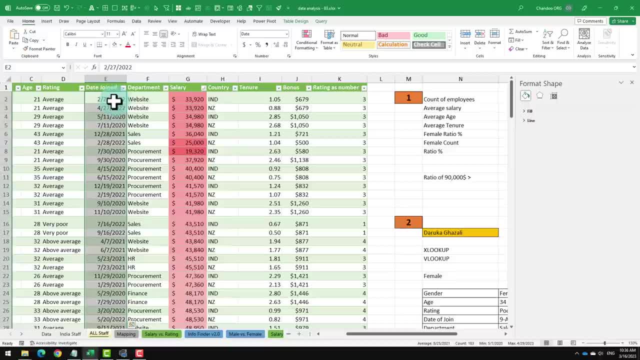 So we would like to see a trend of date joined and how many people have joined on each date as a trend. One simple way to do this is if I just take the date joined and then plot the head count against it, we will get an idea. But that's not going to give us much, so we are going to use some. 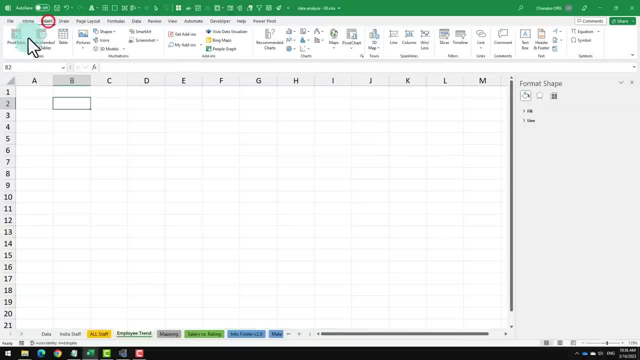 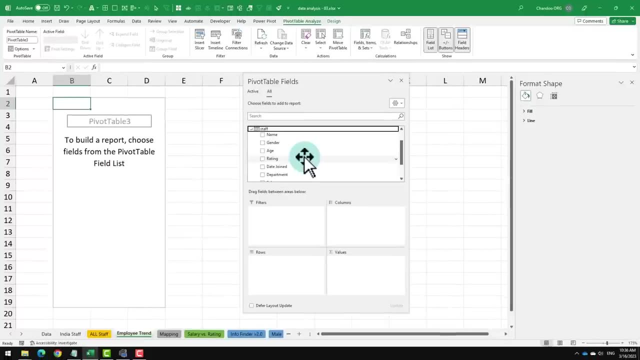 pivot tables and build this out slowly. We'll start by inserting a pivot table from our data model and go to the staff table, take the date joined and put that into the rows area. Whenever you have a date and you put that into pivot table, excel conveniently groups this data. 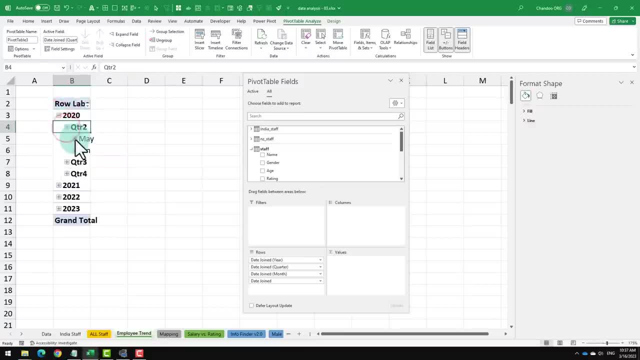 into year, within the year, quarter, month and day level, Let's say. for the purpose of this analysis, we just want to look at year and maybe at a month level. We are not interested in quarter, individual days. so what you could do is take out the fields that you don't want from the 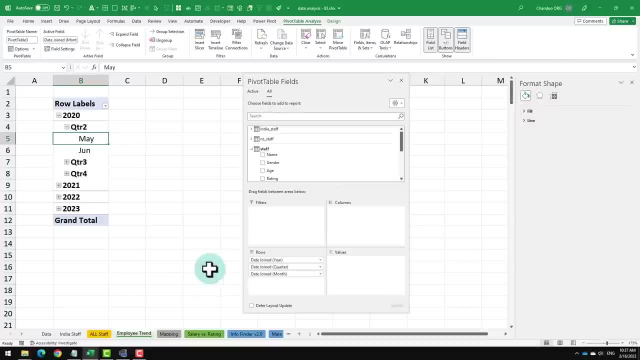 pivot table. just click and drag them, drag and drop them out so that they're gone and you will have something like this: and for each of those periods i just want to know how many names are there. so i'll take the name and put that there. so total is 183 in. 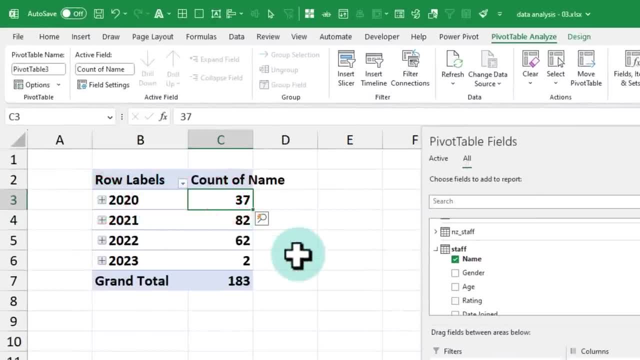 2020, when we started our company, we brought in 37 people, so really small. 2021 was our big year. we hired 82 people, then 62 more, and 2023 we just getting started, so we brought in maybe two people so far and at this point you can go and insert a chart like a line. 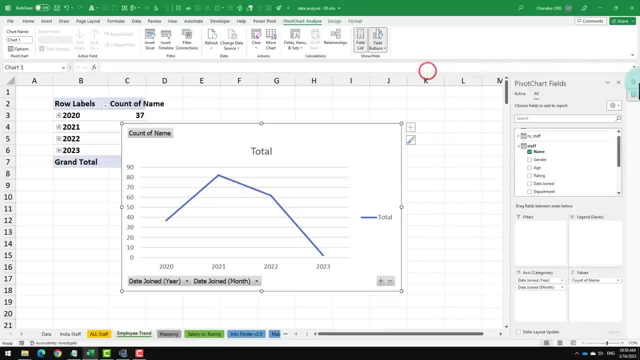 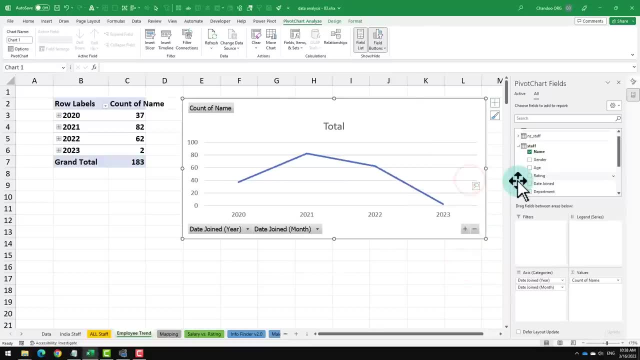 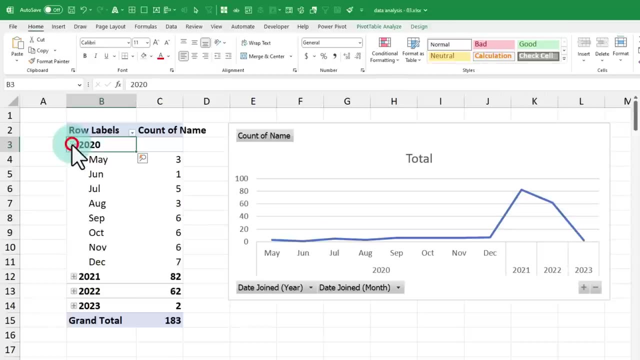 chart that shows you that trend, and, and, and, and, and, and, and. you can see what is going on. this chart is linked to the pivot table, so if your pivot table expands, it will show you the same expansion in the visual. i am just going to expand everything. 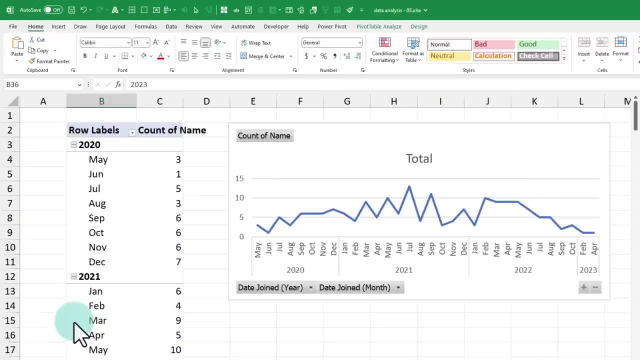 out. so this is how our company has been growing. we had a kind of like a hiring spree between march and september of 2021. we brought in a lot of people, people. then, jan and feb, here we. we hired quite a few people between feb and may, and now we are. 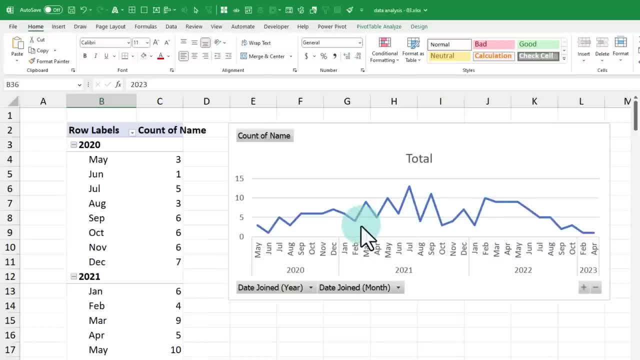 slowing down. the problem with this graph is it doesn't show the growth of the company. it only tells each point time what is happening. so a good way to visualize what we want is if we can get cumulative totals, that is, running total of these numbers over the entire period of time. so to do, 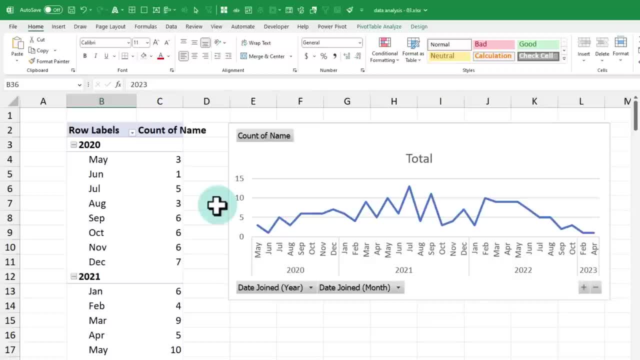 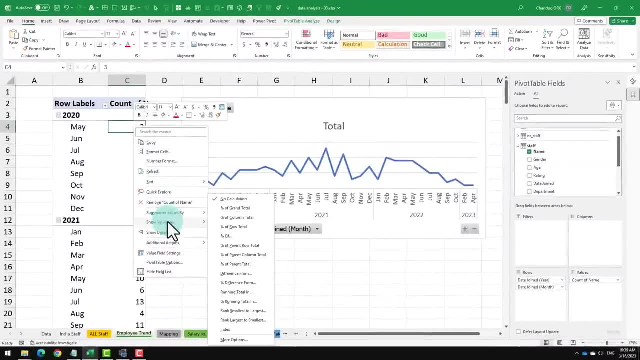 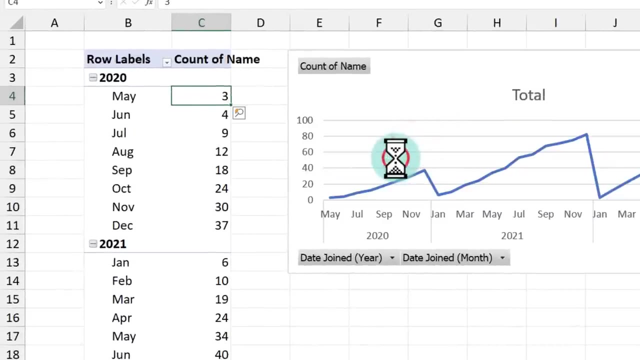 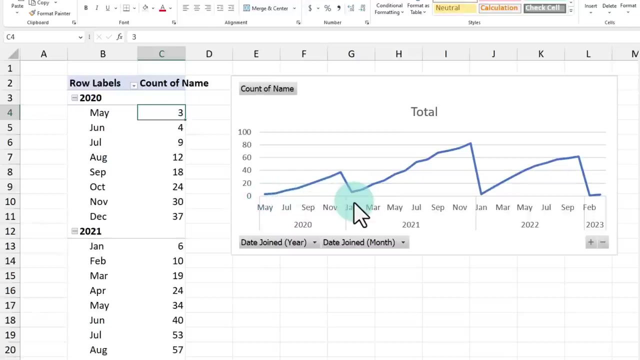 this: you could kind of build some formulas or do complex things, or you can right click on the number here and then say show value as and then running total option here. if i do a running total, i kind of get like these kind of spurts where it goes and then it resets. 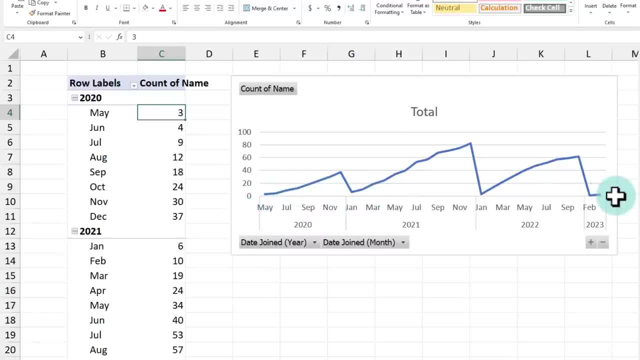 at the start of the year and then it shows you those three kind of spikes. so 2020 we grew from 0 to 37, then we started again from 6 to 82 and then it kind of went down 3 to so each year resets. that's because we have had- we have this kind of a two level structure here, so it 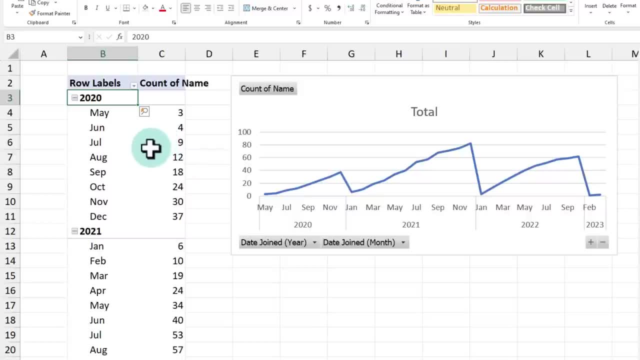 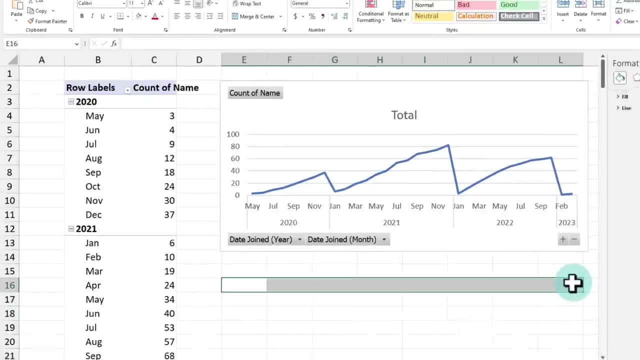 will always reset based on one of the fields that you pick in the running total. you might think, oh, this is good, but i don't really like this structure. how about if i want to just see an entire running total, right from the point of time that we started, all the way until end? and 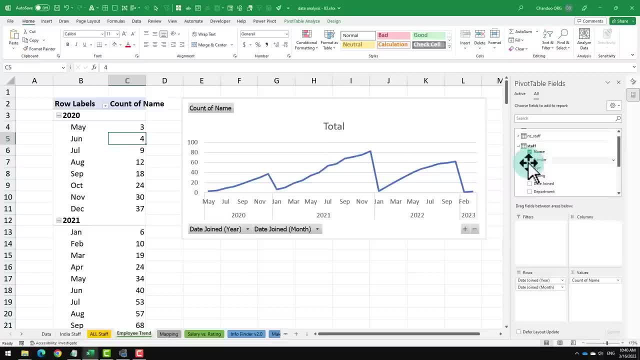 we could do that with two techniques. one is because we are already using a data model. we could use power pivot here to build a measure that calculates these kind of things. but that would be kind of like very advanced stuff and i don't recommend jumping into that straight. 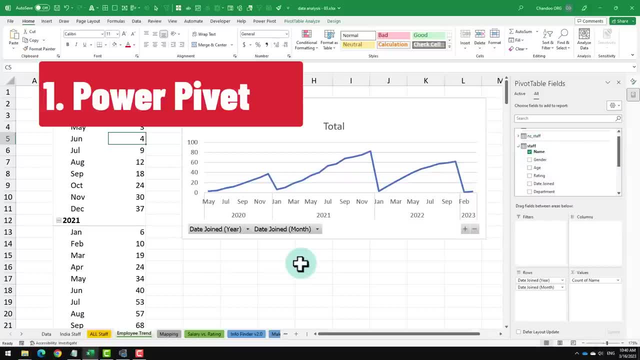 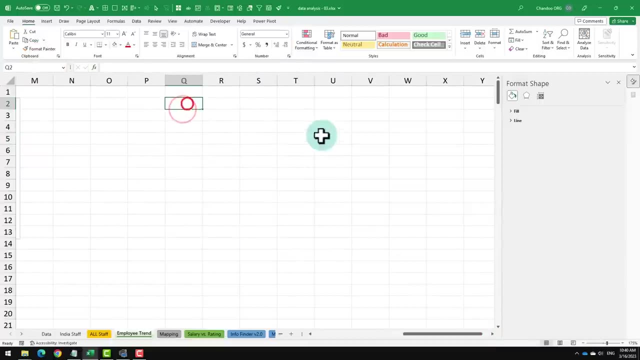 away. the second option is we could also build a page where we can do such calculations ourselves through some simple formulas. so let's do the formula option here. i'm going to use the same page but move it a little bit side and calculate our running total of employees here. so we're 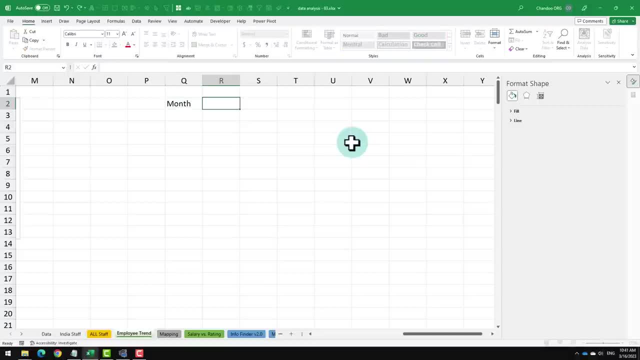 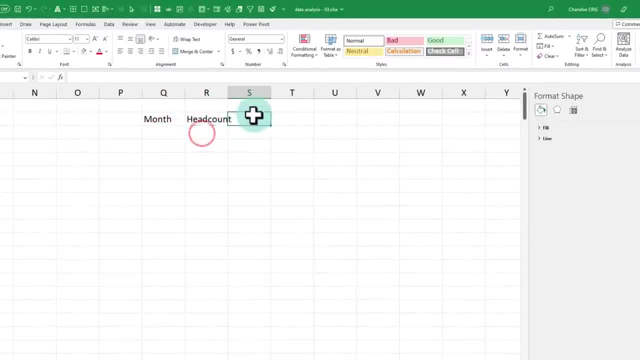 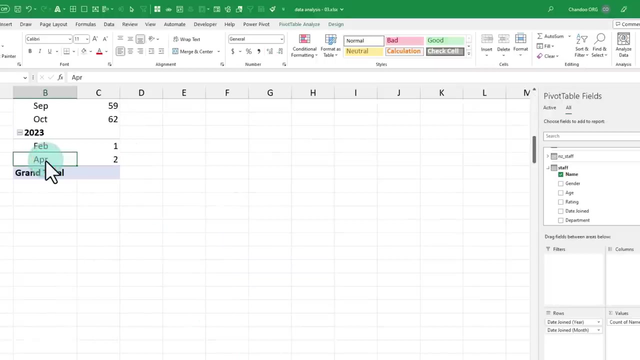 going to have two columns: one is month and then headcount. the idea is, for each month, what is our headcount, and then we can then calculate the running total here. so we started our company in 2020- me, and then we would like to go up to April of 2023. all the 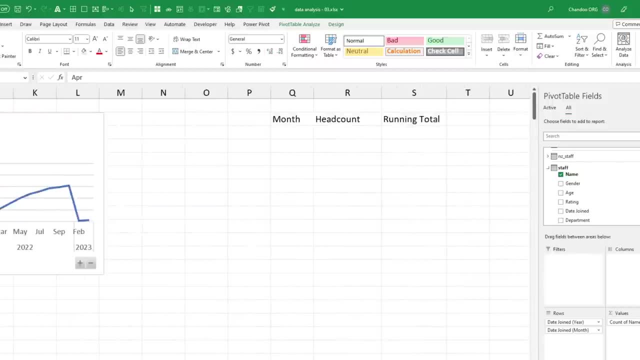 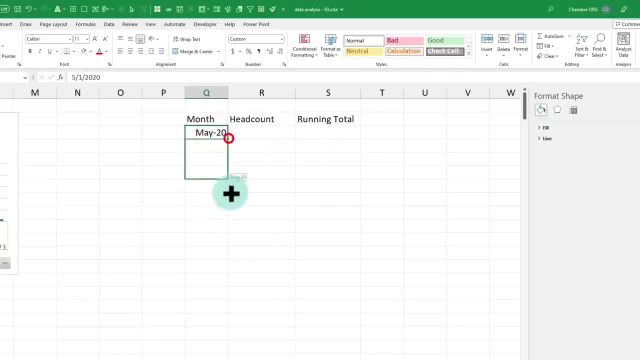 months. so I'm gonna say May 2020 and then you can just drag this down. if it is a one-off exercise, this is fine. you can just drag it down until you see April 2023, but that is not a fun way to do it. the next option is, for example: 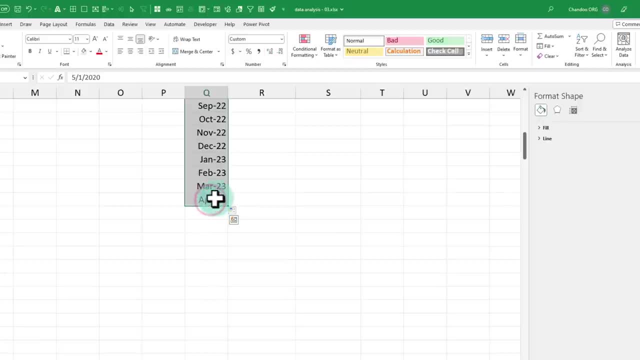 from May 2020. I would like to go up to three years, which would bring us to 2023 May. so, this way, what we could do is, instead of doing it like that, just select this and use the sequence function in Excel to generate the months. so initially, we are going to make: 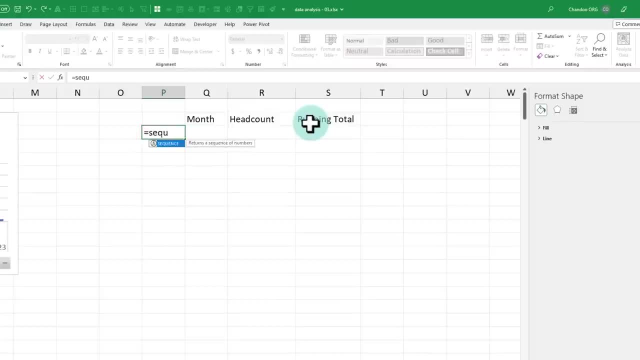 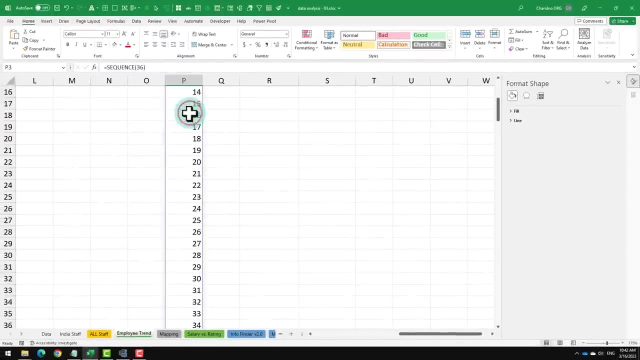 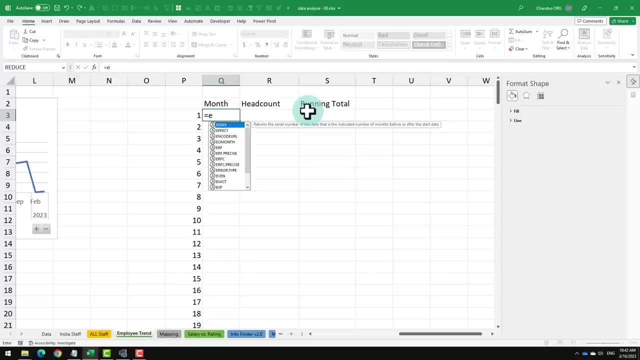 a sequence here. we could do this everything with one formula, but you know it's easier if we have two or three formulas like this. so sequence of 36 will generate all the numbers 1 through 36, and then we can have a E date function with the start date being date of 2020. fifth month, first day. 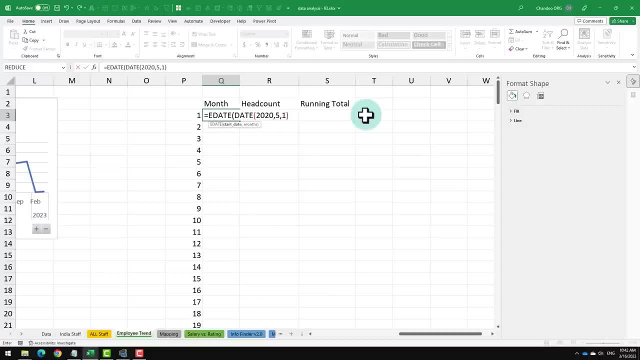 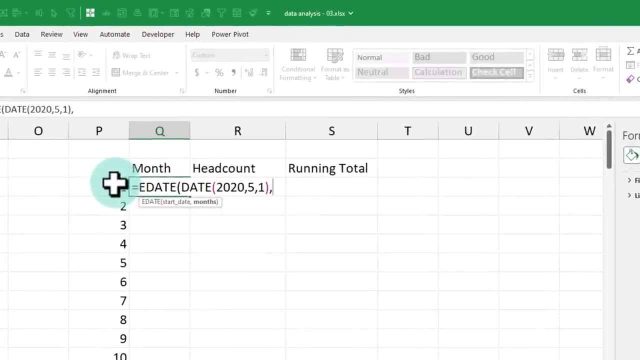 so that is May 2020, and then from that I want to go one month at a time for 36 months. so the 36 is here, so you can say p3 hash. that points to the entire range of sequence values, and I think we should start from 4 that way, because this is: 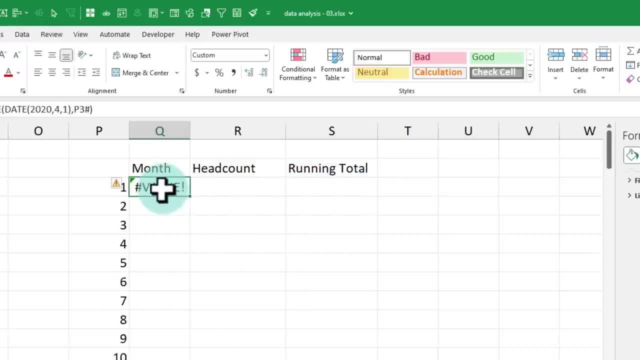 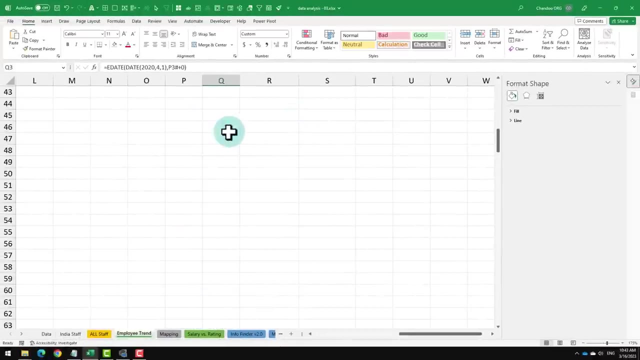 already 1, then it will add that 1 there and it will come up. doesn't really like that, probably because E date was not built for doing spill ranges. but once I add a plus 0 to it and fake it, it kind of works. so we will get all the dates up to. 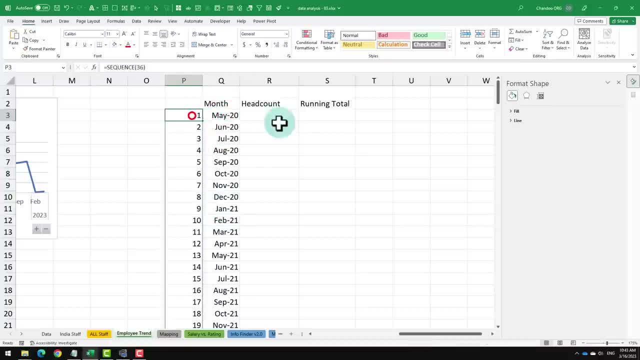 April 2023 here. this is a dynamic formula, so what it means is, if I date my data changes, I can come back here and, for example, change this to 48, and I would have all the dates up to 2024 here as well. let's just undo. 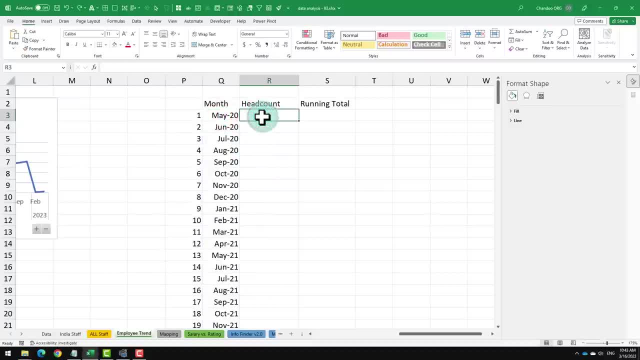 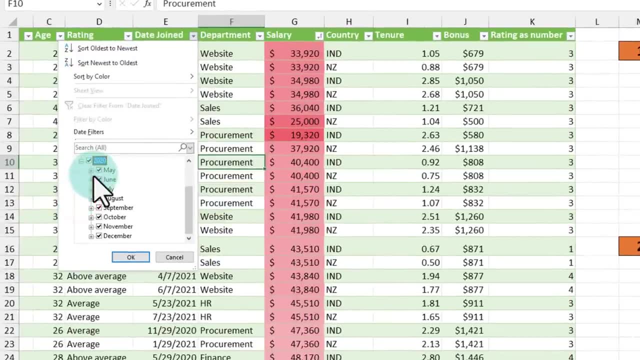 that for now and then for each month. what is our head count? so let's go back to the all staff and see what the problem would be, because employees would join on a specific date. so within May, we hired one on 7th of May, 11th of May, 29th. 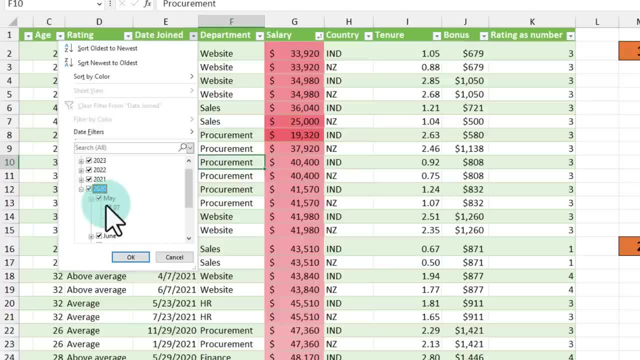 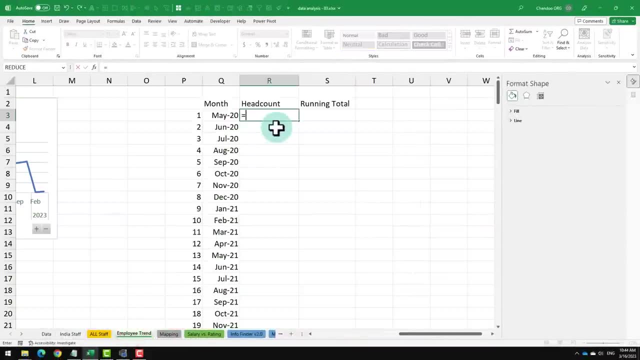 of May. so I would like to- irrespective of when they are hired, I want to count them all in the month of May. so to do this we could use the countifs function, but we'll have to get a little bit creative around it. so let's go back to the 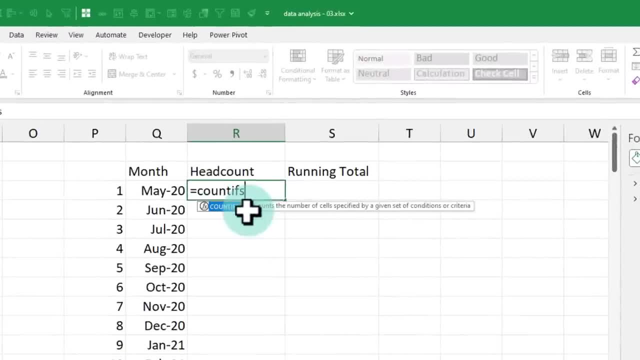 round it so we can say: countifs staff date joined. now the date join has to be on or after 1st of May 2020. so we could say greater than or equal to ampersand that number, because that is a number, and greater than or equal to. 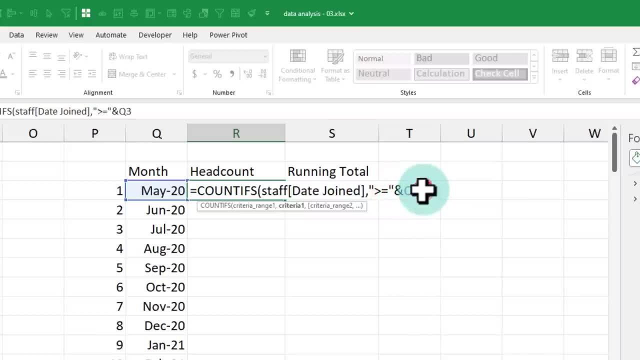 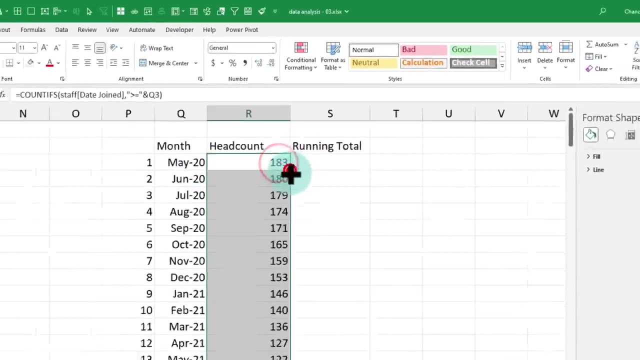 is an operator. we have to use ampersand here, and then it's not enough if they have joined on or after May. we'll also need to make sure that they are just in the month of May. let's just see what happens. if I do that alone, then I'll get kind of like a reverse running total. but this: 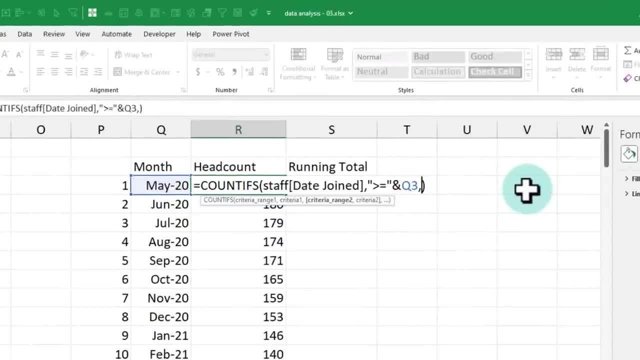 is not the correct one. so what we want is they have joined in on or after me, but they didn't join any time after they. it has to be before the end of May. so one more condition: this time staff date joined is before the end of, so less than or equal to and, and then, whatever this date is, we need to go to the. 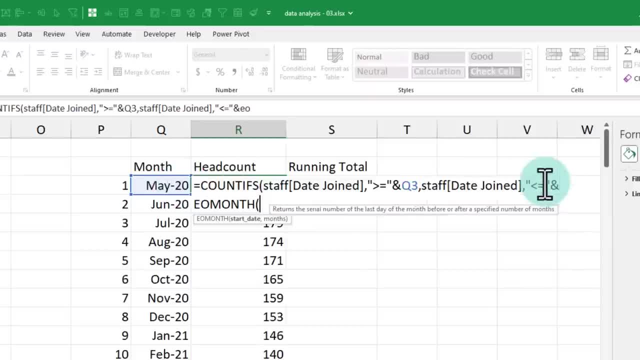 end of the month. so this is where we could use the evo month function of that within the same month. so we'll say zero and close the brackets. so what evo month does is it will take you to the end of the month of 2020, May, which would be 31st of May 2020.. so three people. 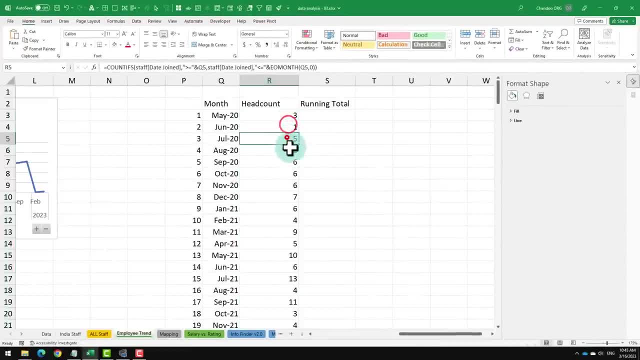 joined in May, one person in June, five in this month. like that. if we didn't hire anybody in a month, that will be simply zero. so now that all the individual numbers are there, if I add all of these up we'll get 183, as you can see in the status bar here. so the running total would be just. 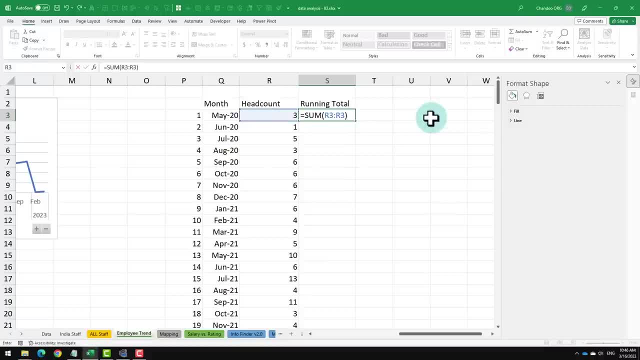 sum of r3 to r3. but we'll make the first part of the sum absolute, so it will be dollar r, dollar 3. the last part is relative and then when you fill this guy down, it will be a running total. so now that all the information is here, I can just select my month column and then select the running total. 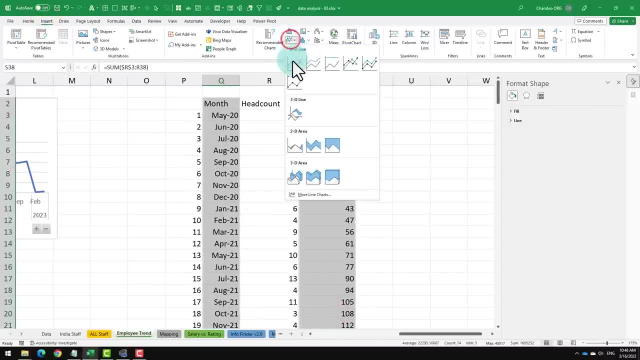 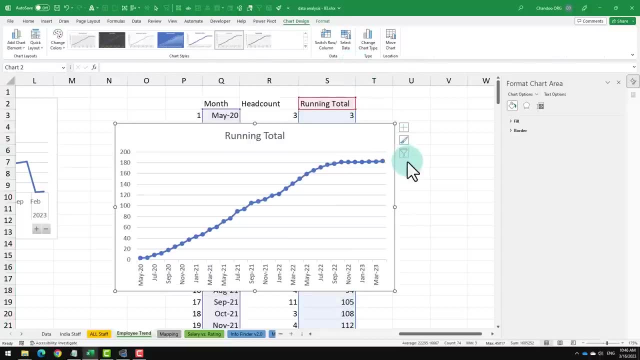 column and go to insert line chart and add a line chart. that kind of shows us how our company is growing so you could see what is happening. over a period of time we had some rapid growth but we seem to have stabilizer now at about 183 people or 180 people. that's because, while people do love, 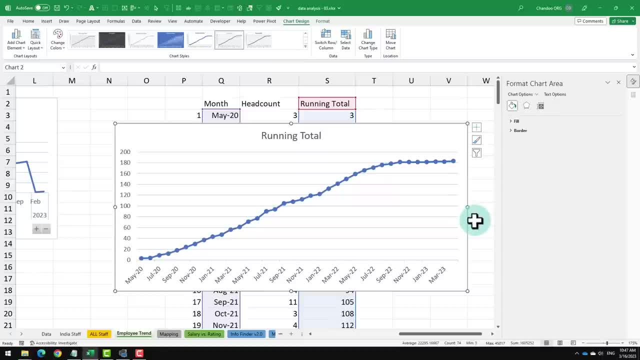 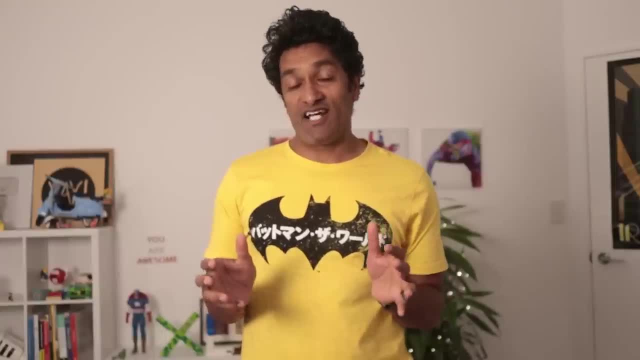 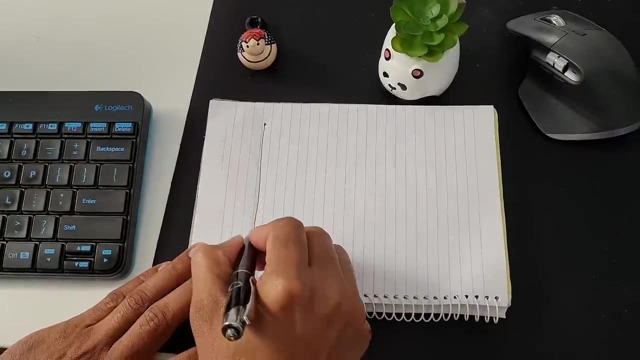 to eat chocolates. we have also gotten a lot efficient with chocolate production, so we didn't need to hire new people constantly. all right time for the grand finale: making a report card between New Zealand and India without data. so maybe we can make a report like this where: 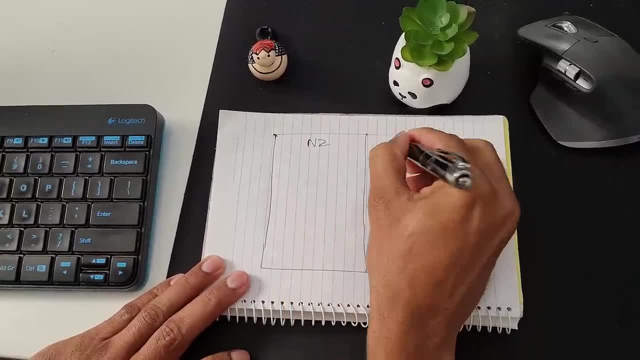 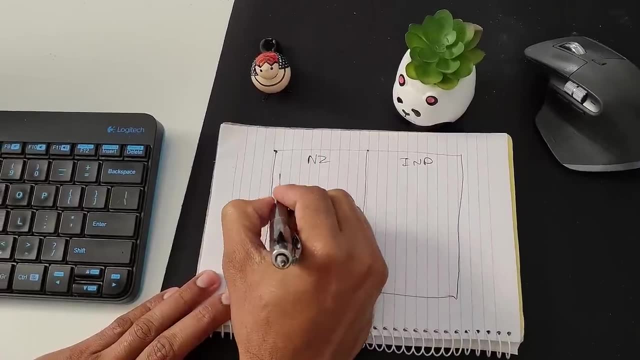 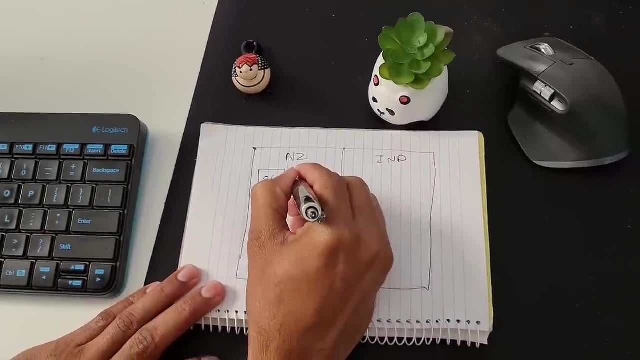 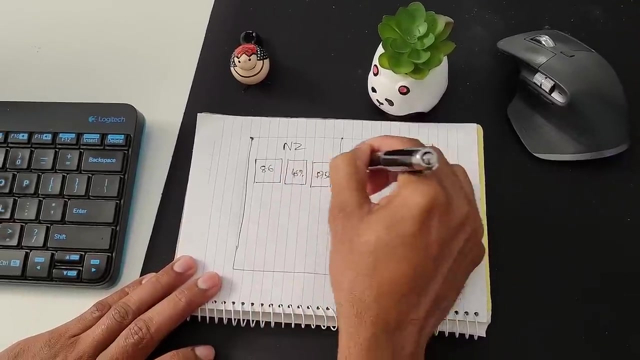 it kind of has two parts- NZ, India, on both sides, and here we would like to show similar information. so maybe I want to show the head count, for example 86, and then female ratio, let's just say 48 percent, and then average salary: 75k, and then similar kind of information here, and then I want to show 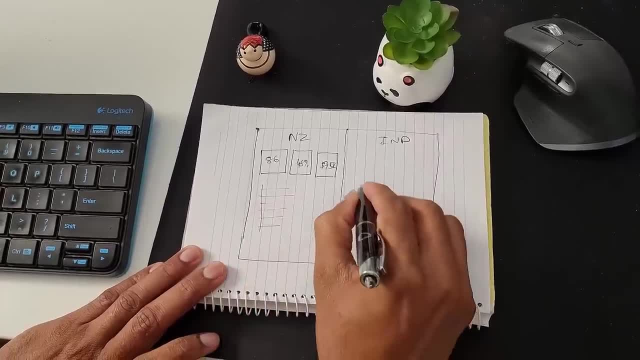 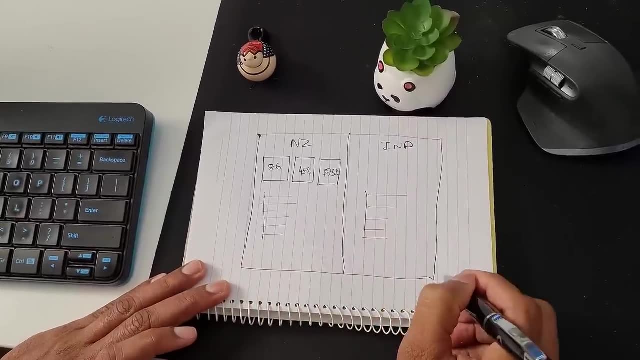 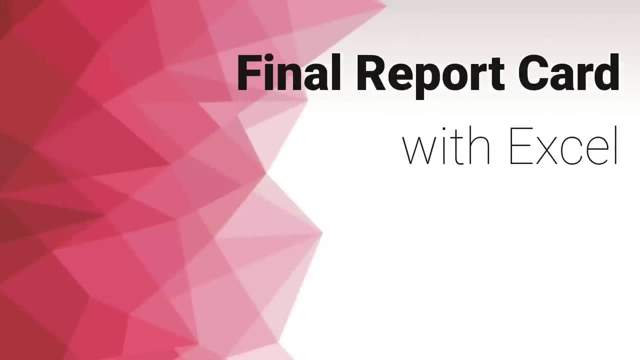 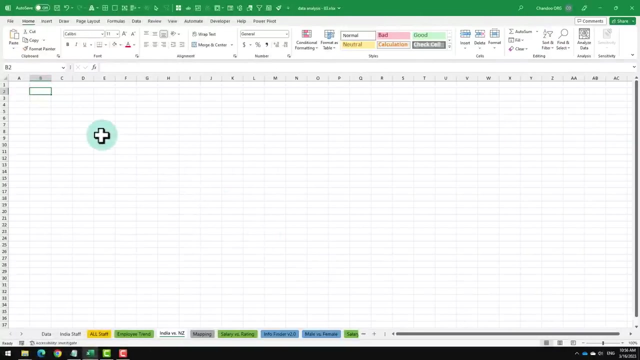 department wise head counts as a graph on both sides, and that's it. but if you want, you could also add other stuff here, so let's go ahead and make this in Excel. in a new sheet I'm gonna make a layout for our India versus New Zealand scorecard. so we need three sets of information. one is head count, one is female. 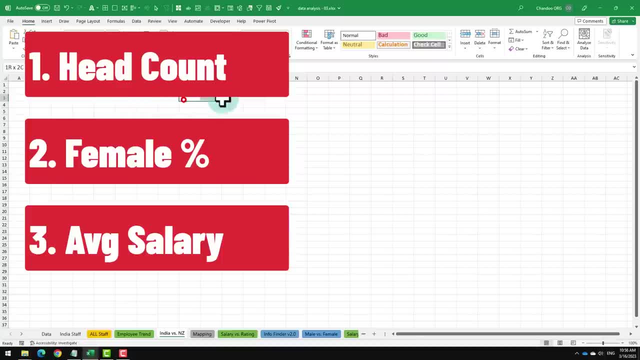 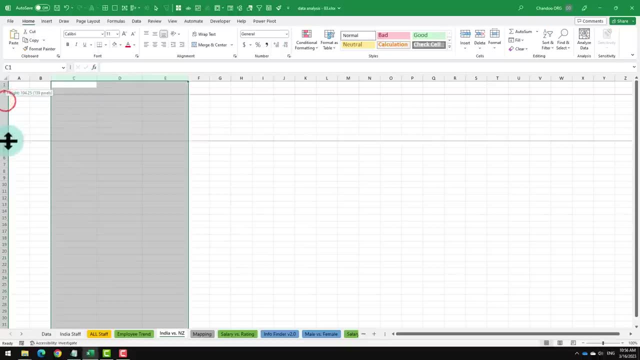 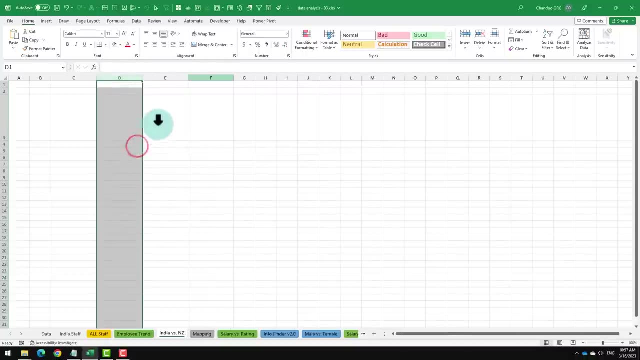 percentage and one average salary, and then the same thing needs to be repeated here. so I'm going to take these three cells and then make them wide and tall, so each cell will contain one set of information and, if you want, add an extra column in the middle and make this column narrow. this way the boxes will not be touching each. 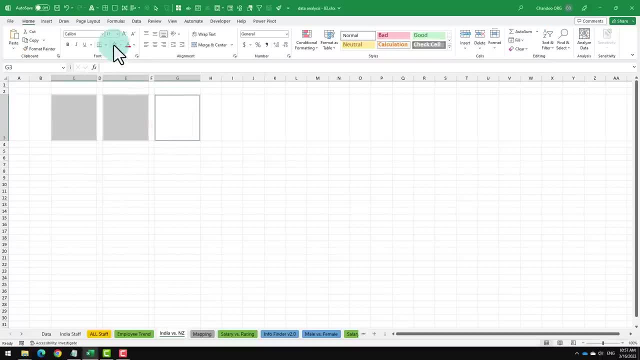 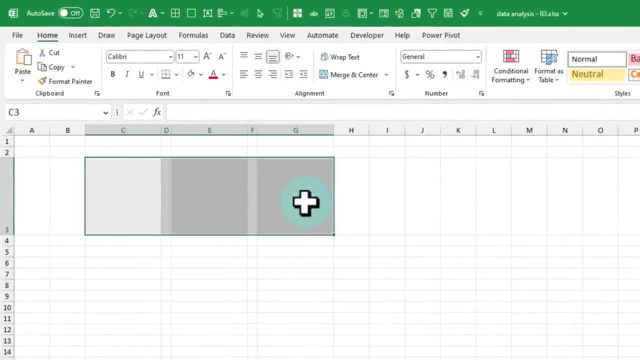 other, and then we can fill up some color here. let's just start with that color, but later on we can change this. so we want a similar structure on the other side as well. but first let's make this for one side and then we can copy paste. 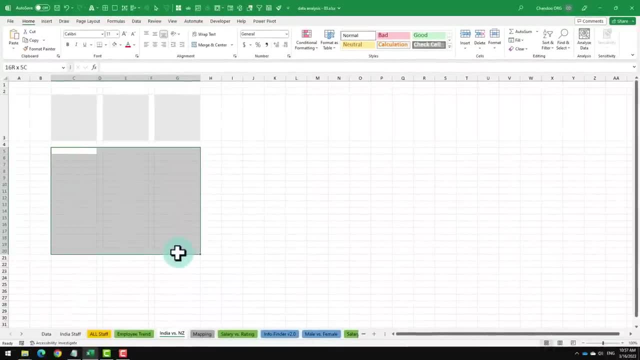 it on to the other side next up here. we would like to make a place for our department spread, so for each of the departments, how many people are there? that information would go here. now that one side is done, I'm going to copy this ctrl C and then go here and ctrl V. it would only paste them. 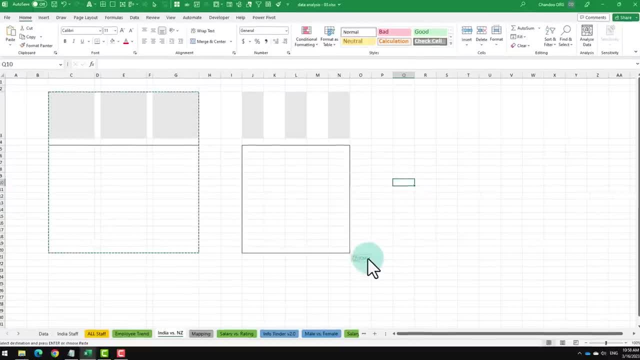 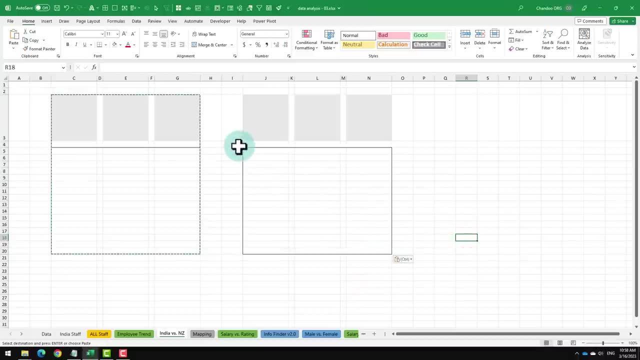 on one side and then go here and ctrl V. it would only paste them on the other side thing, but it won't adjust the widths. but after you paste, use this little box here and then use this option to get the exact column width, same as on the other side. so this is my New Zealand side. 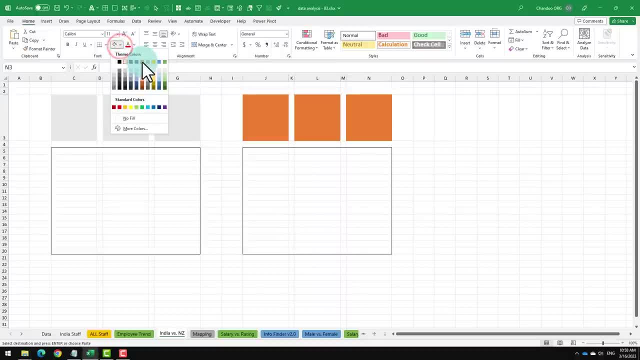 and on the India side we are going to change the colors to that, and for the New Zealand let's go with the blue color that we had originally. so that will be New Zealand numbers here, India numbers there, and then the department spread graph goes here. so what we want here is how many people are. 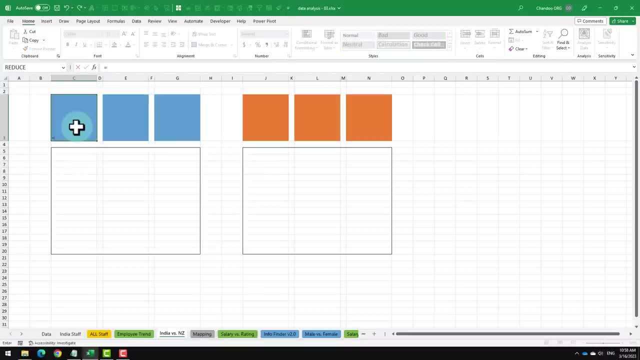 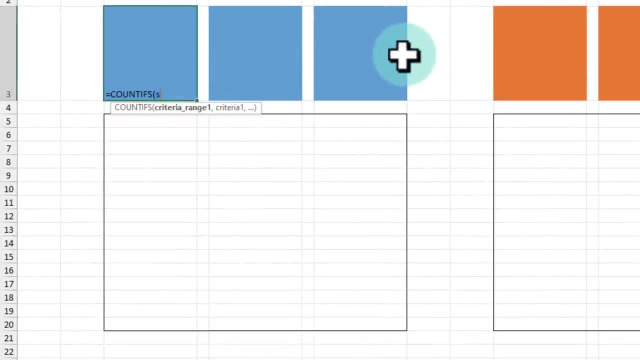 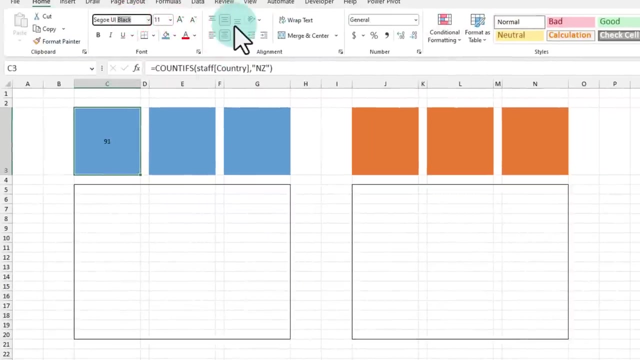 within New Zealand and this is can be done with a countifs function, so we could say countifs and fill up the formula. so staff country is nz 91 people, and just put it in the middle and let's make this nice and big like that. and the female ratio is: we need to calculate how many female employees are there. 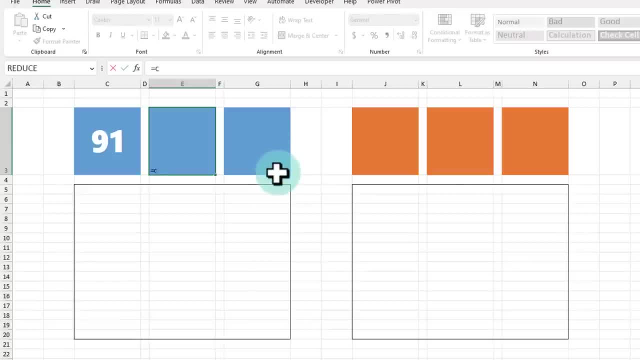 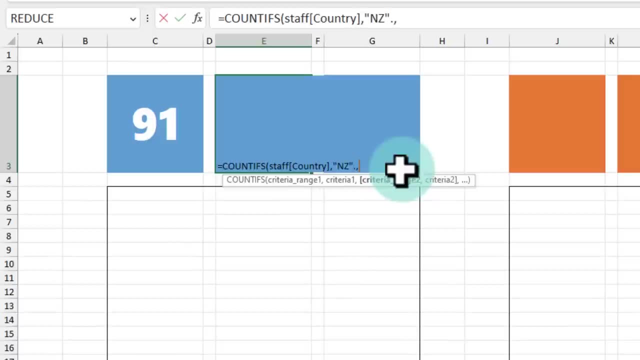 within New Zealand and then divide that with 91. so countifs staff country is nz 91 people and just put it in the middle and let's make this: countifs staff country is nz 91. staff gender is female and then divide that with the 91 that we already have here. that will come up with the percentage. 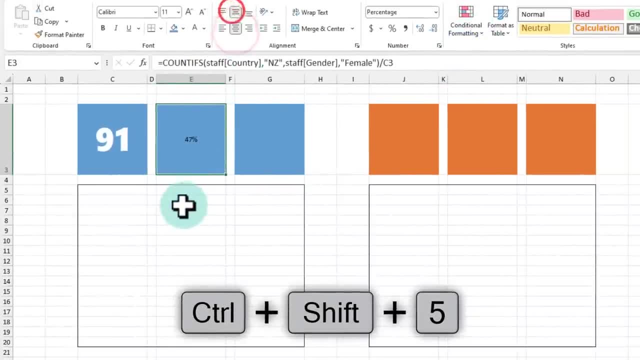 control shift 5, we'll get the percentage formatting and that number goes there. now I want this to look exactly like that, so I'll select this one, click on the format painter and paste that there and then apply the control shift 5, maybe tone that down a. 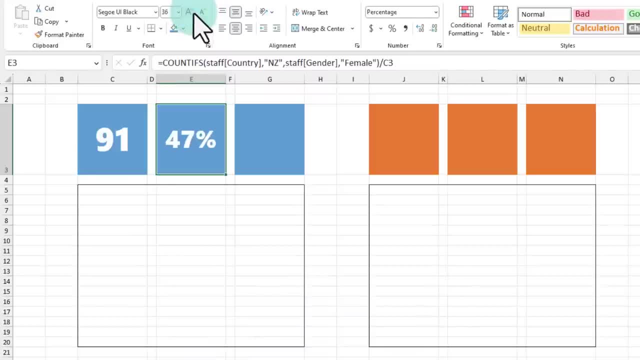 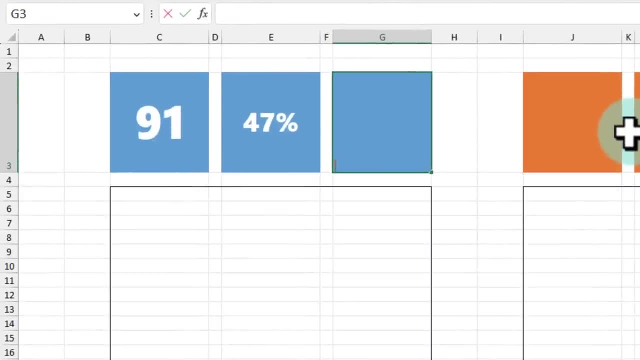 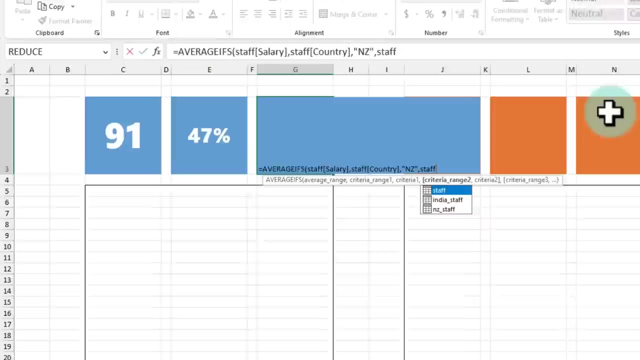 little bit: 36 points, let's go with 28, and then for the salary we could use the sum ifs- sorry, we could use the average ifs function and then say: staff salary, staff country is nz staff. I think that's it. we don't need to do any more conditions- and we'll get the average salary in New Zealand here. 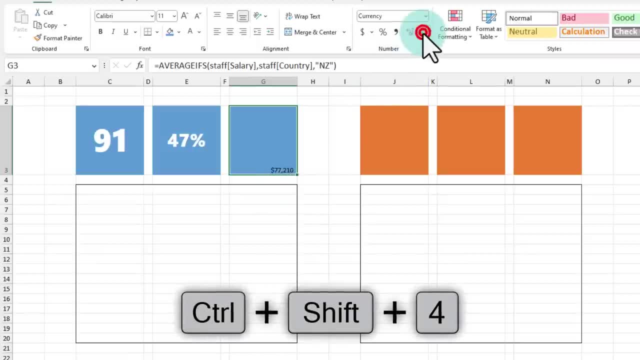 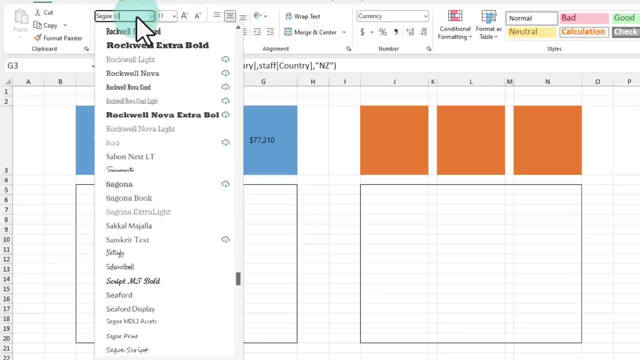 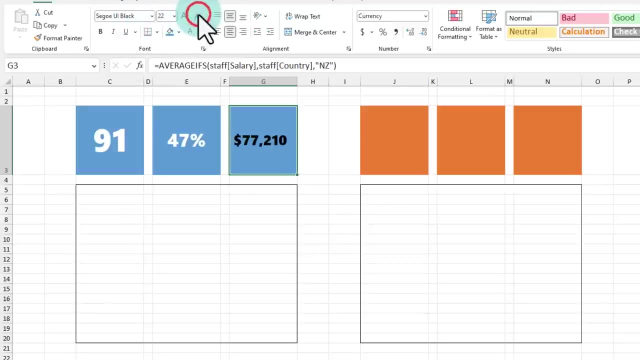 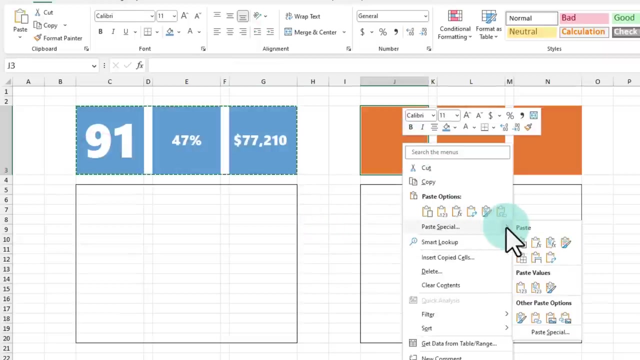 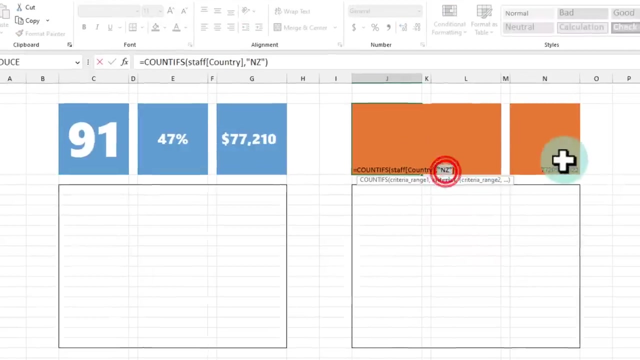 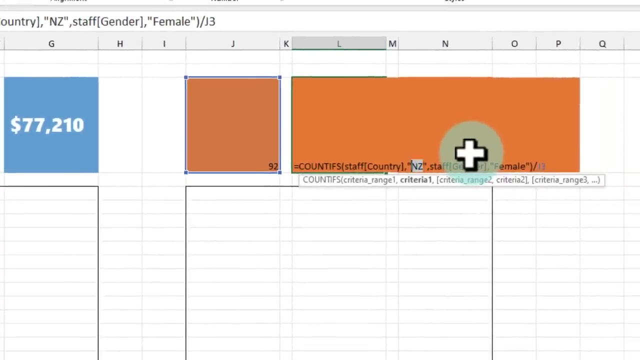 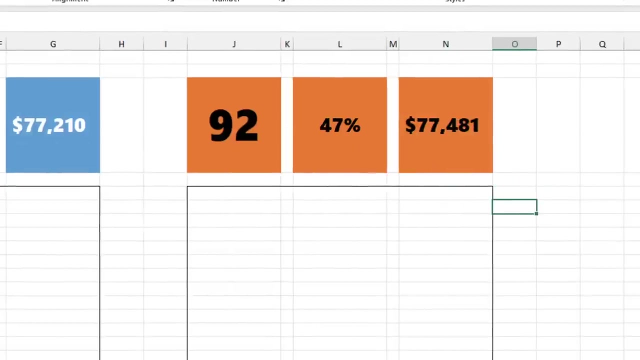 again control shift 4, we'll apply the currency formatting and we'll put this. so let's make. I think that looks good. we'll just copy these paste here as formulas, so only the formula portion comes here, and then change the words from nz to ind. all right, they're almost neck to neck here, but that's because we do have equal amount of staff. 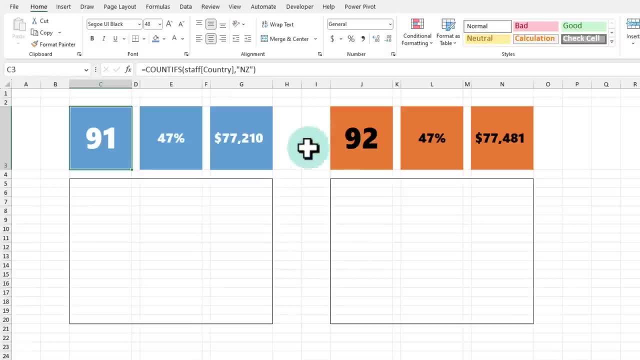 in both countries and they are kind of paid on par. now let's see what is the department level distribution looking like. for this we could use some pivot tables, so it might not be a good idea to put the pivot tables directly here, because that will look clutter. so you may want to just 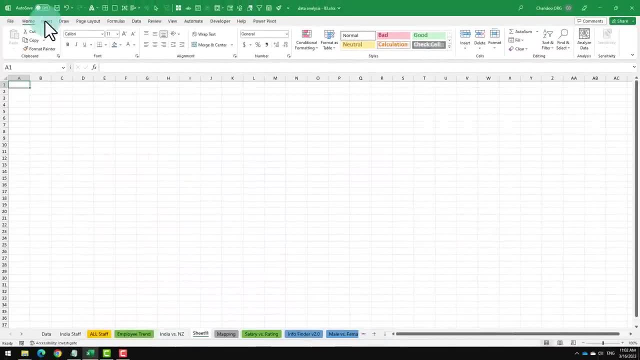 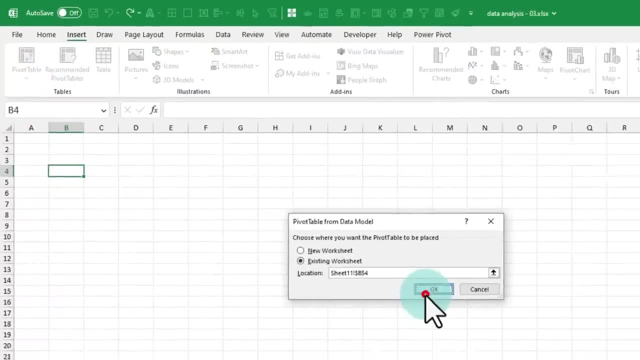 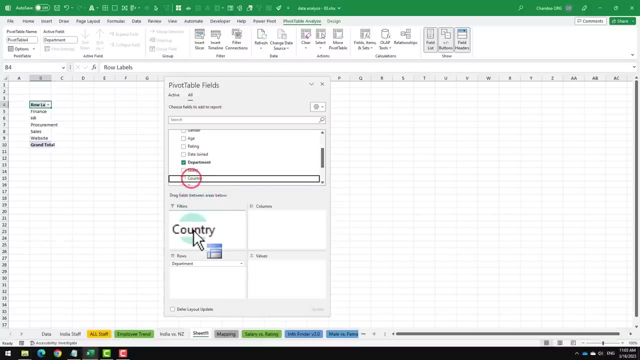 set up the pivot tables in the same way. so let's go ahead and do that. so let's go ahead and do this in a different page and then copy paste the results here. so here, insert a pivot table from the date model, put department into row, label area and country into report filter. 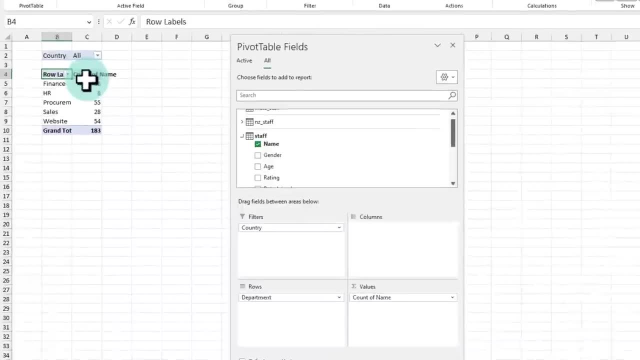 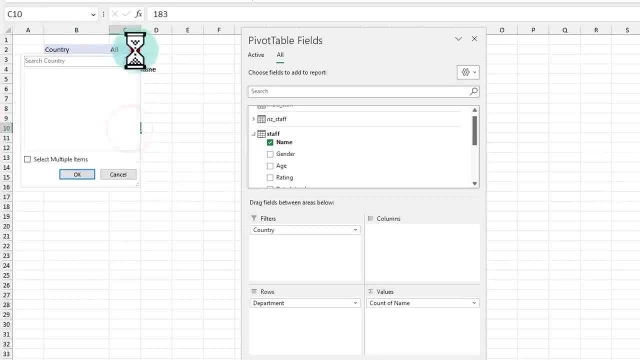 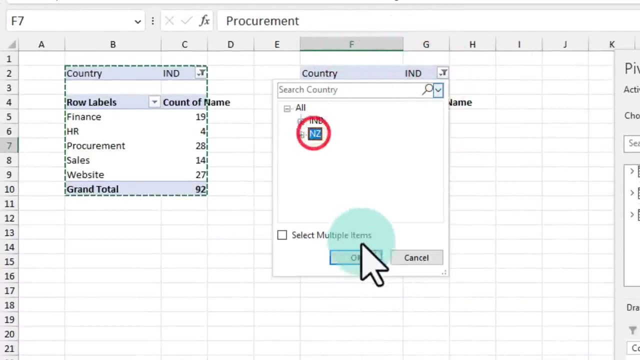 and name as the value, so that we will have all the departments. now this shows everybody. so if I filter this down to just irs and d, I'll have my india distribution of 92 people. I'm going to ctrl c this pivot, paste it here and then change this one to new zealand. so we have two pivots: one for india, one for new zealand. 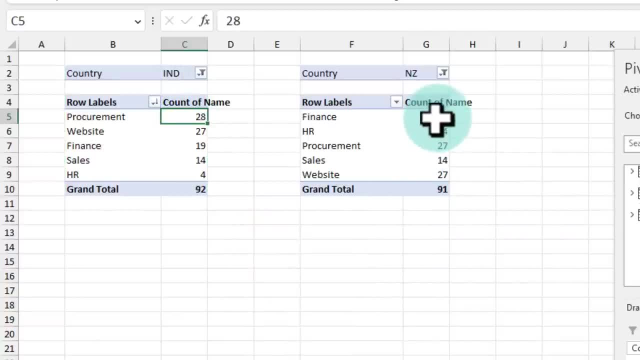 let's just sort this in the descending order of the employee count. so, for example, india has higher number of people in procurement, whereas new zealand has higher number of people in procurement. so let's just sort this in the descending order of the employee count. so, for example, india has higher number of people in procurement. so let's just sort this in the descending order of the employee count. 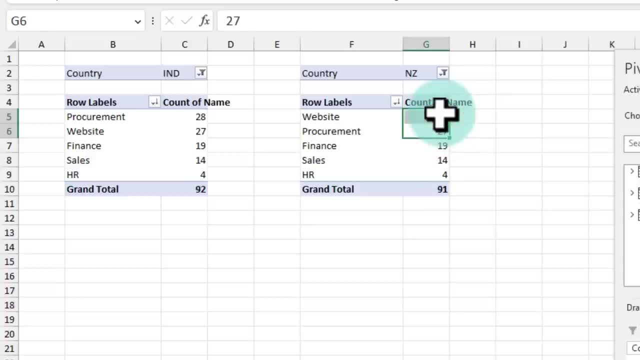 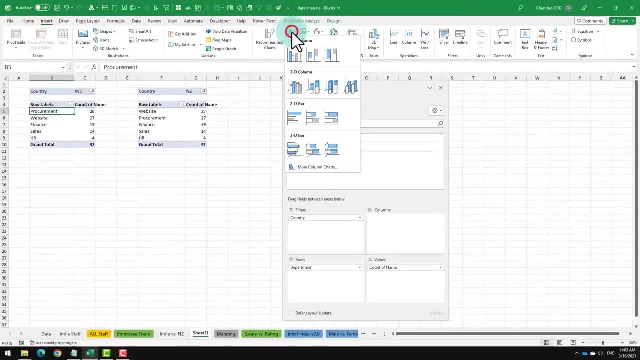 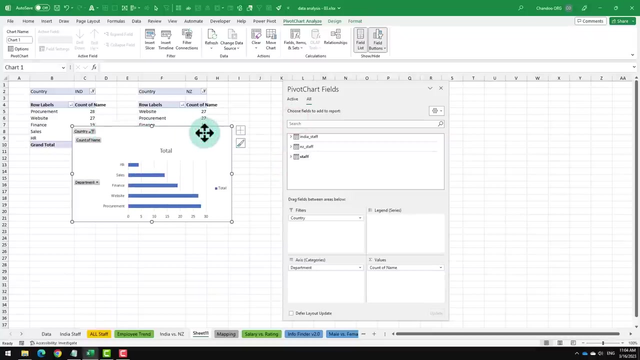 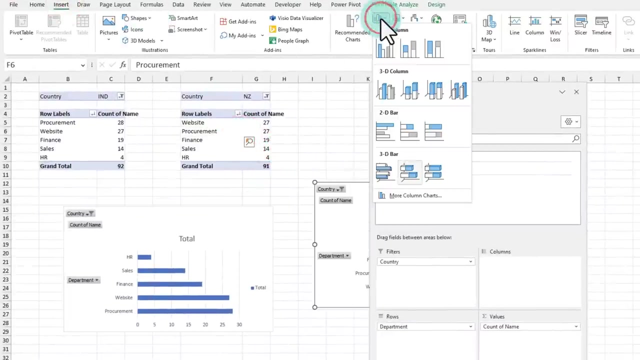 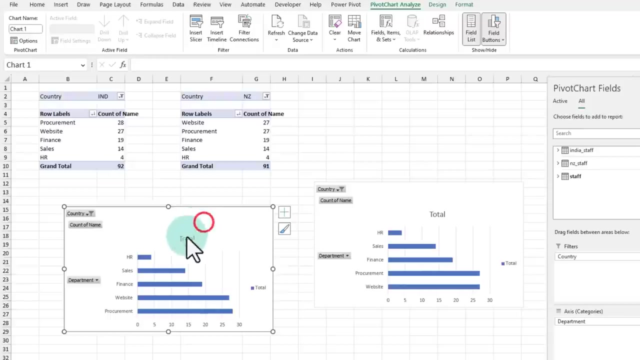 in website. well, they both are same, but that's how that looks. once that is there, then you can just select this and insert this as a bar chart. we'll make a bar chart for this one as well, and then the india bar chart. I'm just going to change the color, because they both look blue. 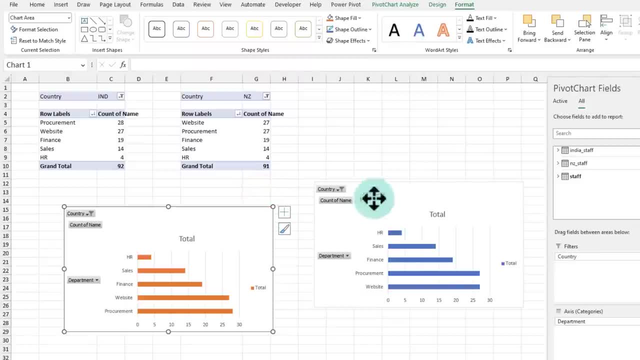 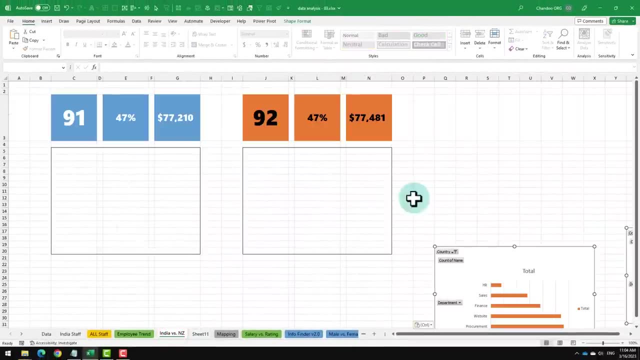 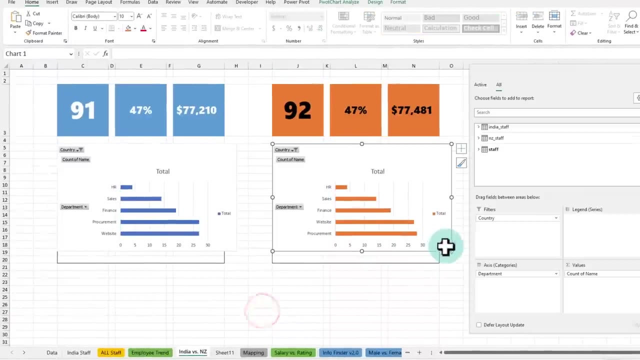 it kind of gets confusing. so india is orange and new zealand is blue. I'm just going to select these ctrl x them and paste them here. that looks good, but it kind of looks like a blue bar chart, so I'm just going to change the color. 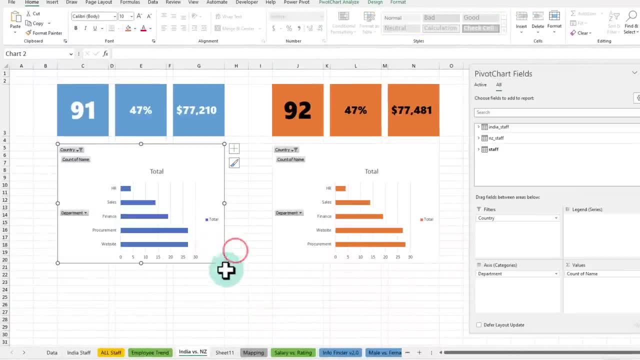 and then the india bar chart. I'm just going to change the color because they both look blue. it kind of gets confusing. so india is orange and new zealand is blue. I'm just going to select these ctrl x them and paste them here. and then the india bar chart. I'm just going to change the color because they both look blue. it kind of gets confusing. so india is orange and new zealand is blue. I'm just going to select these ctrl x them and paste them here. 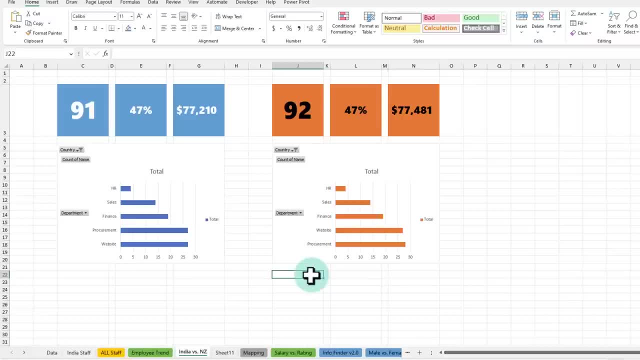 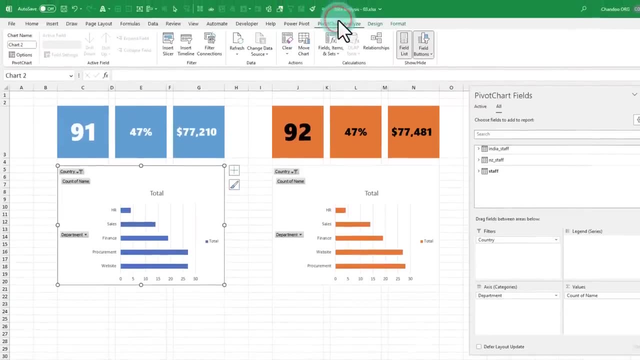 that looks good, but it kind of looks a little bit ugly with all these buttons and superfluous words. so let's clean this up, select this one and then go to pivot chart, analyze ribbon and uncheck the field buttons. so those buttons are gone. likewise, I'm going to take out the legend. there is only one series value, so we don't need the legend. 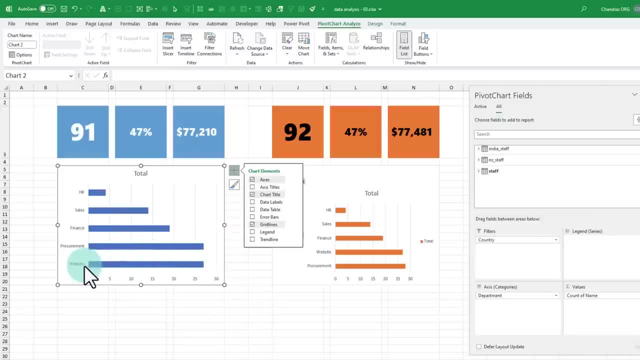 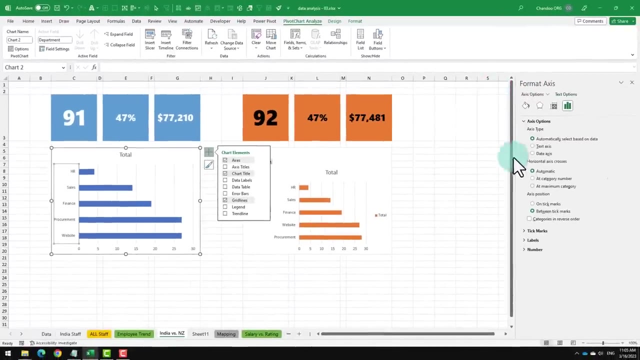 and then if you look at the ordering here, the highest department is at the bottom, lowest department is at the top. that kind of looks incorrect. so I'm going to select these departments, press ctrl 1 to format them and from the format access options, use the categories and reverse order option to. 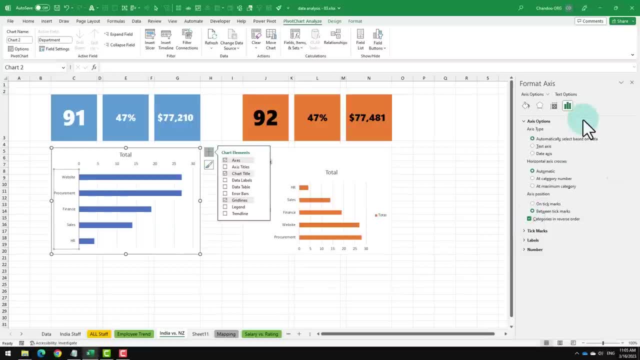 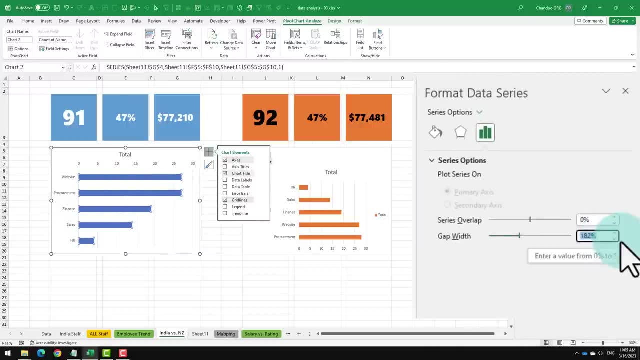 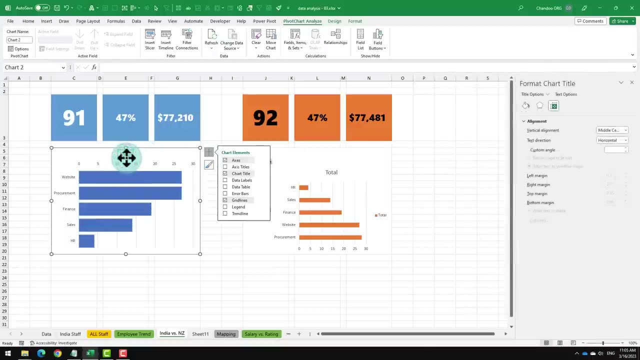 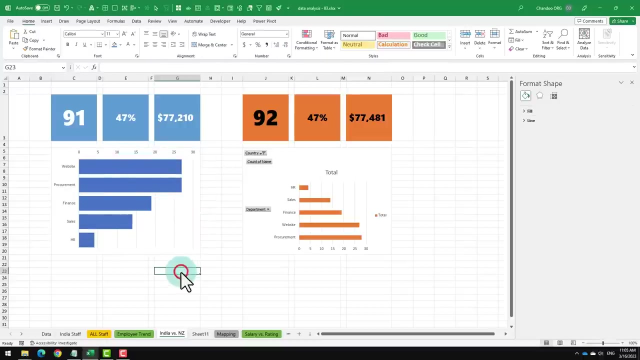 flip the order while we are here. let's go to the bars themselves, and then the gap width is too high, so I'm going to make this 25, so that the bars are nice and thick. and then the word total is not required, so I'm going to take that out and place it like that: this: 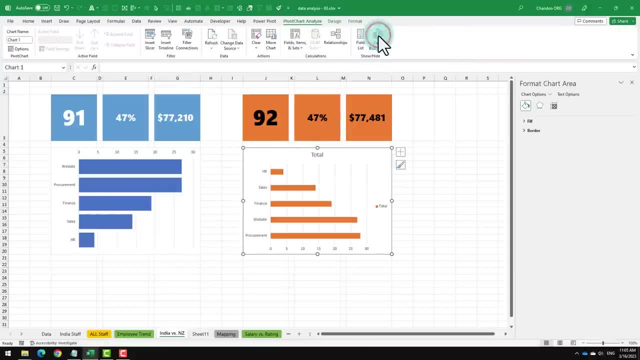 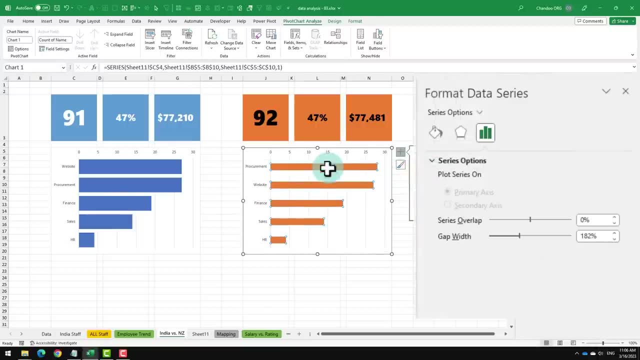 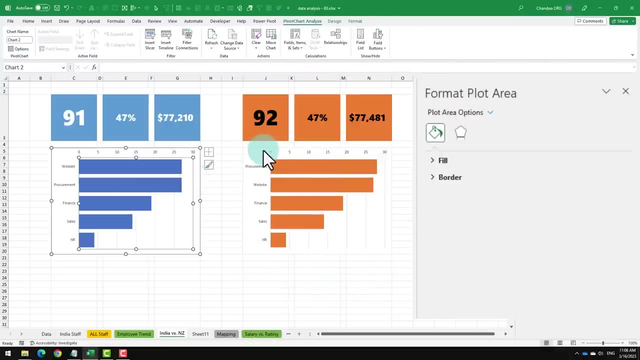 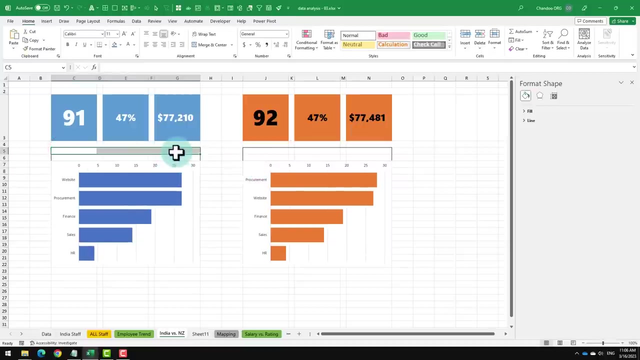 looks good. let's do the same thing for this one as well, and then let's just move them down a little bit and then let's add few more rows in the middle for our title. so here I would like to put a title. I'm going to select that entire. 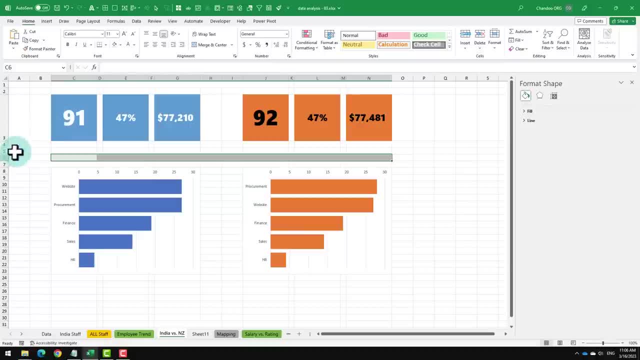 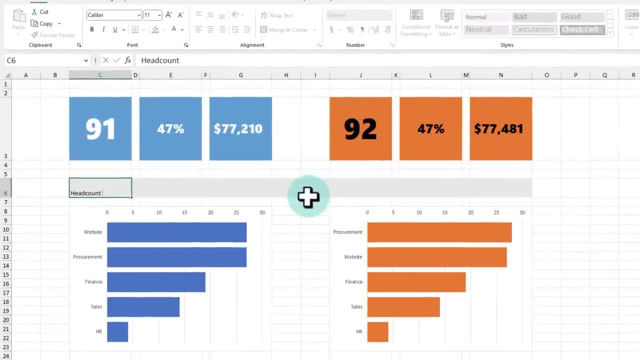 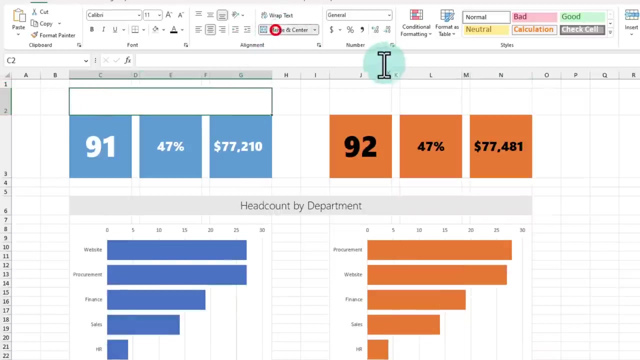 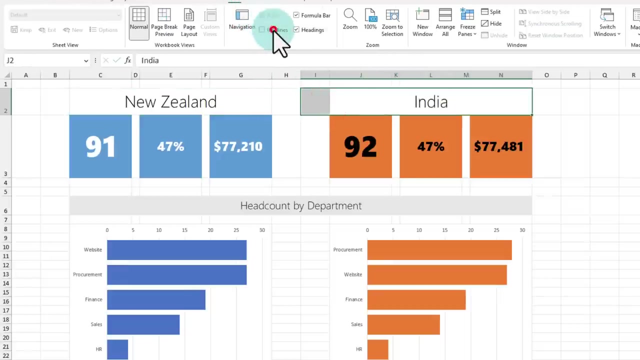 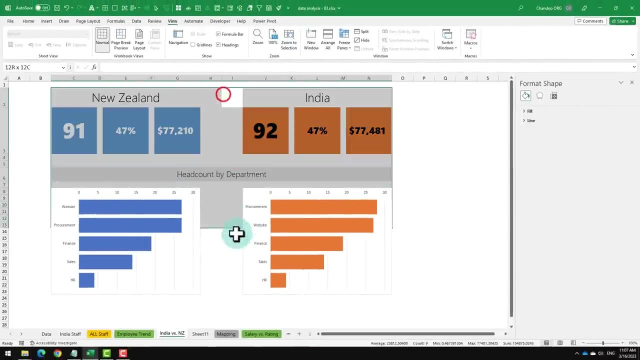 thing and then, all right, that looks good. let's just tidy it up by putting a word here that says New Zealand and India, and we'll go to the view ribbon, take out the grid lines so that we have our scorecard ready. if you want, you can add a vertical line in the middle. you can. 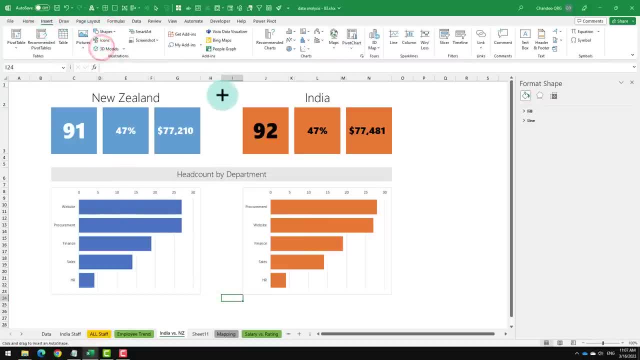 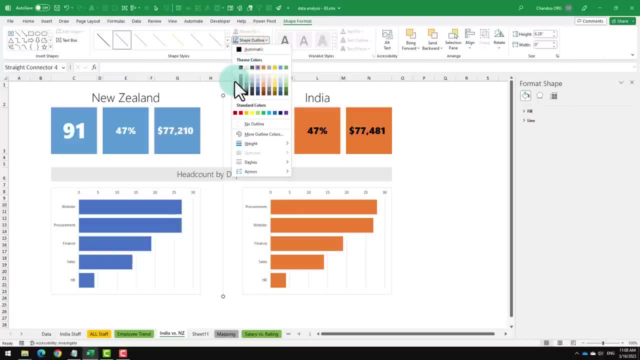 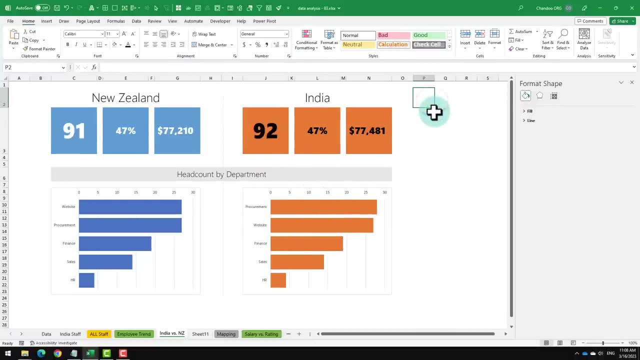 just go to the insert shape and then select the line and add a line that cuts through the entire thing like that, and just make it dull and dotted. so there is our kind of simple but also elegant india versus new zealand comparison. like i said, there is nothing interesting going on here, but it does prove that through this process we discover. 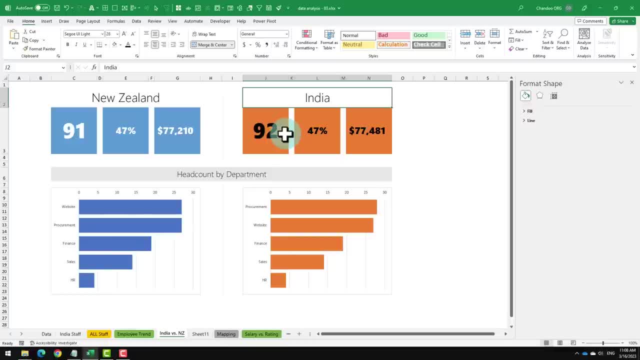 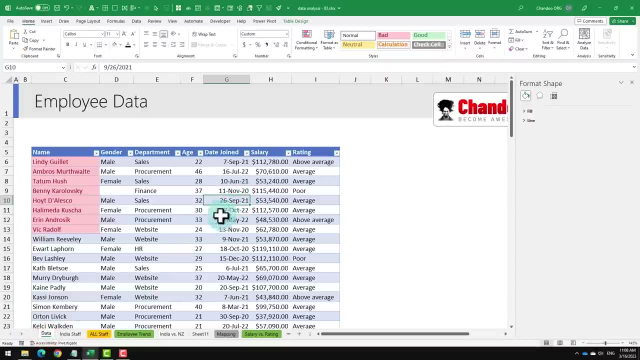 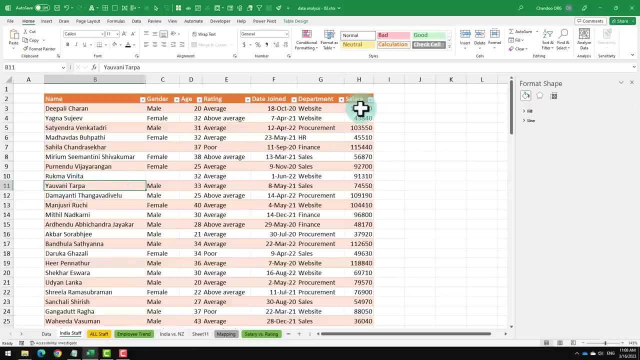 more about the data and also make it more presentable and elegant, and all of this is dynamic. so if your data changes- for example, either you have more people in new zealand or india and one of these tables change- all you have to do is update the data. so, for example, let's just take 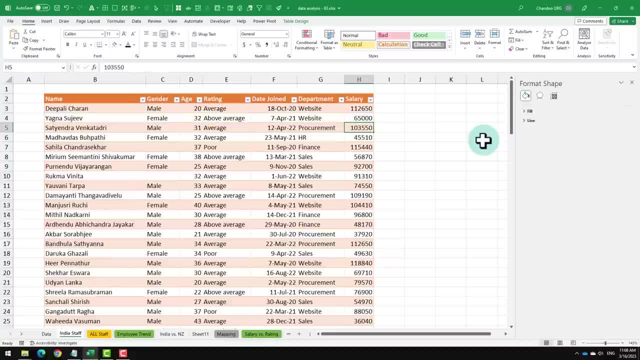 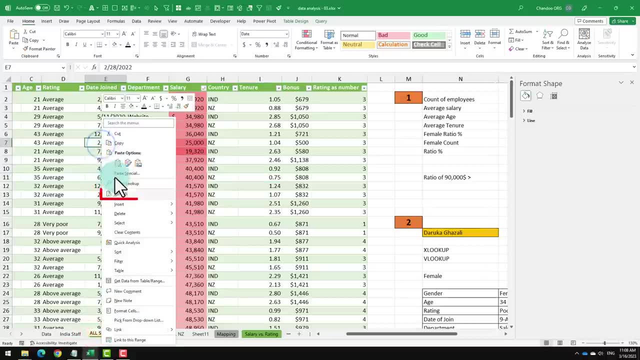 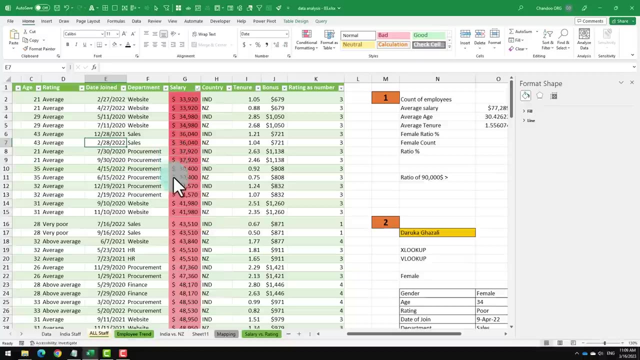 this person and then make their salary 65 000. so we changed one person's salary and i can come here, right click and then refresh. this is gonna refresh this table, which will update the person's salary here, and then we can go to our india versus new zealand page, go to data and refresh all in. 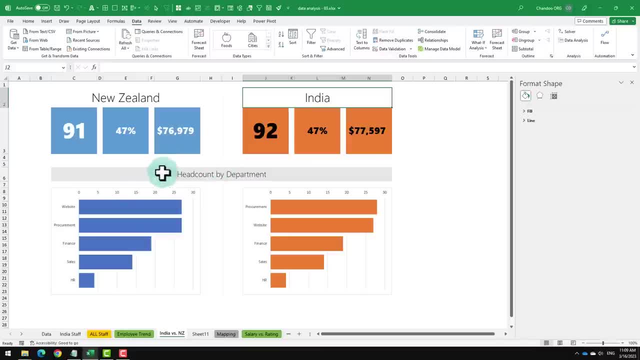 any of the pivot tables or any calculations. that will all be updated, of course, here, because the salary is just directly formula, it would have already been updated. but if there is any other changes to the department or something, that would have also been reflected. hey, i hope you enjoyed. 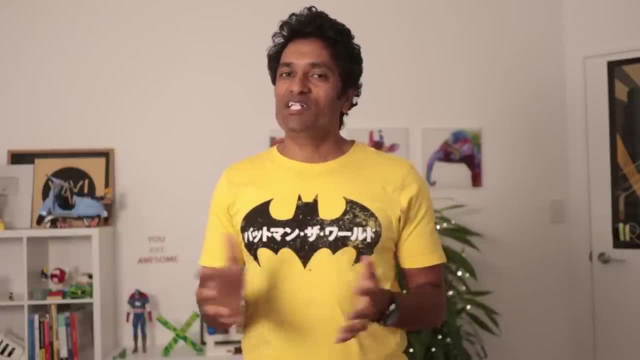 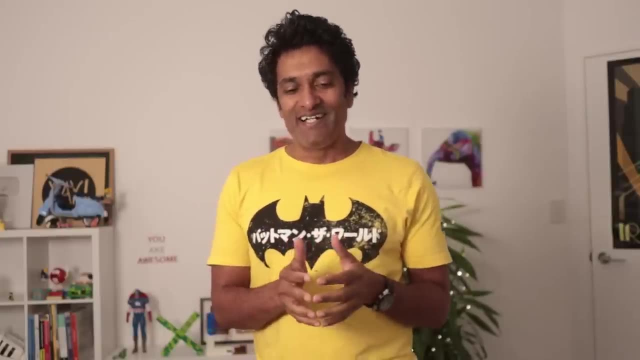 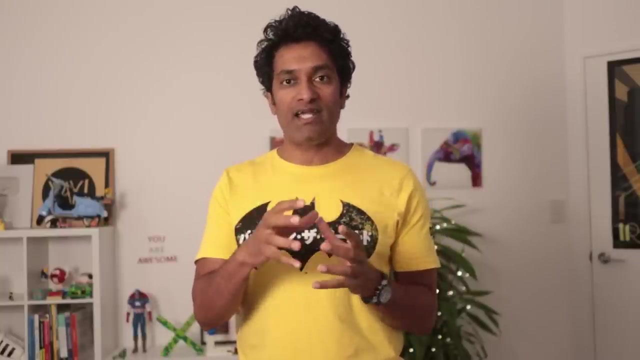 this video. if you do give it a like and share this video with some of your friends and colleagues so you can also learn, excel and excel in their work. thank you so much for taking time to watch this video and if you like these style of in-depth videos where i take a business data and go in. 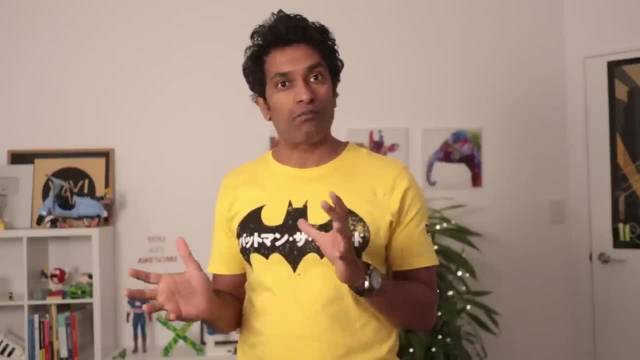 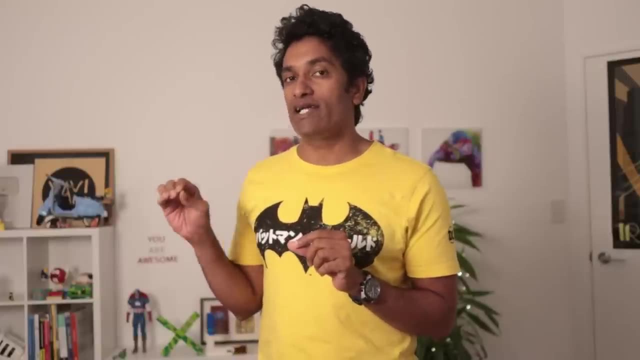 depth into solving various problems and showcasing how to present the data in elegant, beautiful manner. then do consider checking out some of my detailed courses. i have got two courses, one on excel and one on power bi, and the links for that are on the description below, and i hope you found this video. 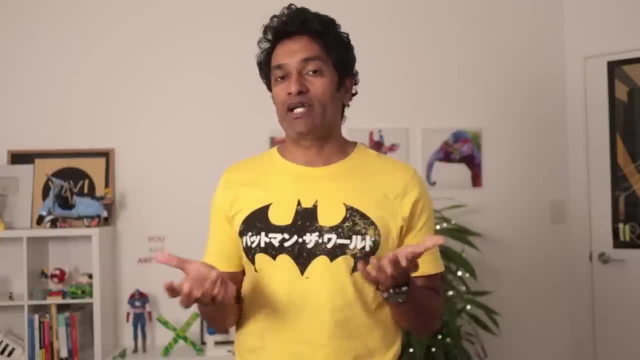 helpful. i would love to share it with you, and share it with you on another offer that you may want to take advantage of and I'll see you in my next video. Bye, available in the video description. check them out and sign up if interested, as 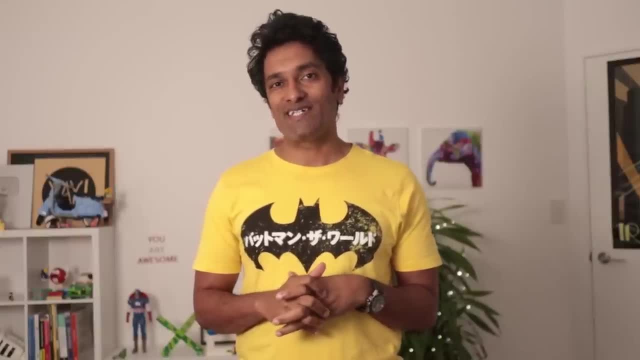 always. it is a pleasure talking to you and I'll catch you again somewhere else. bye.